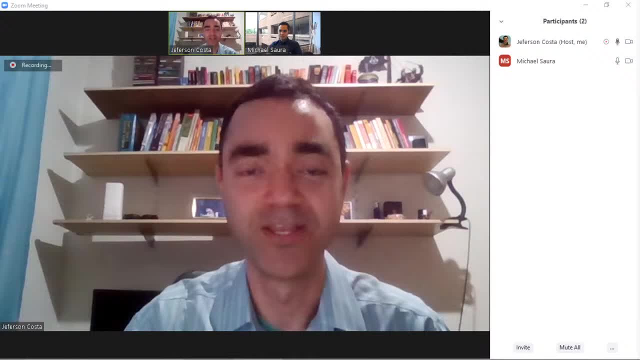 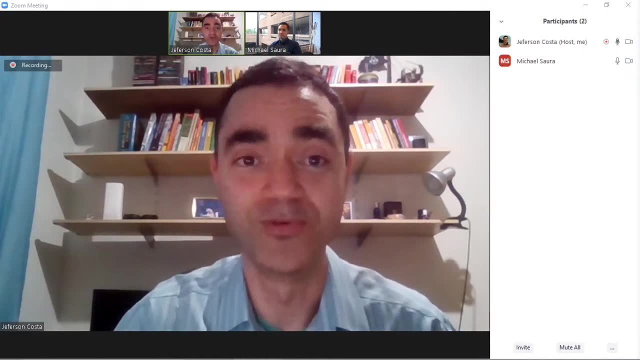 you really, really love this subject And I am very, very, very happy about that because it will be very nice this talk with you, So please present yourself. Michael Sauer is the representative of US and I will start with a brief presentation, And I will start with my 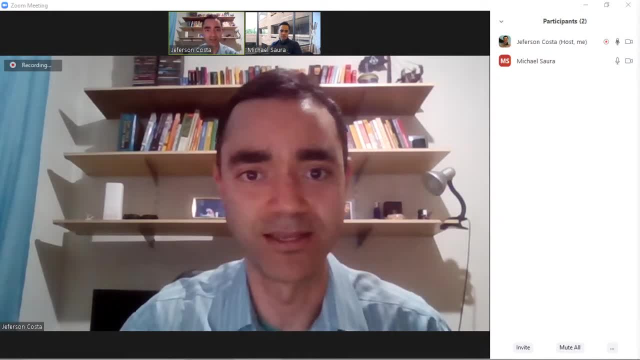 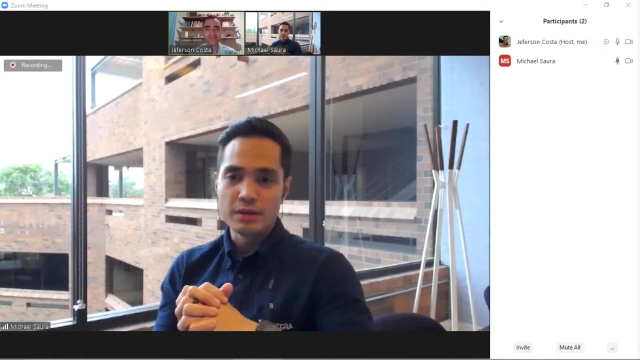 questionnaire that I have here to help me, And in this meantime, people talk to us where they are from. Awesome, So good morning everyone. First of all, Jeff, I'd like to thank you once again for inviting me in this live session. It's an honor to be here And, yeah, just to introduce myself, my name is Michael Sauer. 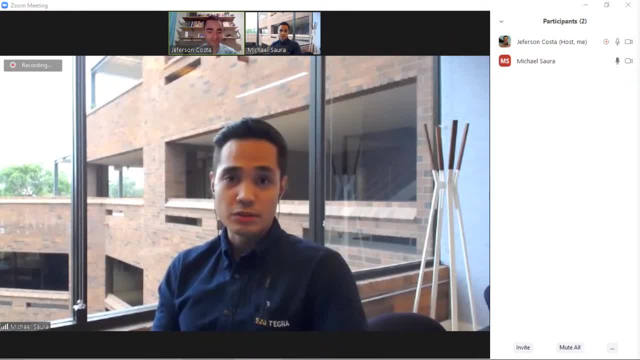 I am a process safety and risk consultant from Salt Circle Consulting, And I know that Jeff will be asking for my background later on, but my degree is in mechanical engineering. I've done that for about 15 years now. I've been a design engineer for four years And from there on I transitioned into process safety, And so, yeah, here I am. 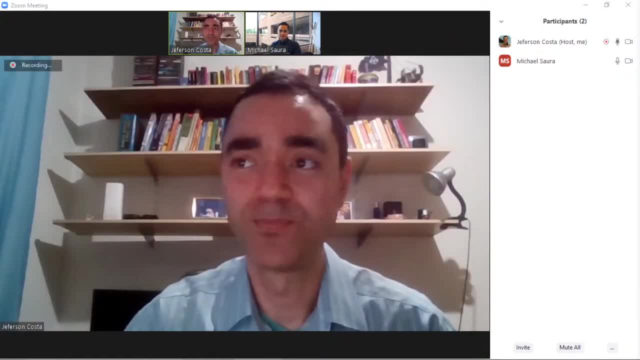 And I will start with the questions, But let me share with you guys some curiosities. I started this live, the in-process interview, with the objective with having chemical process engineers, at least one from each country, And Michael is representing the US. 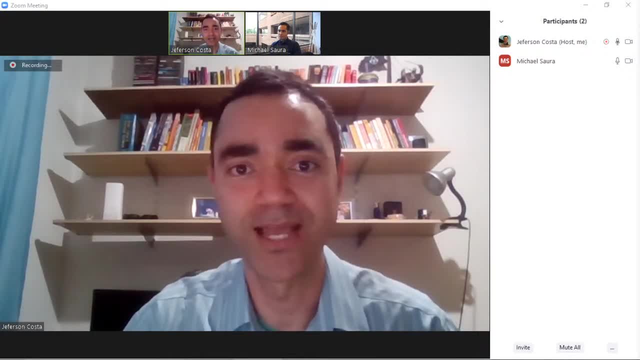 But I had a nice surprise that in fact he is from Philippines And one week before I did a presentation for the Philippines Institute And I was very surprised to find out that Michael is a professor of chemical engineering And people from there was very, very kind with me. So thank you, Philippines, for liking my work And thank you. Thank you a lot, Michael, for this good surprise, for sure. 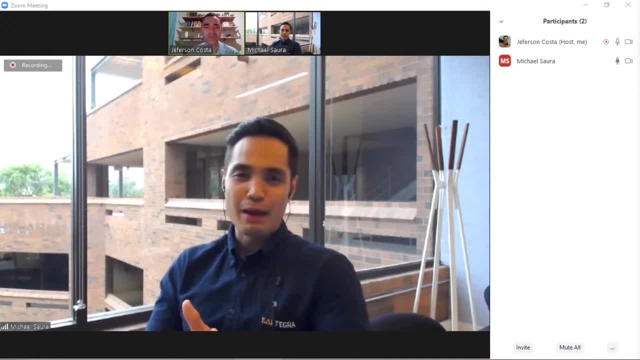 Oh yeah, So no, no problem. Like I said, once we get to the background, my background. I was going to say that, but it's interesting that you already mentioned it, So thank you. Some spoilers sometimes happen during live sessions. 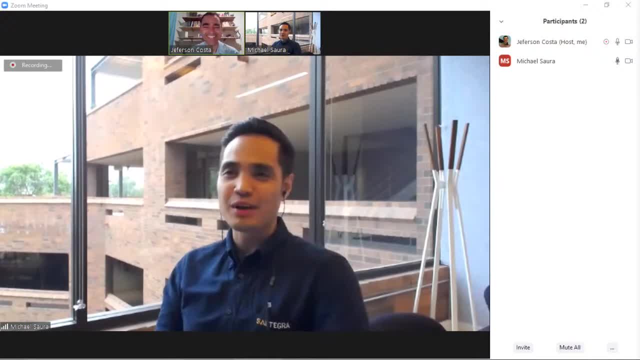 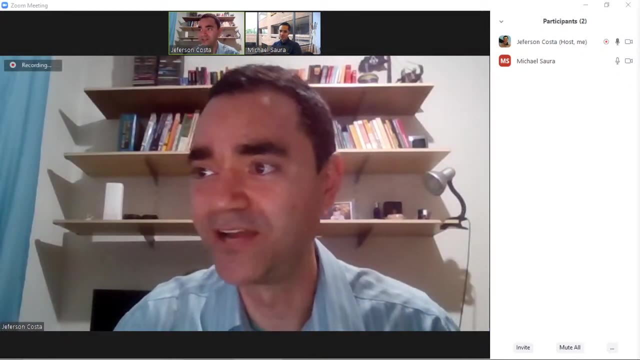 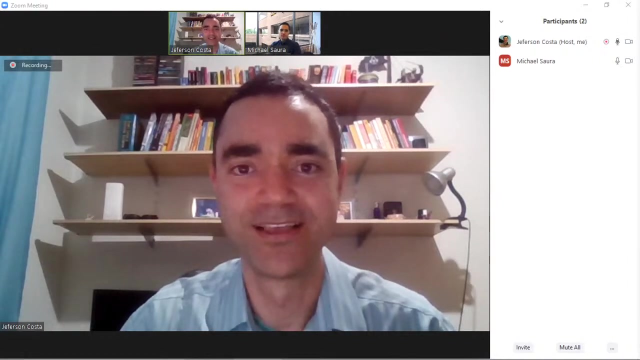 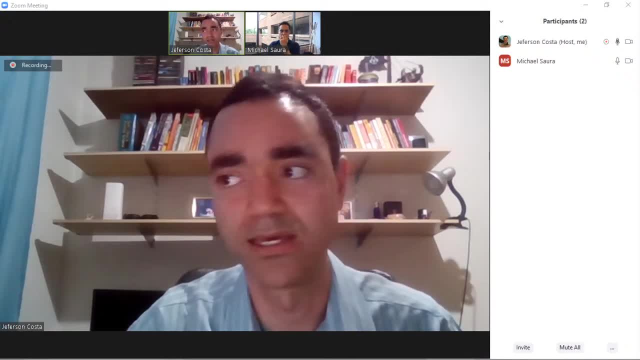 Okay, My first question is: how did you get your first job And how were you towards the transition between your? Okay, My first question is: how did you get your first job And how were you towards the transition between your? more information about the hasop and we, if we have time, proceed with lopa and see if you have time. 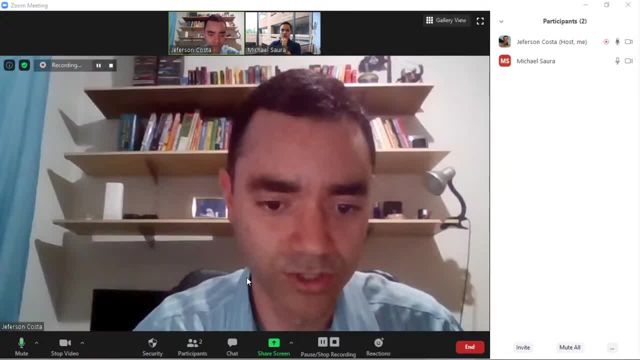 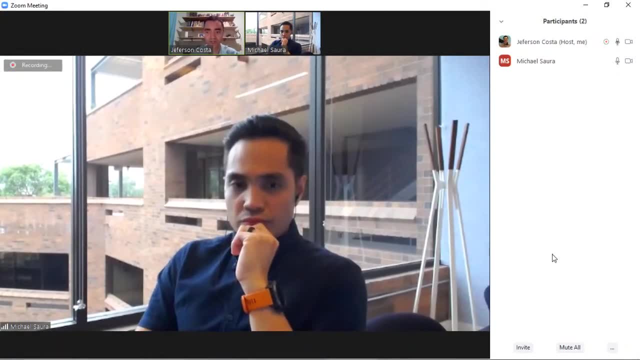 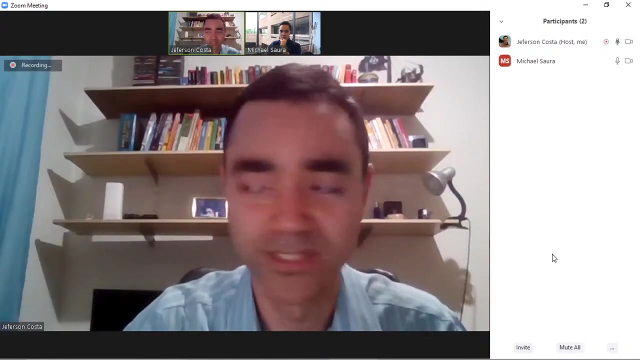 sure, yes, sounds good. ah, so if you need to share any screen, let me allow you to do that. so if you want to share anything, you are free to do that. okay, no problem, yeah, okay, this is like here, and while you are uploading your presentation, i have more, more tabula from south africa and moha. 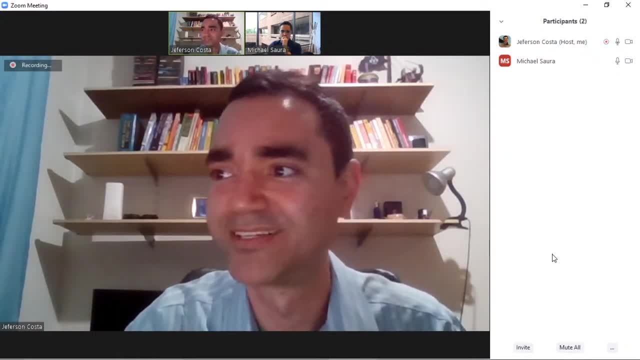 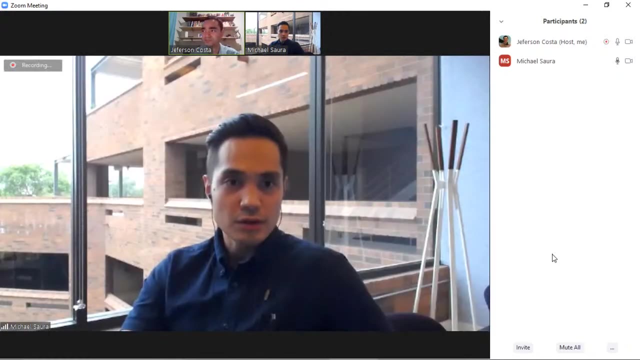 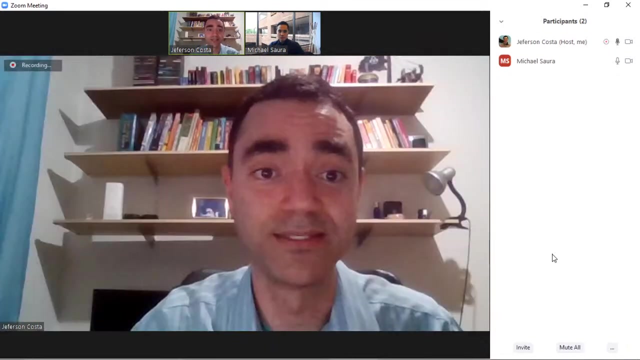 morais and from iraq. welcome, welcome, very, very nice people from very, very continence, very continence. okay, just a second here, and, guys, this is the while michael is preparing his presentation to show us. it is the last live session in in process interview live session that i was worried about. 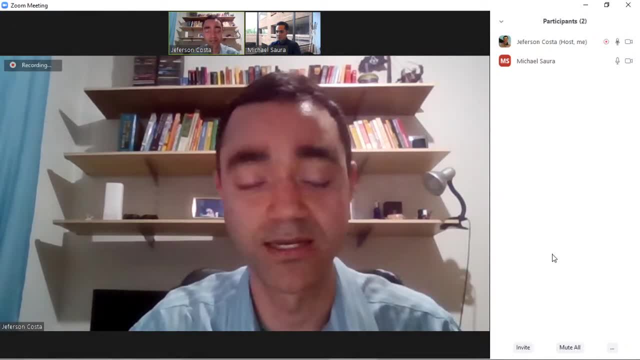 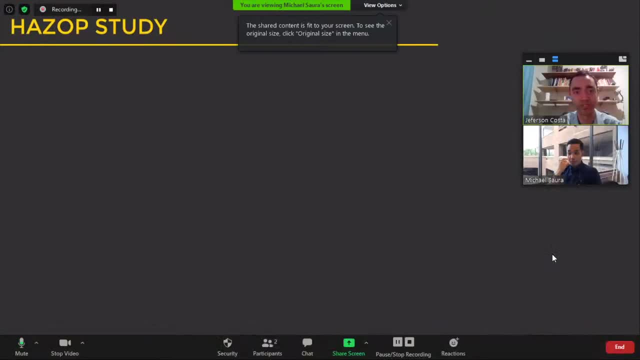 doing my schedule to not repeat the guest countries. i tried to do this first season to not get too much people from brazil, not too much people from india, for instance. so michael is finishing this this cycle and when we return i will not worry about that too much and i already have some schedules and soon you will know. 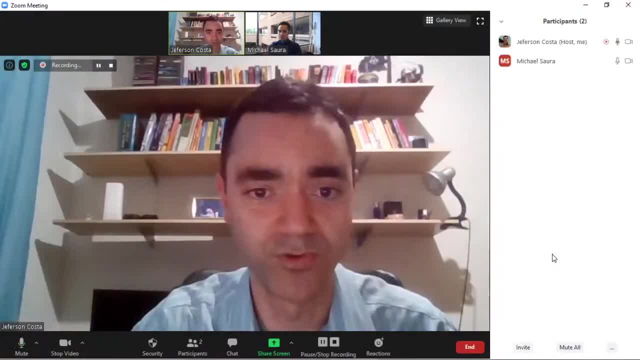 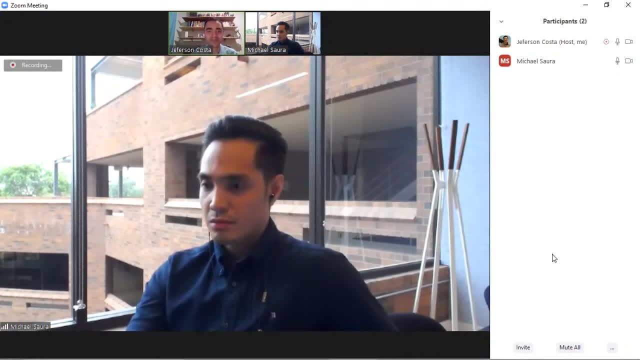 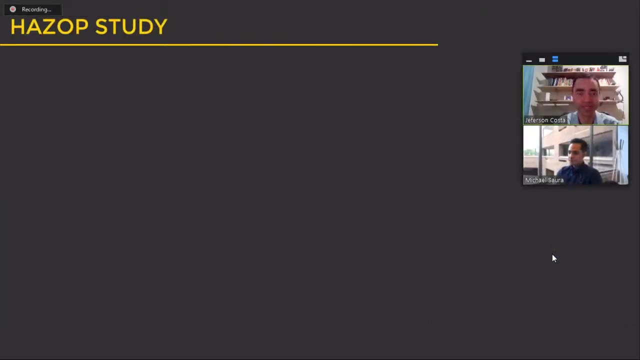 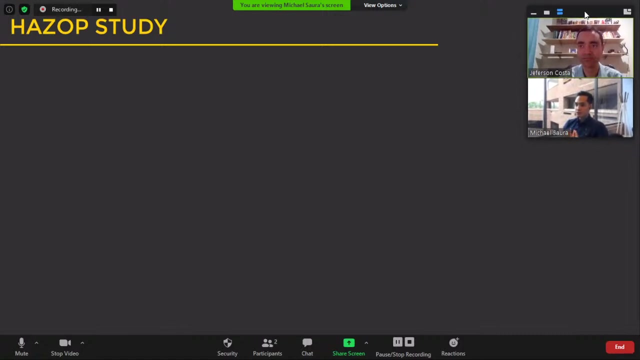 more about that. so, michael, it's a, it's free for you. yeah, okay, sorry, let's do that again, please, let me. so, let me know if you see my screen. yes, okay. so before i go into hazop study, i already mentioned process hazard analysis and process hazard analysis again is one of the key elements. 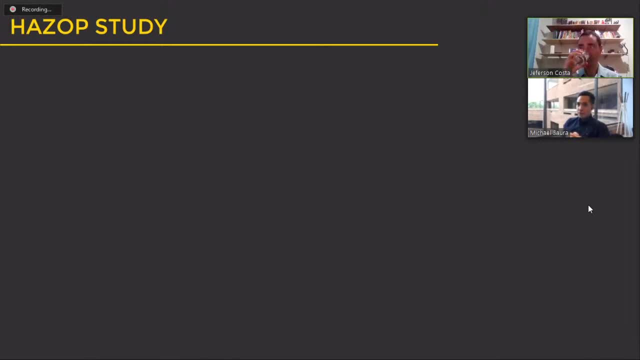 in process safety management. hazop is one of the ways or one of the methodologies that is widely used in the chemical processing industry to comply with the pha, and so the phd is to analyze and identify and analyze the hazards. the house up is a methodology and so has up really just stands for. 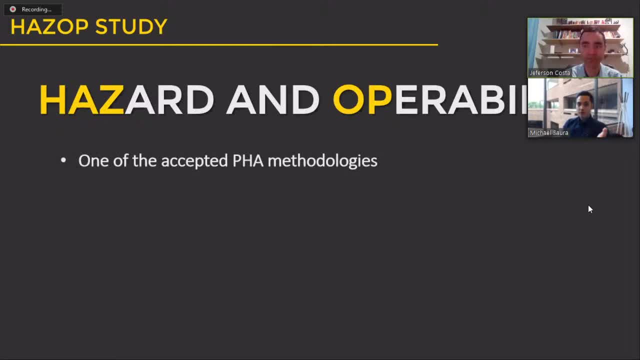 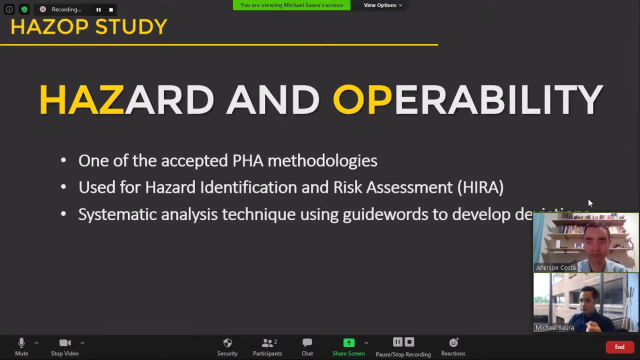 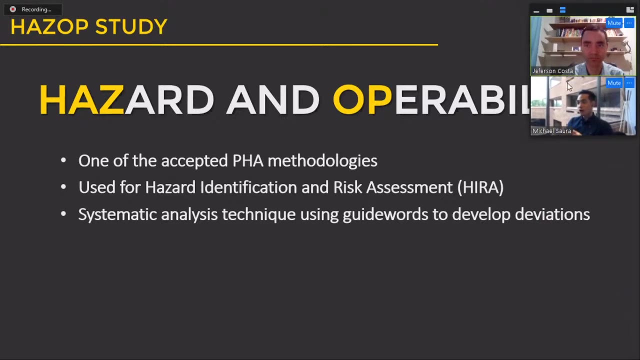 hazard and operability study. so it's one of the accepted phd methodologies. it's used for hazard identification and risk assessment. it's a systematic analysis technique that uses guide words to develop deviations and from the deviations you develop certain causes and that can lead to the deviations. 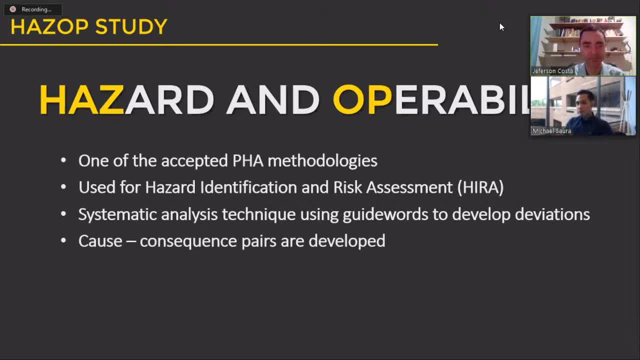 So it's usually a cause-consequence pair that you will develop when you go through a hazard and operability study. Typically, the information from the HAZOP is usually carried or migrated into layer of protection analysis, depending on the agreement between the HAZOP team. 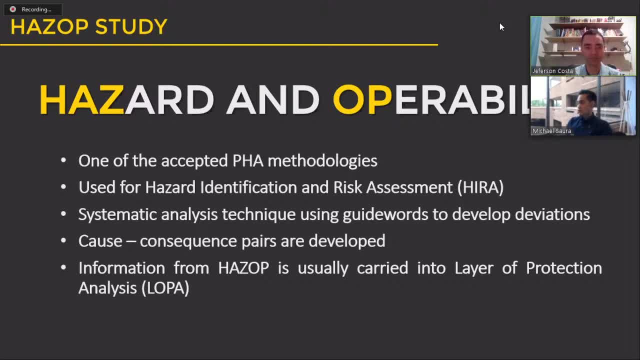 and the LOPA team. What is their criteria for considering into a LOPA or layer of protection analysis study? So, in a nutshell, that's what a HAZOP is as my definition, And it is a systematic qualitative technique. So the key there is qualitative. 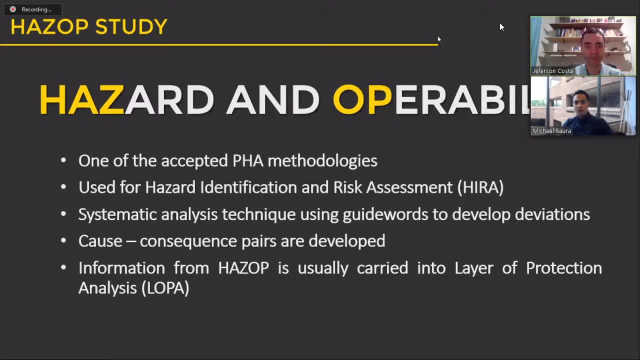 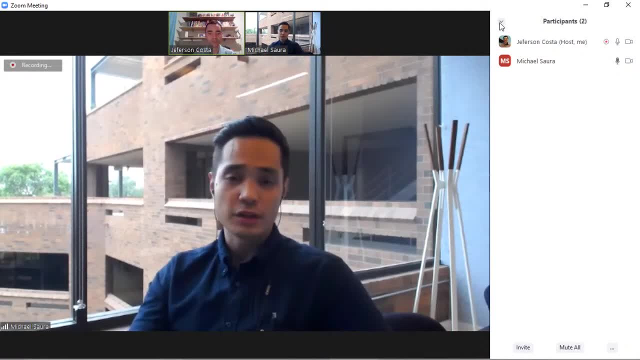 And again, it's used for identifying process hazards, And let me just go back to myself. So it's a systematic, qualitative technique in identifying hazards. right, With the guide words, you come up with certain causes. So for the guide words, you come up with certain causes. 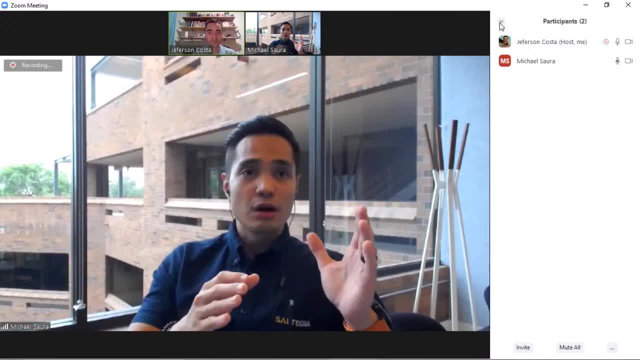 With the guide word methodology, for example, you've probably encountered low flow. So that's your deviation. The guide word is the low and the deviation is the flow. So you put them together now you have sorry. the parameter is the flow. 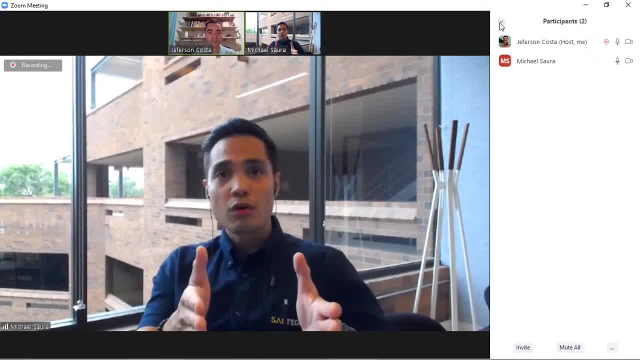 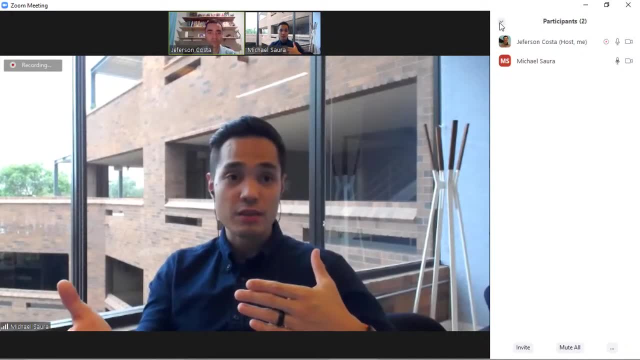 So you put them together, you now have a deviation of low flow. So with that low flow within a certain node, you want to talk about what can cause low flow in this node. So if we're talking of a feed surge drum, for example, for a certain unit, 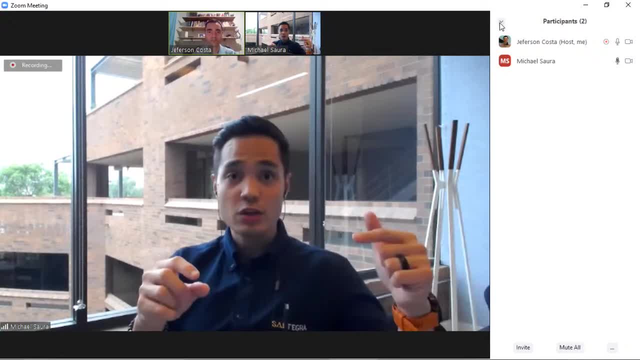 that whole feed surge drum in the line going into it is considered a node. So if you talk about what can you consider as a low flow case here, then the loss- losing feed to the feature drum- is a loss of flow And there's many ways of doing that. 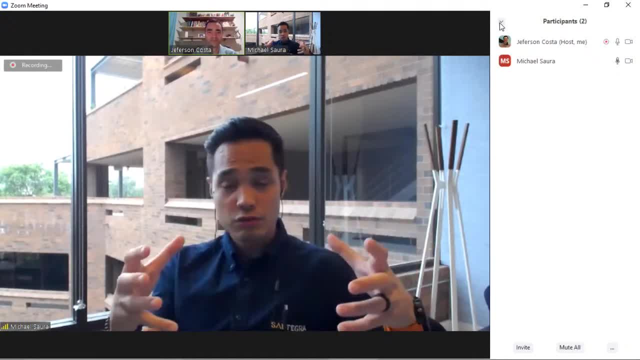 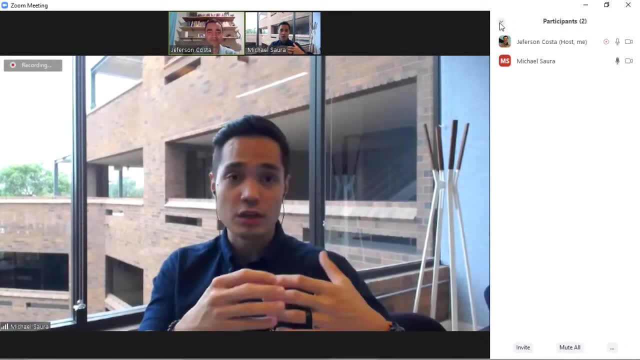 Either a control valve fails on the feed line going to the surge drum, maybe a pump fails upstream, So those are valid. No flow cases or causes that you can include into that deviation And I will show an example later on on what a typical has up looks like. 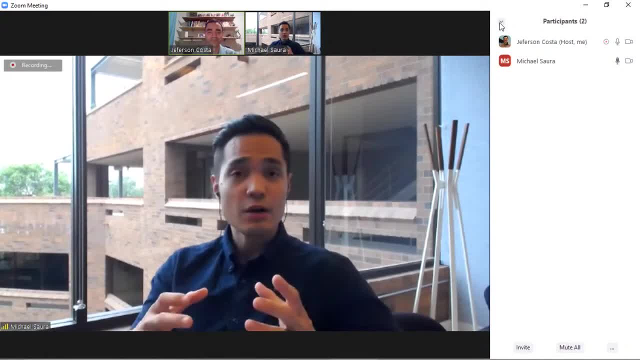 at least in how we do it. But that's how you go about: a has up And back then a has up. actually it's been evolving So before. has up is really mostly used for hazard identification, So you would identify what can go wrong. 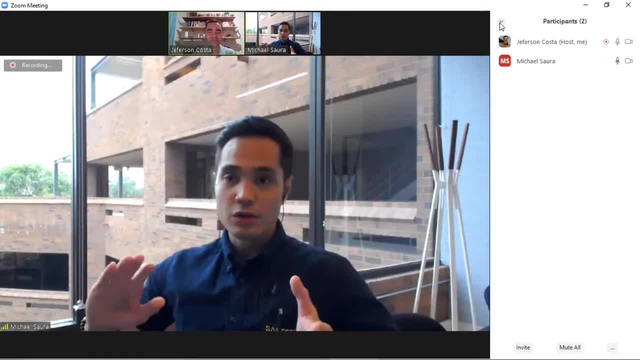 but they don't do any risk analysis, meaning they don't analyze what the severity is, They don't analyze what the likelihood and what the overall risk would be, And even what the safeguards are Before they would just list what can go wrong. 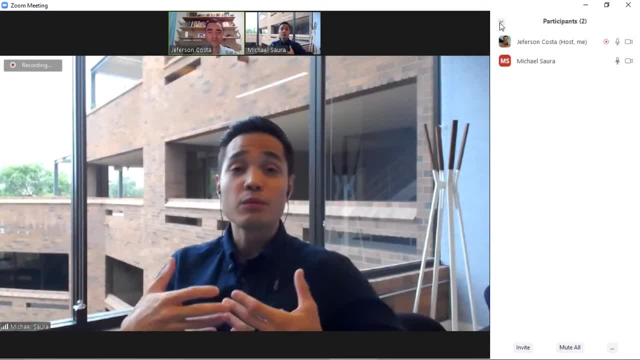 Sometimes they would list the safeguards and that's it. They end there, and then they would come up with recommendations to maybe prevent those scenarios from happening. So it evolved from that. So it evolved from that that to what currently is best practice right now. 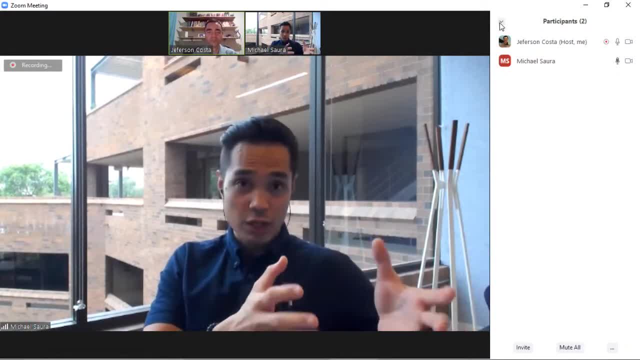 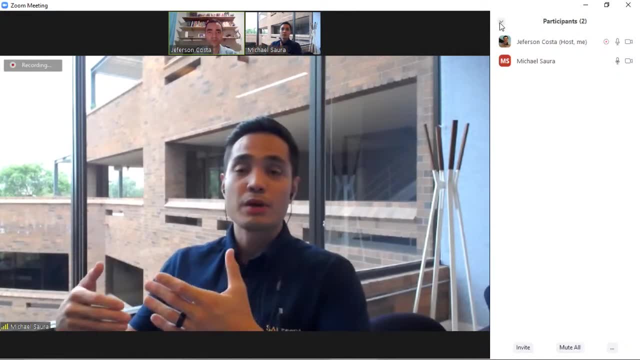 with the hazard identification part- what can go wrong- as well as the risk analysis part. So companies started developing their own risk matrices, which is basically a- I wish I said this- it's a representation of their tolerance to risk. One company's risk tolerance will be different. from the other, And so some companies consider a death their highest severity in just one death. At least one death is their highest severity. So to them that is extreme And they absolutely want to make sure that that doesn't happen. For other companies, five or more fatality. is their highest severity, And so you notice that there's a difference there. So each company would do their own thing, and that's okay. It really depends on what they are able to tolerate, right? At least in the US, there's no mandatory requirement. 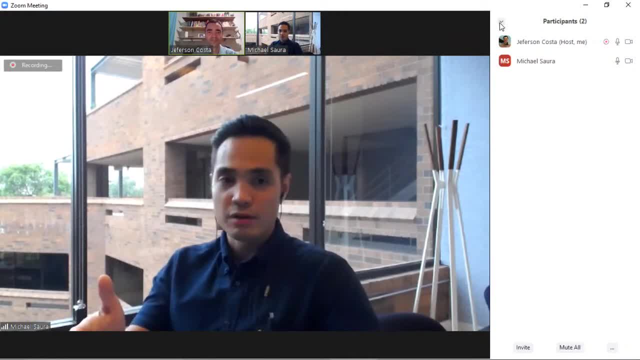 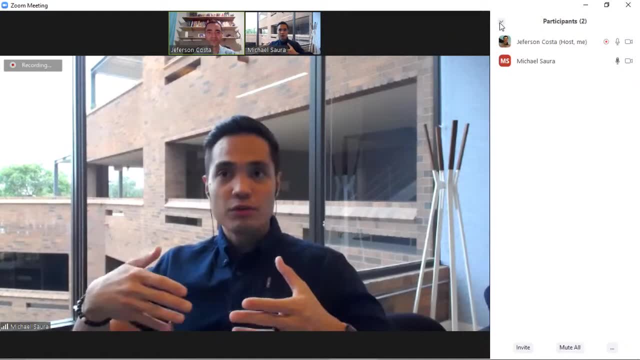 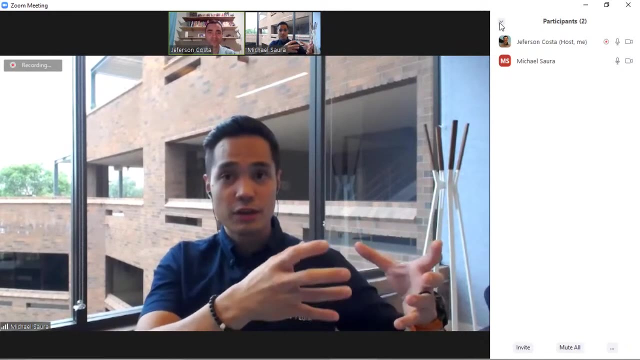 on what would be considered your maximum severity. It's not prescriptive that way, So, but I just wanted to give context that after that came about, it became best practice to do your hazard with both the hazard or identification of the hazards, what can go wrong- and then develop the severity. 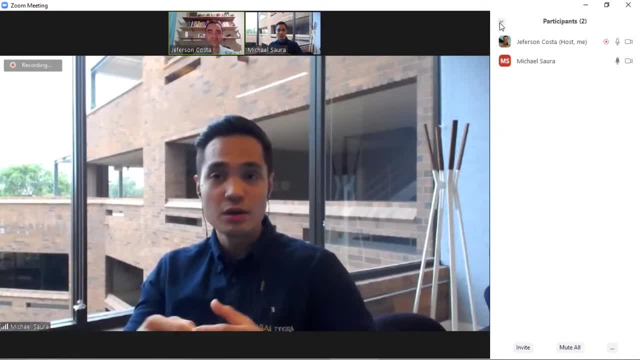 So what is the best practice? What is the severity of the consequence that we've mentioned, without any safeguards, And so I'll give a good example later on. Hopefully everyone will be able to follow along. But when we're doing a HAZOP, we always ask: 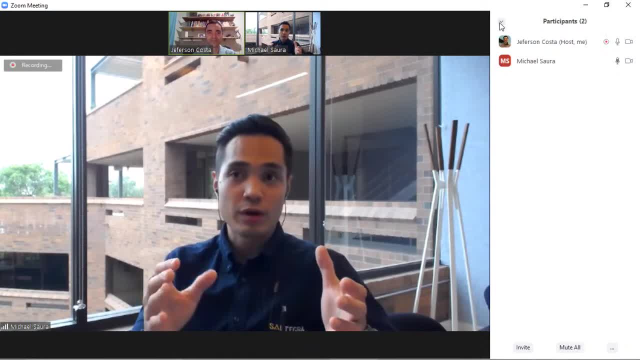 So for this consequence, if I, for example, for a pump, you have a pump, a centrifugal pump, and you block the discharge of the pump right And then the pump discharge was blocked. Maybe it's a control valve failure. 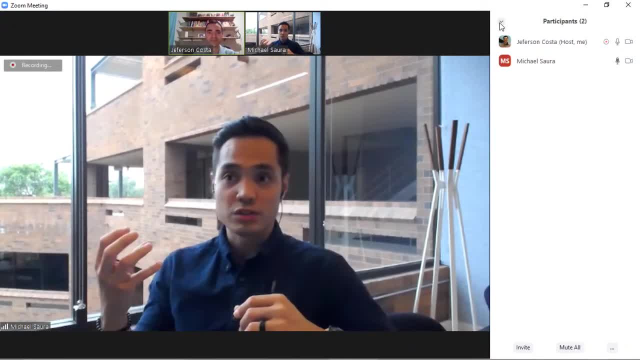 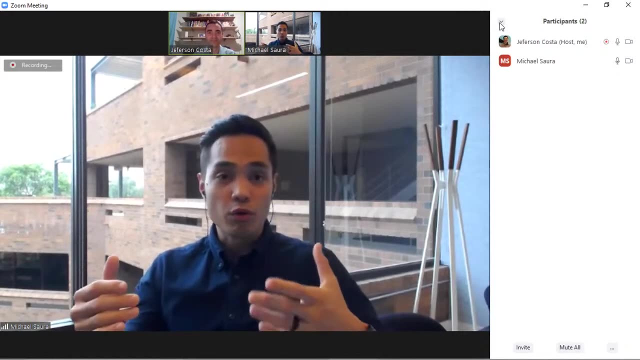 For maybe the loop failed or just mechanical failure. it stopped closed. So now you have a block pump correct. So over time, if no one did anything, when we say what is the consequence of this, We want to think of the worst credible consequence. 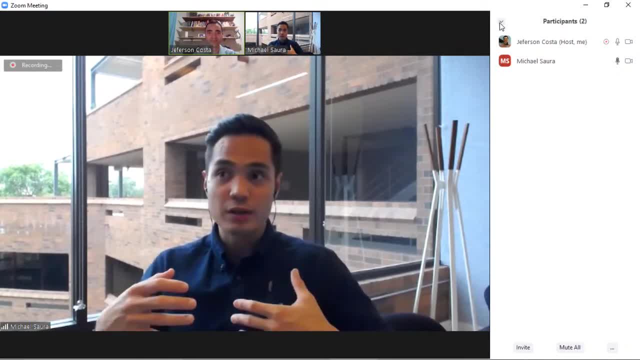 Some companies have different ways of doing the consequence, but I'm just gonna generalize it and say that typically you assume there are no safeguards. what will go wrong? There is no safety requirements for a block pump and for a prima templo bras Magna Block. 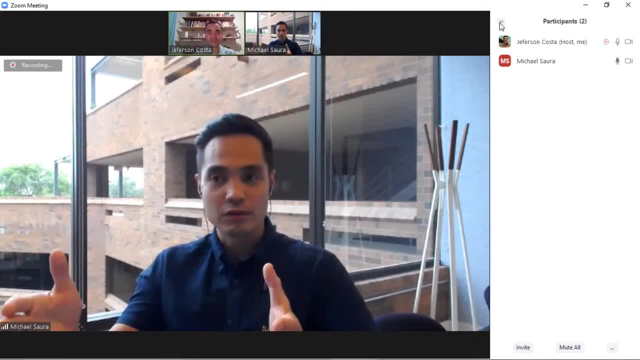 There is no safety needed for a block pump And disregarding any preventative safeguards, Okay, so for this case, for a blocked pump outlet, the consequence would likely be that head of the pump- meaning you, it's potentially gonna either overpressure the discharge piping. 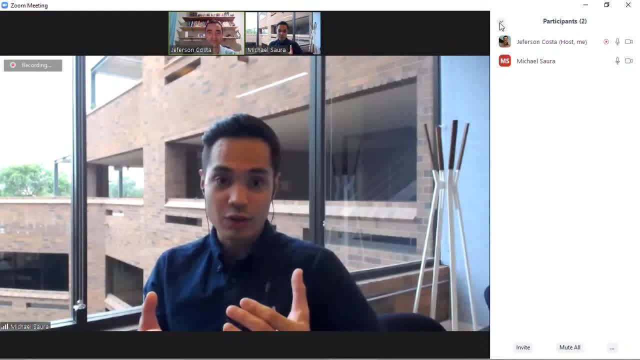 or damage the pump, seal and have lots of containment of material. If we're talking, we're talking about an LPG operation, then these are like Hydrocarbons that are going to be leaking out of the pump as well As we move up this slide and move to the next slide. you can see on this slide that I wanted to add a few things. 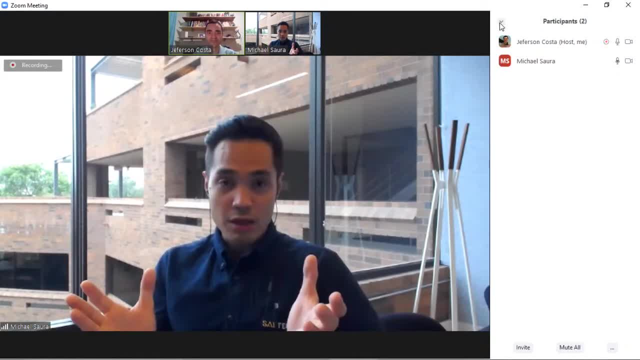 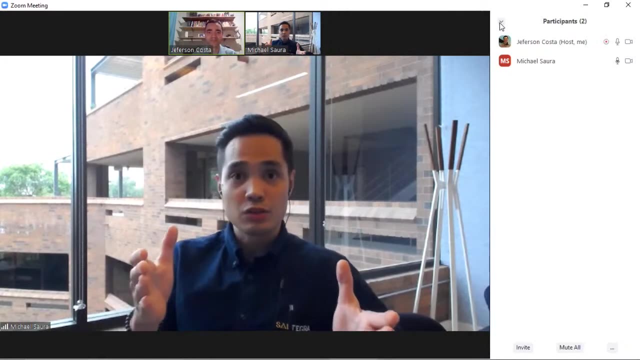 seal And if no one again did anything, you can have. if there's confinement and congestion around that plant area, you can have a vapor cloud explosion. So the worst when we do these things. some companies and some consultants already have specific guidelines because they've been doing. 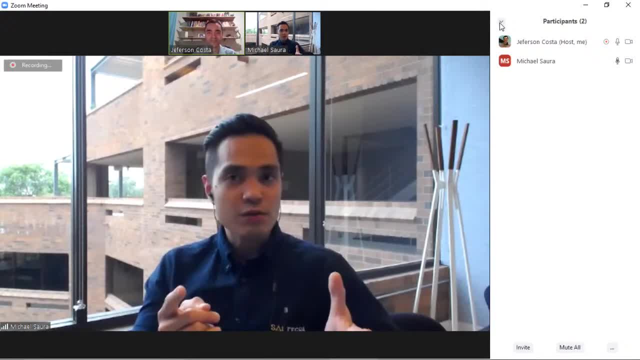 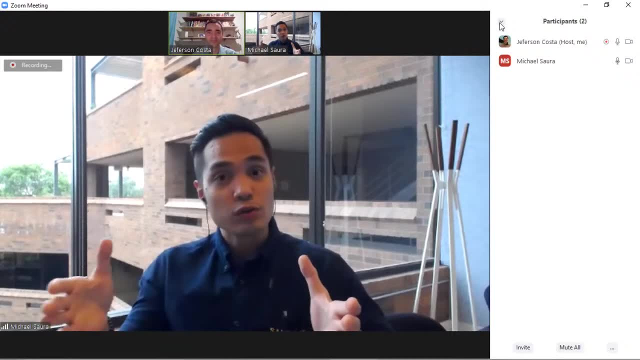 this for quite some time. So once they hear this scenario, they'll already know. yes, there's possibly a potential for vapor cloud explosion or not. But again, we don't want to go into that detail because we're doing a house up at this point. So you just want to brainstorm And later. 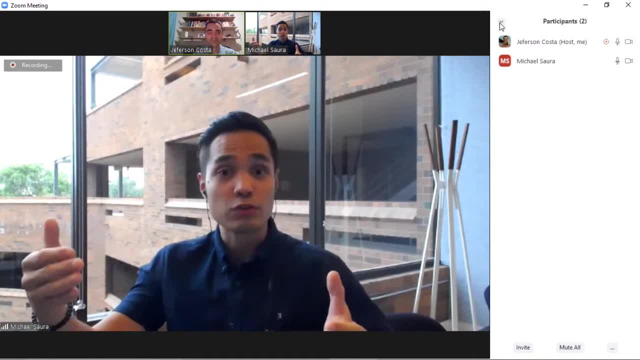 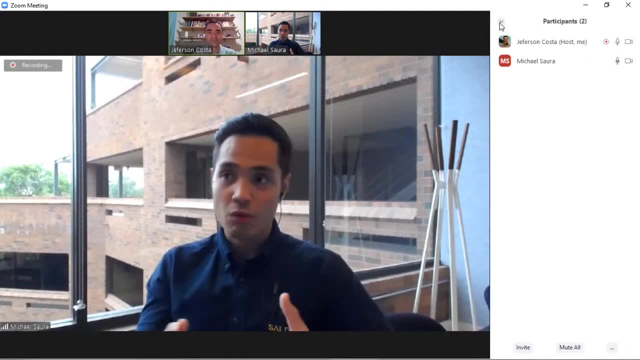 on. you can fine tune it if you go into the LOPA, which is more quantitative. So that's the worst case: Potential fire explosion, impersonal exposure or environmental impact, And people, because let's say, for example, the severity of that is a fatality right, At least one, So in your risk. 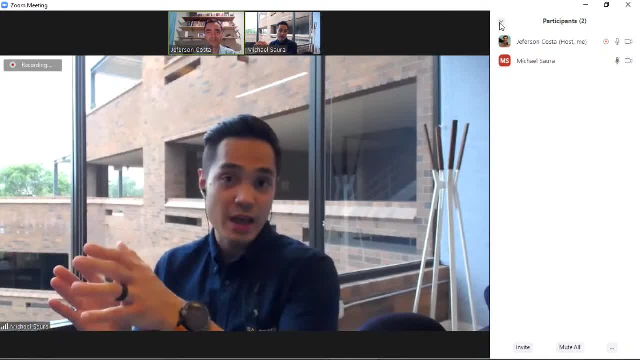 matrix. if your highest severity is, let's say, A, which is a fatality, then you assign A to that consequence, right, And so that's without any safeguards. So now that you know how bad it is, then you start. 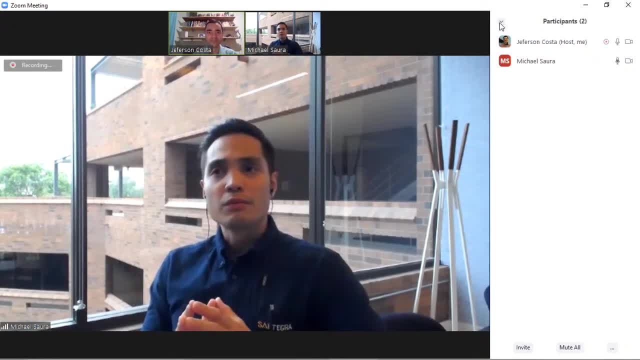 identifying your safeguards. So okay, the team would now start brainstorming: what do we have to prevent this? And so one operator might say: oh, I do have a low flow trip on my pump discharge, So that can be a valid safeguard. So you can credit that. You need to identify what's the trip. 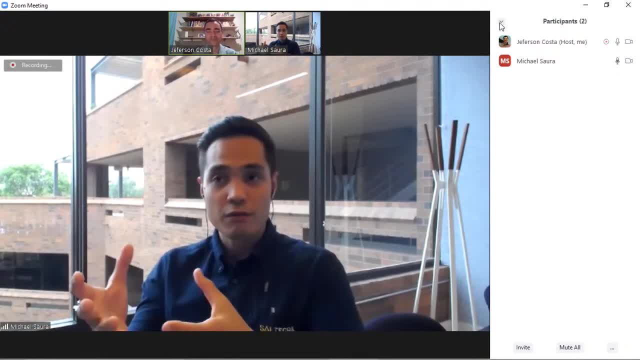 set point. you know what is it going to do. So obviously this will trip the pump to prevent addition of any energy and to prevent the seal failure. So that's one, And then another one perhaps is a pressure relief device on the discharge of the pump which will relieve to. 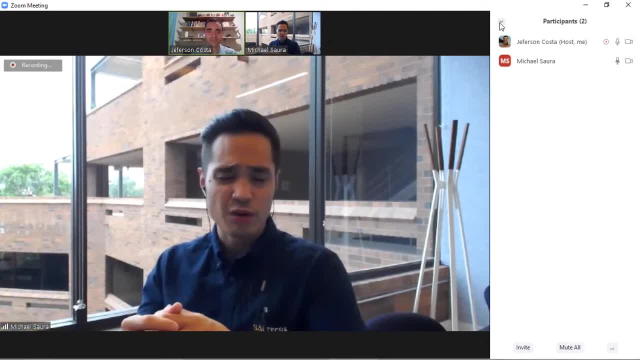 maybe a flare system or another open-closed area, or maybe to a safe location, If it's sized for a block in case, then it's a safe location. So that's one, And then another one perhaps is a, and you can credit it as a safeguard, and so on. So now, after you've identified all your safeguards, 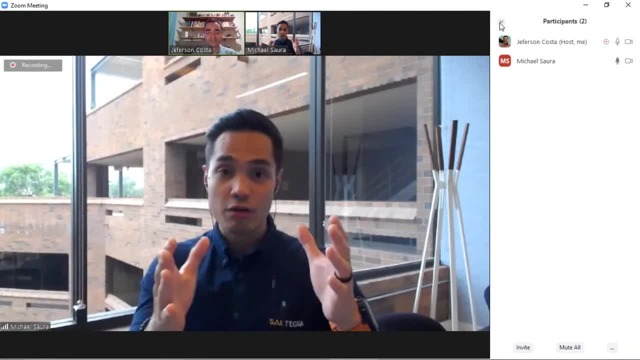 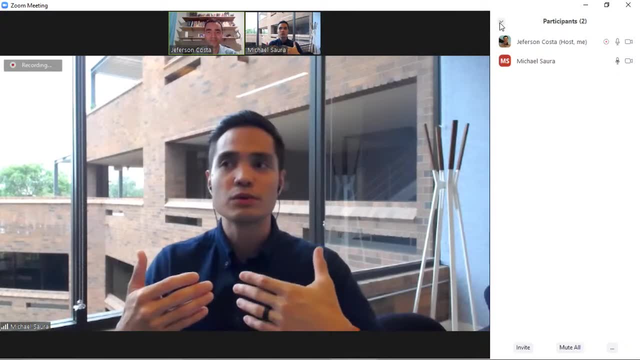 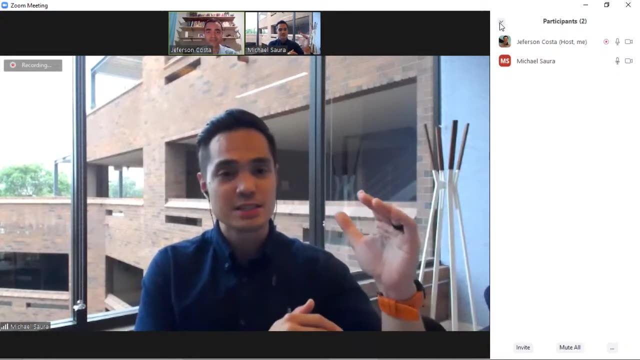 you go about identifying what is the likelihood of this scenario. So this is where also one of the qualitative parts will be. The team needs to come up with the likelihood based on the criteria that their risk matrix has set. So there are certain generic risk matrices out there, but 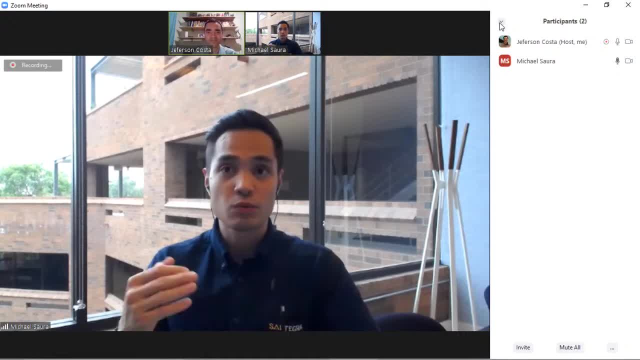 let's say for this particular scenario we'll say it's one, It's highly unlikely, And so in the risk matrix that one and the severity of a A to them is considered an ALARP as low as reasonably practicable, which is basically saying that it's as low as it can be and we can accept it. So the 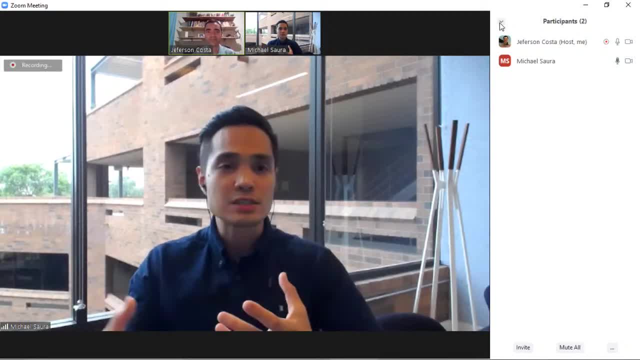 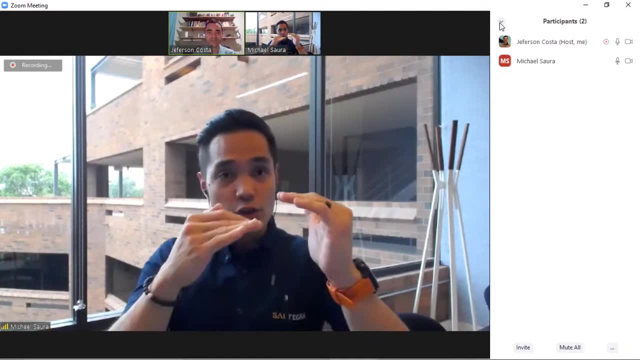 team has to decide whether or not it's acceptable. It's a team consensus-based analysis. That's why it's qualitative Okay. So yeah, that's how you go about typically a HAZOP study, And then you go. so that's just one cause. There are multiple causes, And even for one cause there can be. 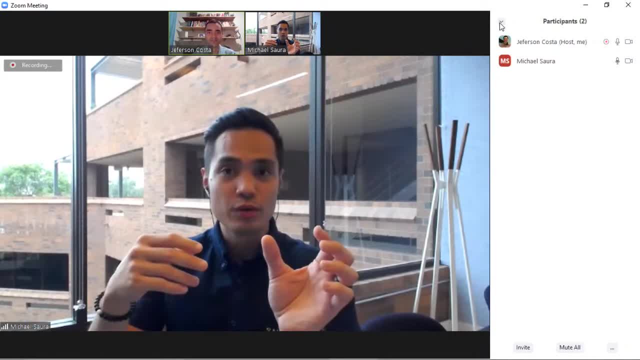 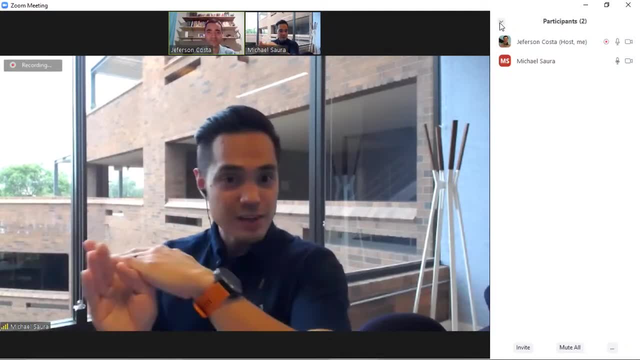 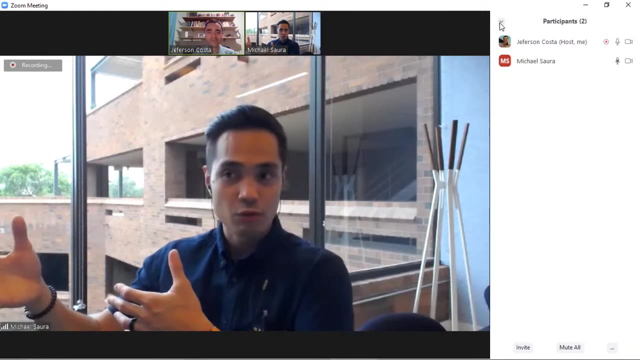 multiple consequences. So for that block pump discharge there can be consequences downstream of the control valve. that was blocked right Because you're feeding something with a pump. So if you're feeding, let's say, a fired heater, right, That's, you know, with a gas-fired heater. 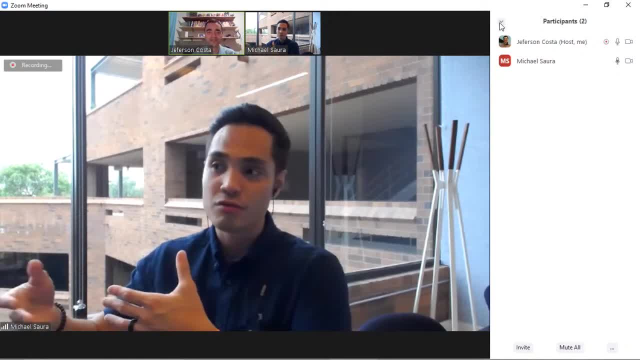 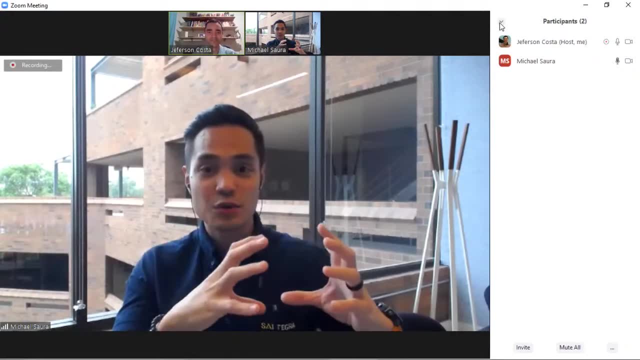 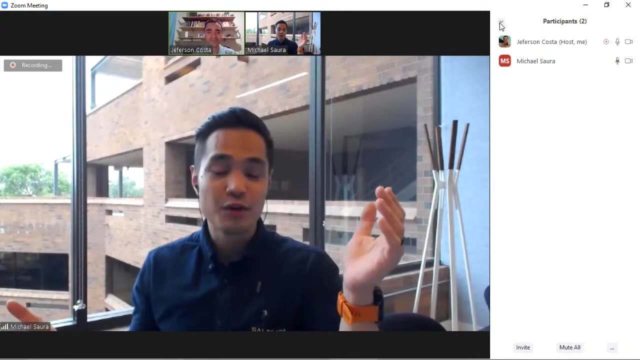 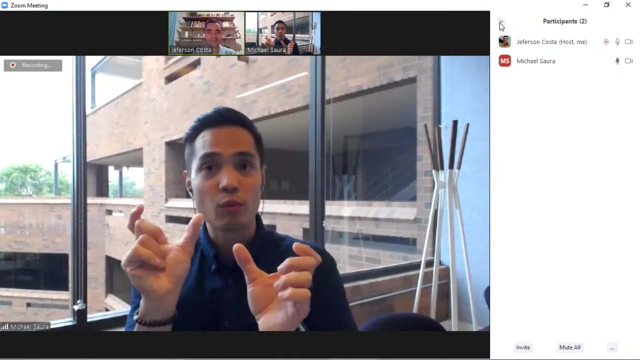 that fired heater might also have a consequence of coking and maybe tube rupture. So you have to also add that consequence into the same cause. So this one cause can have as many as 20 consequences or more, I don't know. But the team has to understand which scenarios are credible and 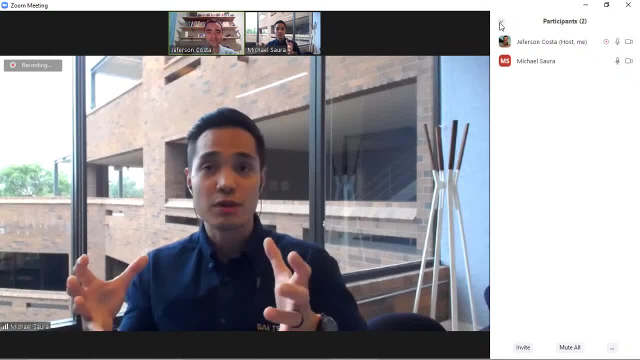 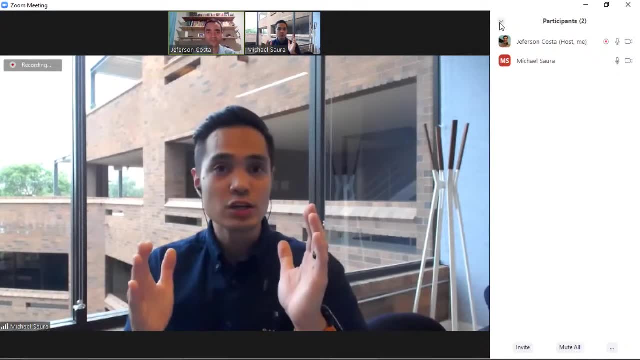 what can be immediately seen And it's up to them to see, Or probably the company has rules as to how far do they want to take it. But in general you look at what happens immediately upstream and downstream of the cause. So at least those 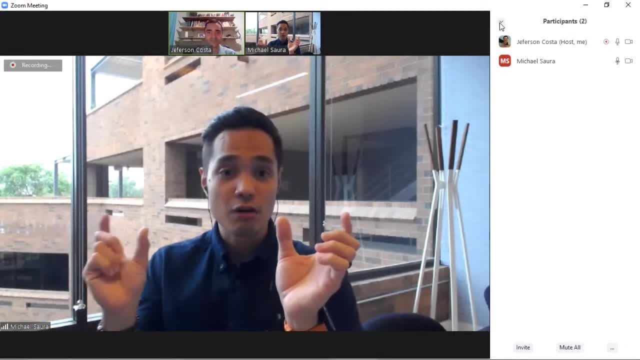 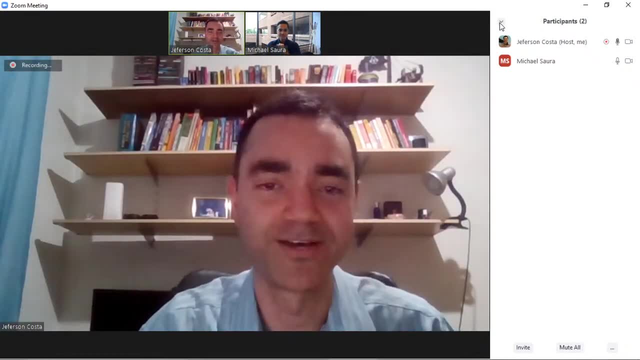 two will most likely feel the effects of the block flow case. And guys, this was just one example. Now imagine this in a meeting room with many people talking about that. And Michael, how should be the best size of a HAZOP team And how important is to have the experienced people? 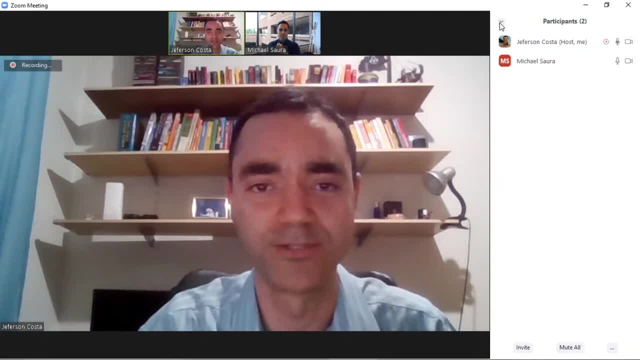 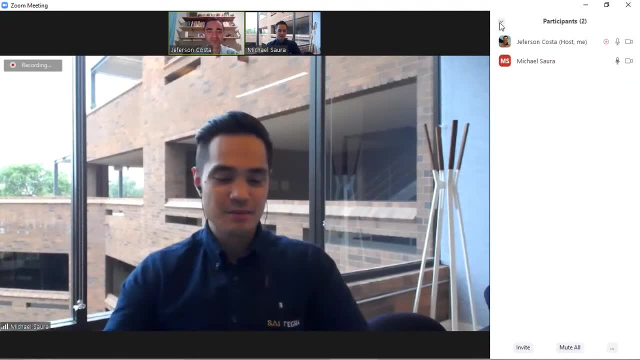 and fresh people in the HAZOP? That's a great question, Jeff. I always get asked that question. I was just doing training this week And that's one of the questions that were asked: How many people should we have in HAZOP? So I'm going to tell you: not 20.. 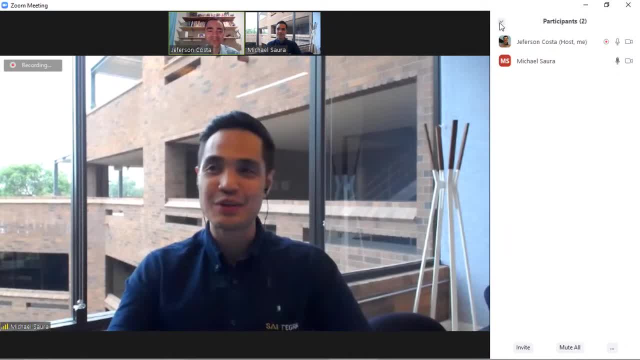 So don't have 20 people in the room. It's not providing any value. I understand that there's a lot of people who want to contribute their thoughts, But keeping the team between five to 10, 10 is usually a magic number- is essential so that people can have the opportunity. 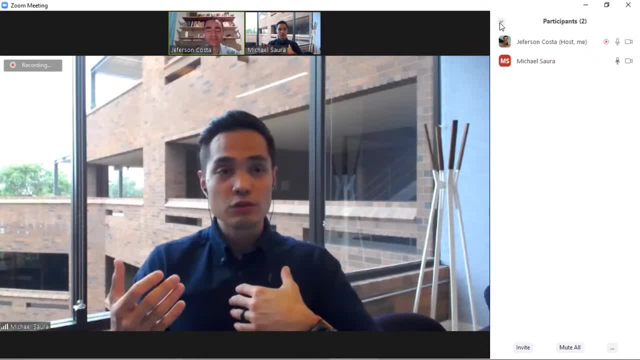 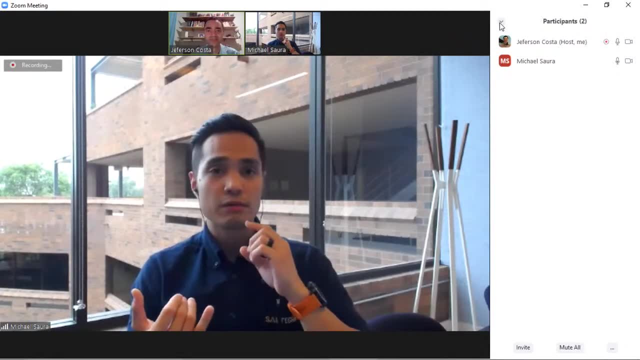 to speak, And usually the core people that you would want in. let's say, if we're talking about just a current, an existing plant, you would want to have the process engineer there. definitely You want to have an experienced operator, perhaps a maintenance personnel, also controls engineer. 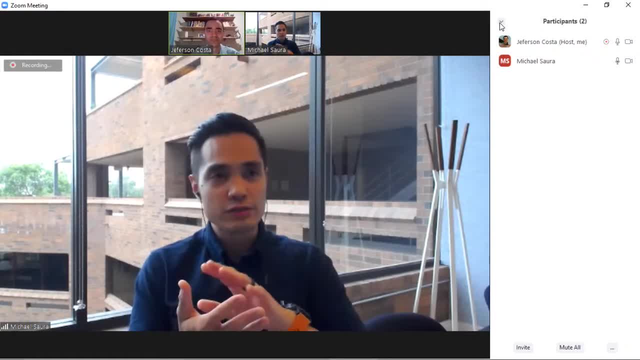 process controls. If you're doing LOPA, then you add some more people like instrumentation engineer and perhaps a subject matter expert on the unit or the process that you're working on, So they can be full-time, But the primary people would be, of course, the facilitator and the scribe. 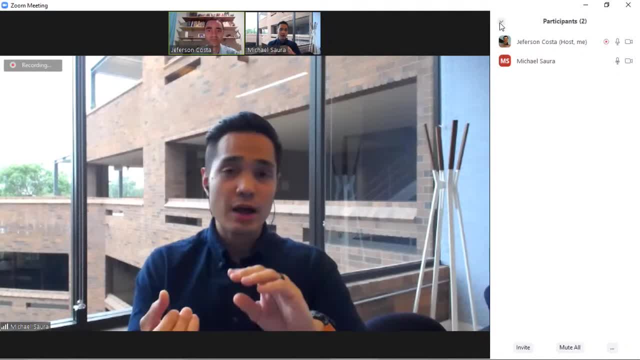 depending on who you're working with, But definitely scribe facilitator, operator, process engineer, process controls engineer. typically is what I've seen in the scribe. if they're required for the study As you go into LOPA then you'll add more people. So, as you can, 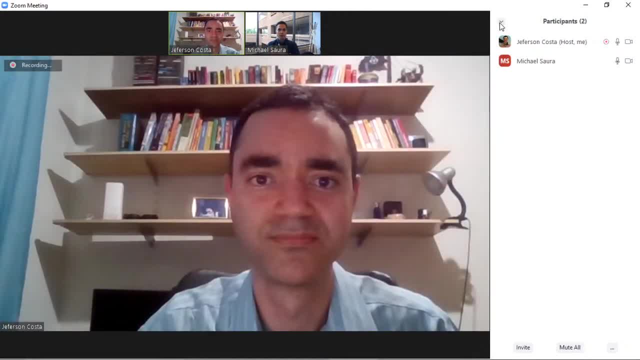 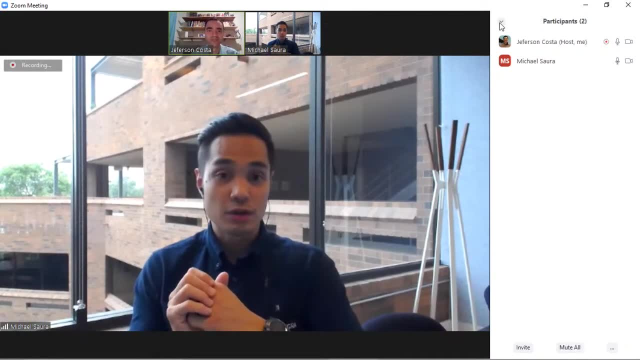 see that's around five, right, And then you can add more if you have a lot of damage mechanisms or corrosion-related scenarios, and you can always bring in your experts in for damage mechanism or corrosion personnel. So, but definitely need experienced people. Your house-up is only as good as the information that 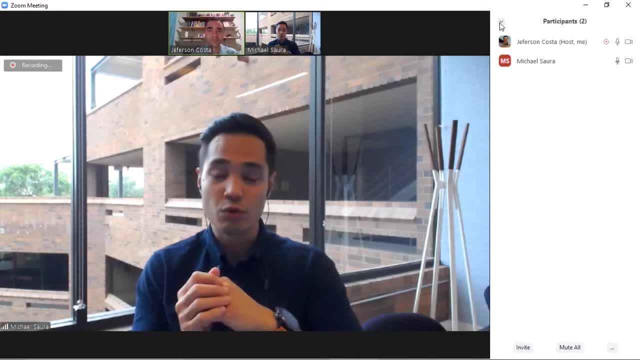 the team can bring, And so if the people are experienced, then you will most likely have a high-quality house-up And, of course, a facilitator who knows how to properly lead the team and also understands the process a little bit or more is better, of course, if they're able to understand, Because 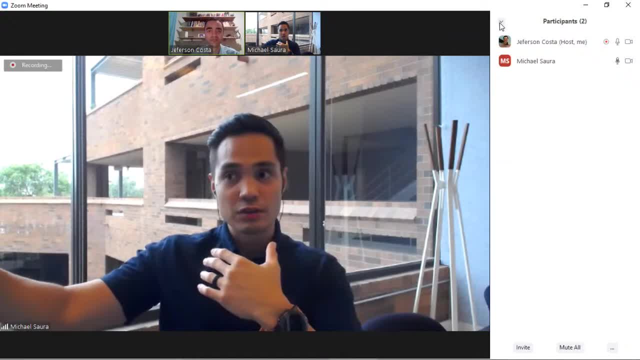 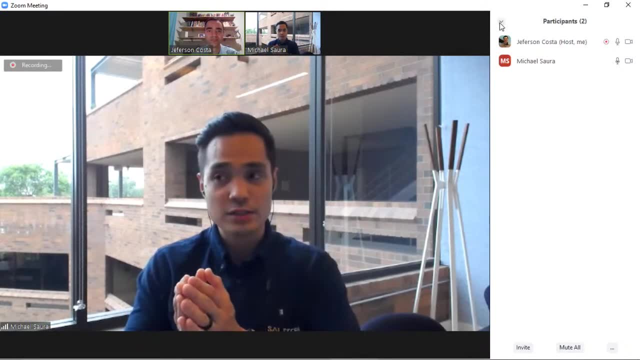 sometimes if there's a lack in experience on the team side. if the facilitator knows the process and what can go wrong from that type of process, then they can always suggest. But key thing here is the facilitator mostly needs to know how to handle the team, And so they can always suggest. 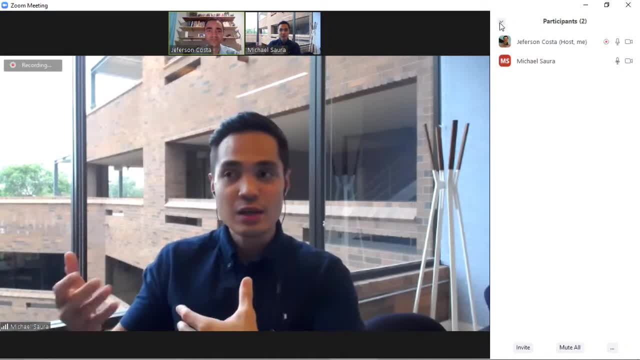 But key thing here is the facilitator mostly needs to know how to handle the team And so if the people are experienced then they can always suggest. But key thing here is the facilitator mostly needs to facilitate and get the team to talk and listen, But sometimes you get stuck. So the facilitator- 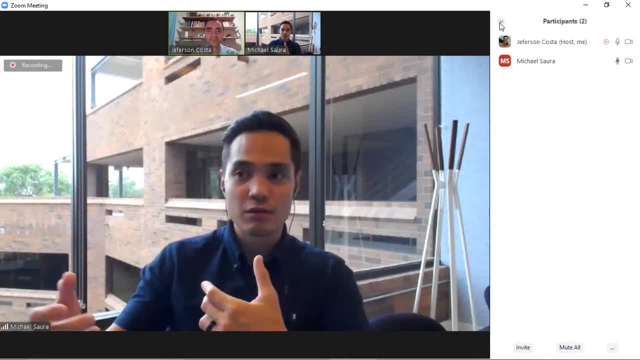 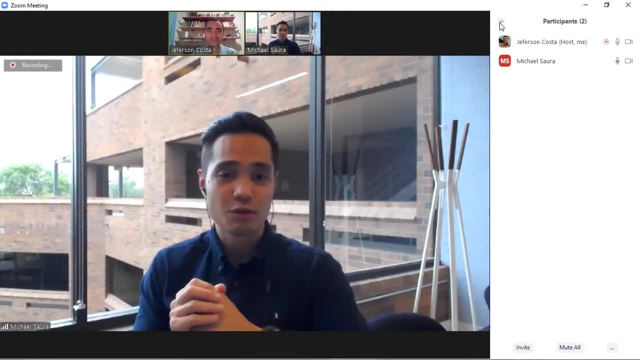 must also be able to pull information out of them or suggest if the team is lacking experience in that regard. But that's a very good question. So five to 10.. Thank you, Yeah, So I know that I promised a quick house-up example, And so let me. 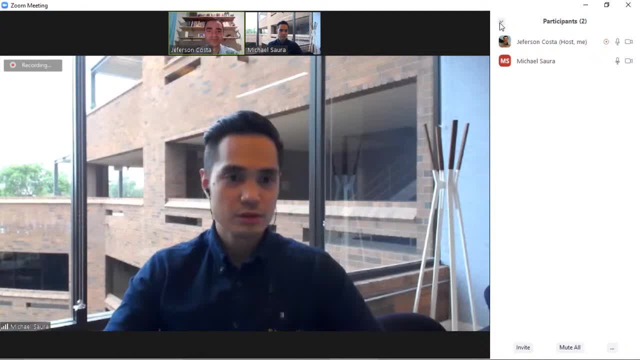 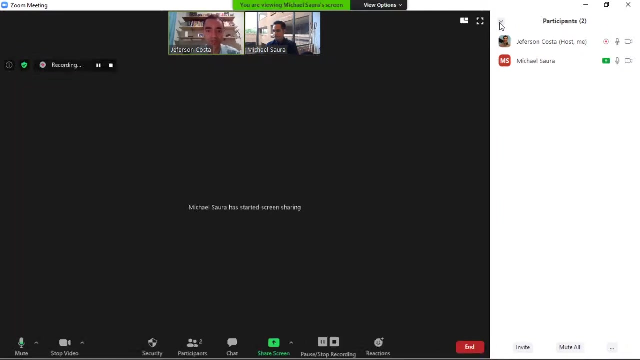 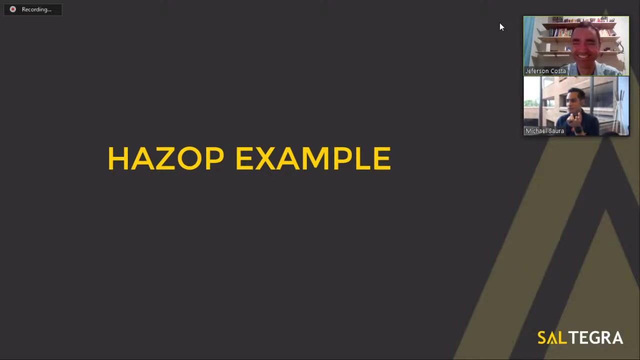 just pull this for everyone. Okay, You talk a lot and we chemical process engineers are the engineers that like to see drawings. okay, Like to see drawings? Yeah, Oh, no problem, Here it is. So this is. do you see my screen? 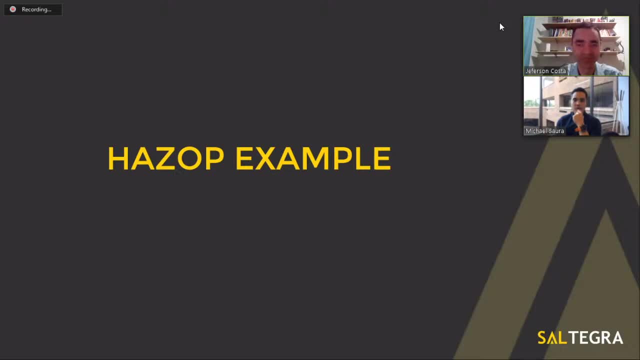 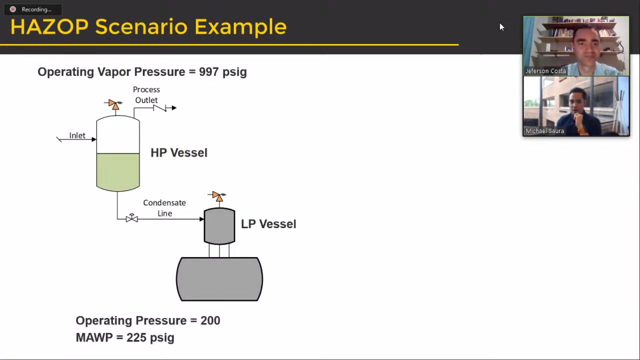 Yeah, Yes, yes. Has a lot of example, Perfect. So this is just. this is an example. It's not representing any sites that I have worked on, but this is an example of a blow-by case. So you have, and this is again. 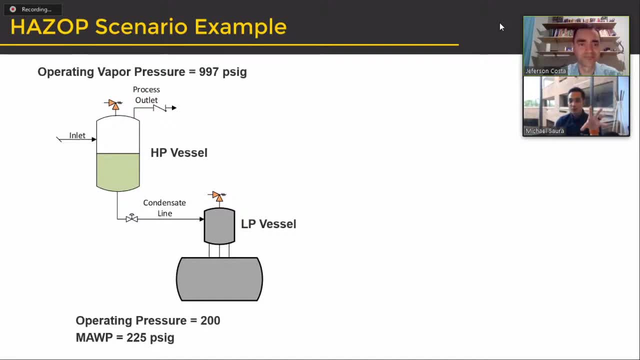 this is just generic representation, So there's not going to be any too much detail here. The goal here is just to understand the scenario. okay, So you have a high-pressure vessel here. Let me use my pointer: You have a high-pressure vessel here operating at 997 PSIG. 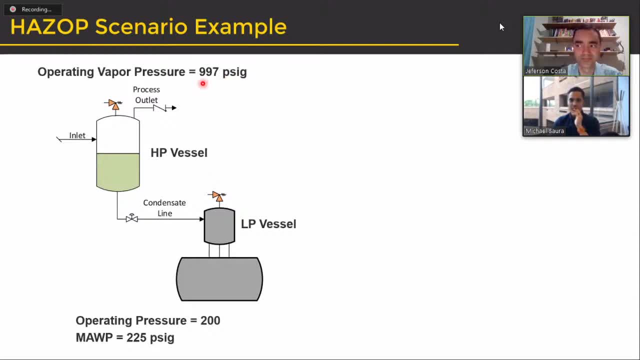 I'm using PSIG and American standard, but just bear with me here. 997 PSIG and there's a low-pressure vessel that goes operates at 200 PSIG with an MAWP of 225. So the scenario here is that this valve malfunctions fully open. 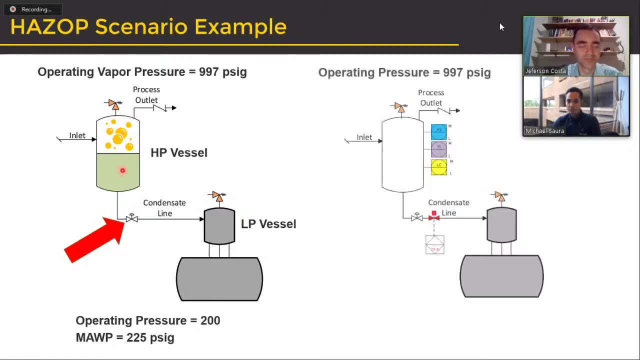 So this, as you can see, has vapor and liquid. So, in the event that this valve goes fully open, your vapor, well, your liquid level will first drop and if no one did anything, without any action, any safeguards, eventually your vapor phase. 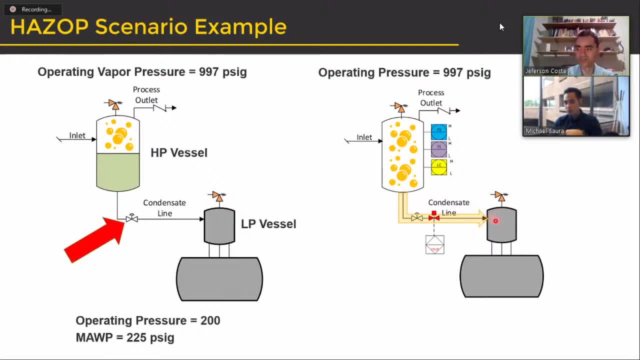 your vapor will start blowing into your low-pressure vessel site. Please ignore the condensate line for now. That's not a condensate line. This is a hydrocarbon vessel, So you flow into your low-pressure vessel, So what'll happen is that this vessel will now experience. 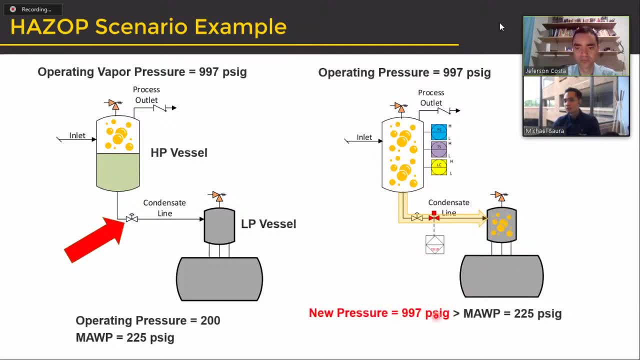 the new operating pressure of 997 PSIG. You guys still with me. So 997 against 225 PSIG usually means over-pressure, because now your vessel is operating, or should I say is experiencing a pressure that is not supposed to be. 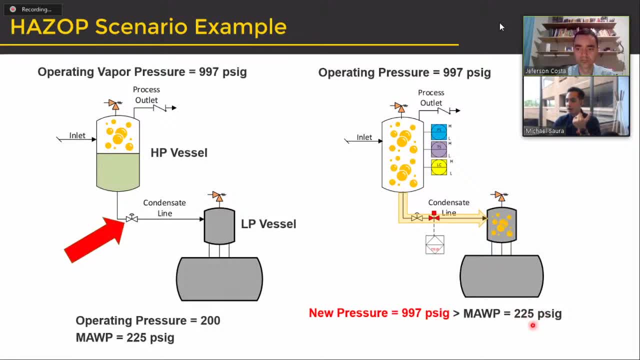 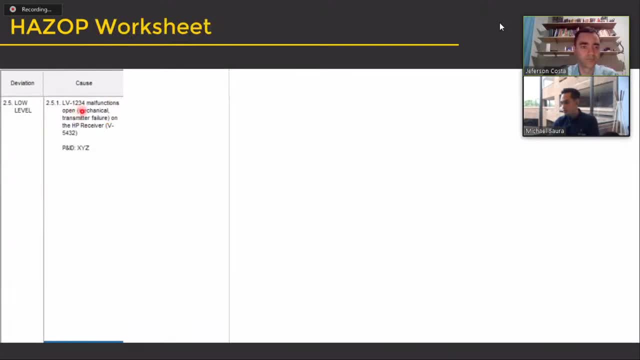 operating under, because it can only handle 225.. So in a HAZOP worksheet, let's say, for example, that: can you read this, by the way, And everyone? is it readable? Yes, yes, Okay. So this deviation is low level. 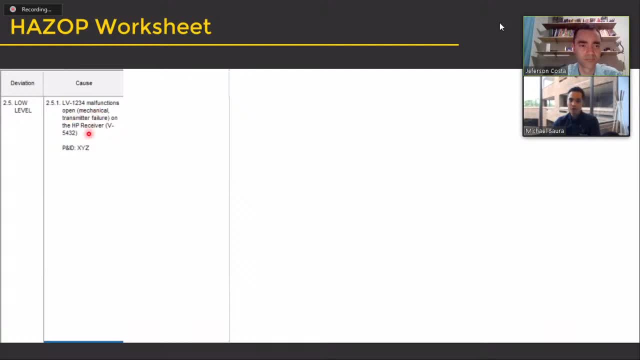 So the cause is LV1234 malfunctions, open or you know, because there's probably mechanical failure, transmitter failure on the high-pressure receiver On this P90,. the consequence is, without any safeguards, low level in the high-pressure separator and gas volvi of 997 PSIG into the low-pressure separator. 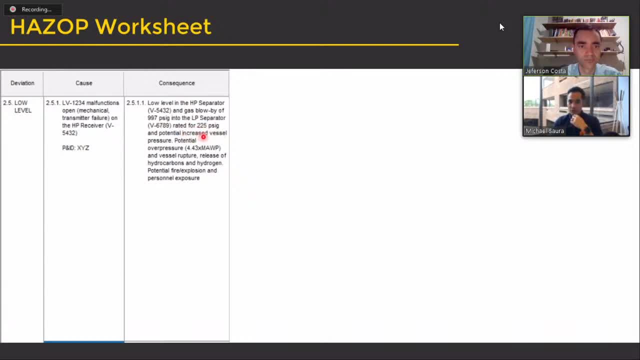 which is rated for 225, potential increased vessel pressure and potential over-pressure, which is 4.43 times MAWT. So why is this important? This is important because you want to understand what the ratio is of the consequence. There has been studies. 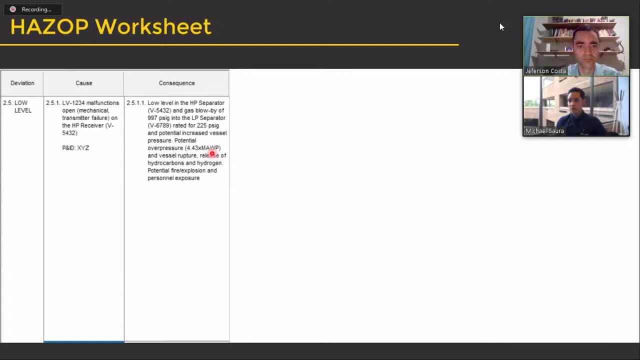 and this has been very well documented. but one of the known incidents, the BP Grange move incident. similar scenario: a blow-through of high-pressure vapor got into the low-pressure separator And the ratio of that scenario was 3.5 times the MAWT. 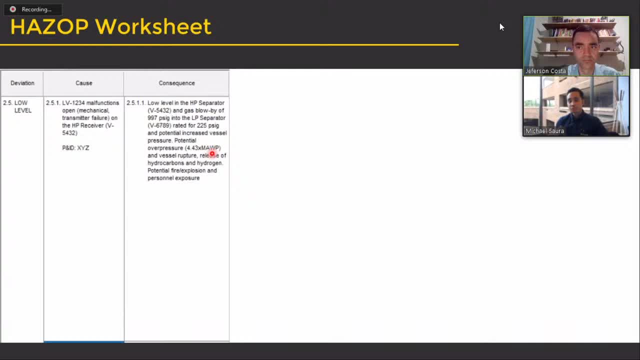 So if your vessel, for example, is, if your downstream vessel, the low-pressure vessel, is operating at 100, MAWT is 100 PSIG and your upstream pressure is 350. So if that 350 got into the 100 PSIG vessel, 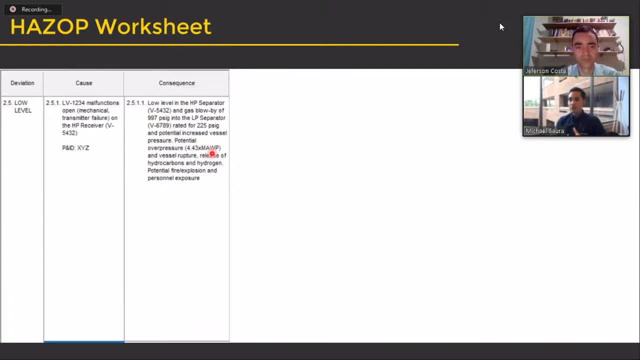 that's a 3.5 times MAWT. And why is that important? Because when that happened, the low-pressure vessel ruptured and shrapnels flew out from you know, there it was and there was a big explosion. So they started analyzing that. 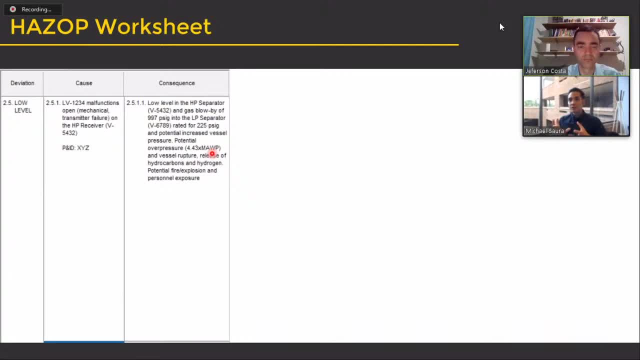 and there were various studies revolving that, And so it seems like the- at least the petrochemical industry, had identified that 3.5 times the MAWT is a number that you can expect rupture to happen for sure. So that's why we usually 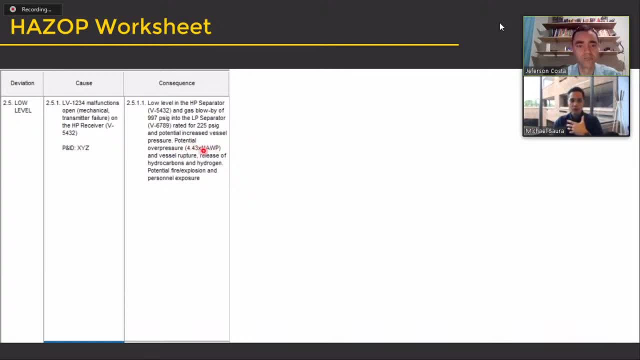 in our locals at least- for overpressure. we try to determine and identify that so it's clear what the what the ratio is and what the possible consequence is. So this is a vessel rupture. That's why you see that here. release of hydrocarbons and hydrogen. 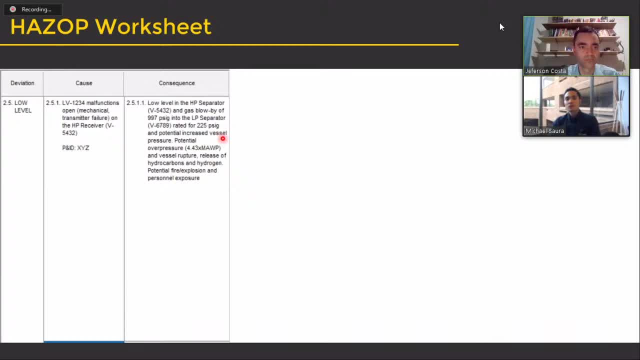 potential fire explosion and personal exposure. So you'll notice that we don't take into consideration as a present. So this severity for that company, for example, considers it as an A consequence. It can possibly have, you know, multiple fatalities, right. 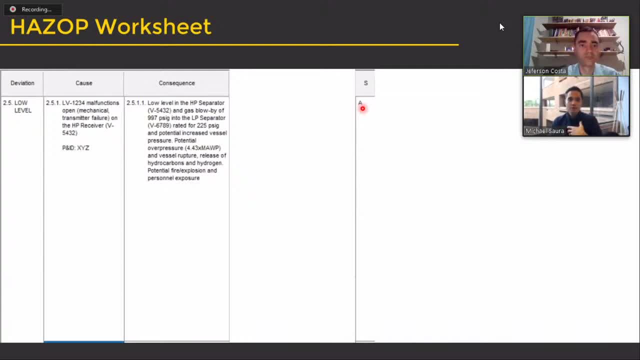 More than one. So to them, that's their A severity Now that we know how bad it is, based on the scenario and the risk matrix that the company has, we identify our safeguards. So one safeguard would be an alarm that has a high or low deviation. 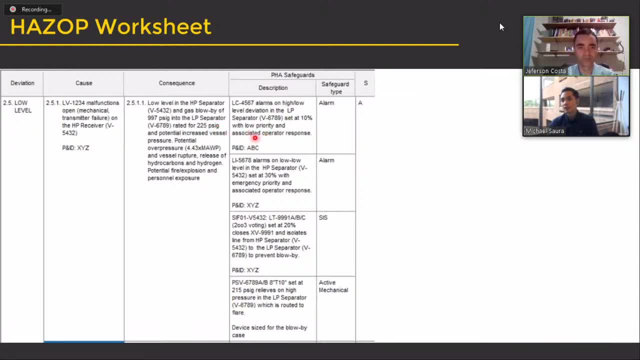 on the low pressure separator. That'll indicate that, hey, my pressure- I might sorry, my level is going up and it's higher than what it should be. So that's an alarm and an associated operator response. The next one is also an alarm. 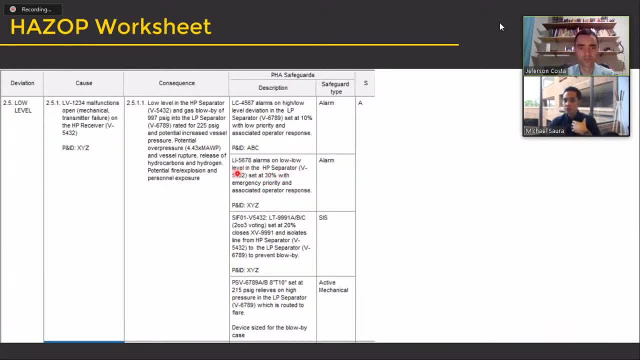 on the high pressure separator with a low, low level set point, which is at 30%, with an emergency priority, So a high, very high priority. people must do something about it with an associated operator response, And then there's a SIF. 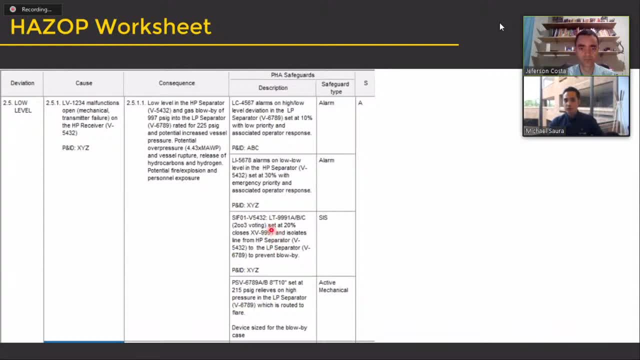 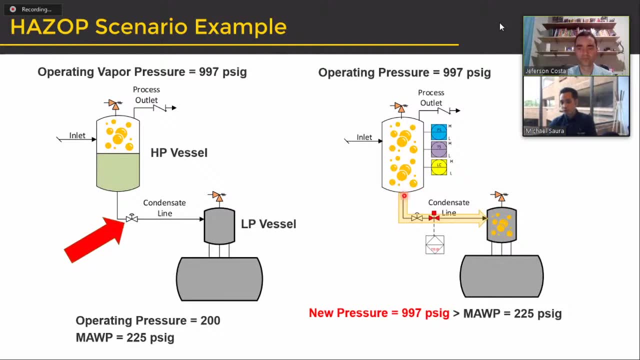 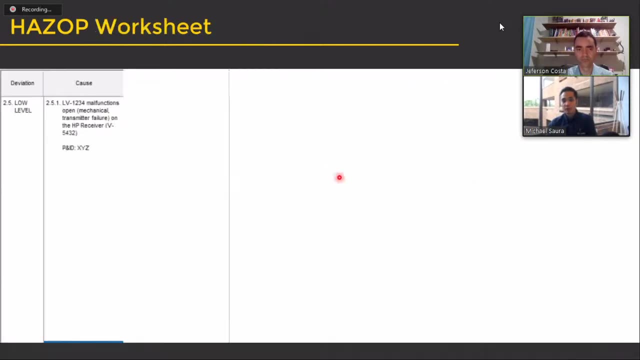 safety instrumented function that would isolate the, which is this one. it would isolate the vapor line or the sorry this line right here, Once it detects that this vessel has lost level or at least has met the condition of 30%. 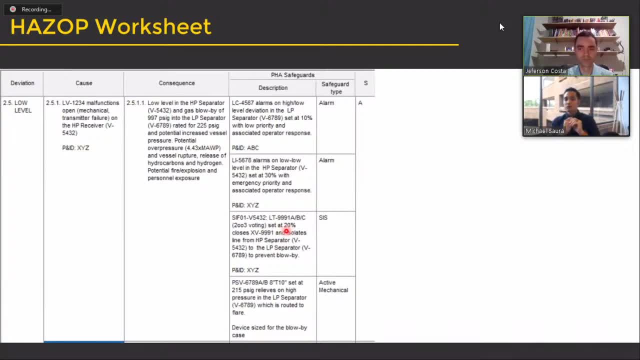 sorry, 20% set point and it closes that valve to isolate the vapor. So now we don't have vapor bloating, right. But then again there's also another safeguard, which is a set of relief valves or process safety valves. 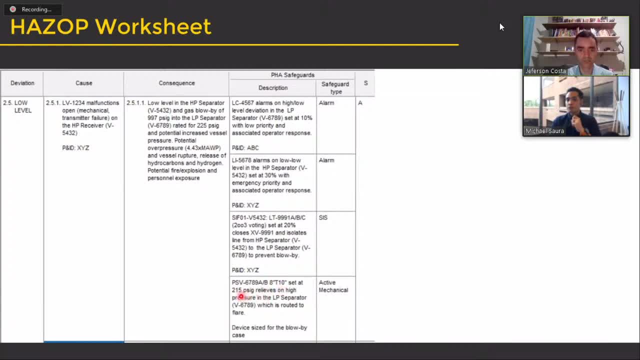 here in this scenario set at 215 PSIG. So it means that once the pressure downstream has detected 215 PSIG, it will relieve on high, high pressure, which is rather to flare to prevent the blow by case. So it is sized for a blow by case. 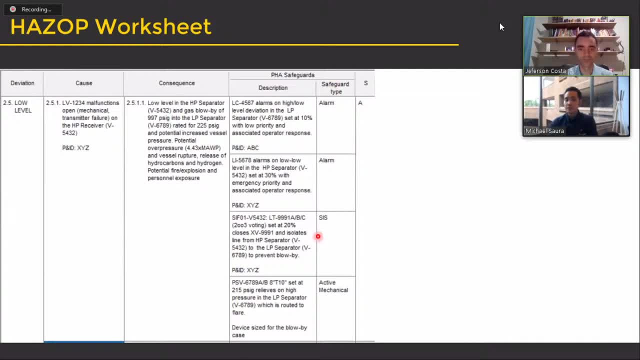 And so understanding what these are. now, the team felt that the likelihood of this would be a one which is, for them, the lowest lowest likelihood and therefore the risk is medium, And for this company, for example, they, their medium risk is considered a LARP. 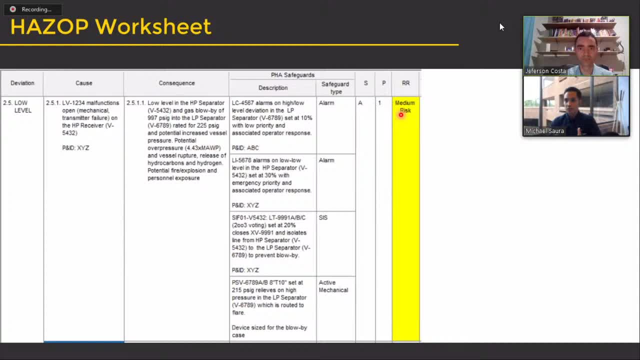 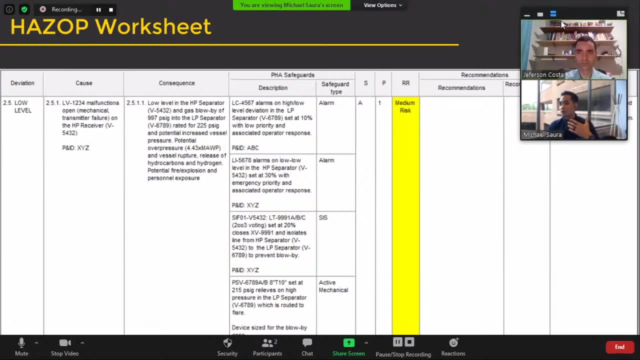 as low as reasonably practicable, And so they can decide to keep it as is and not do anything. They considered it as low as reasonably possible, or they can do further analysis, So this team decided that they want to review this in LOPA. 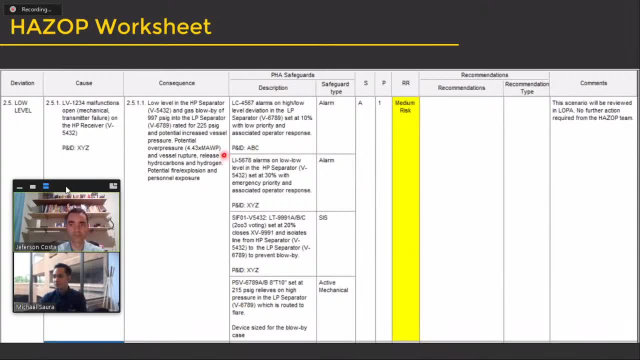 no further action required for the HAZOP team. So that is one example And, like Jeff was saying, this is just one scenario. So you'll have to do this for all nodes and for all other, all possible low level deviations in that one node. 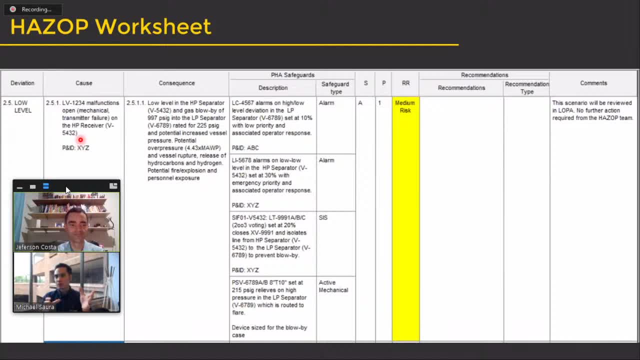 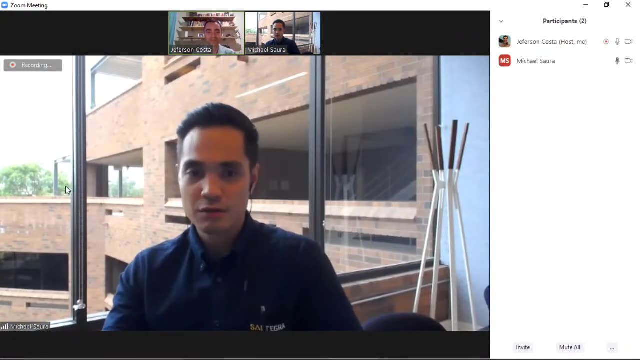 And this node is from the high pressure separator, through the low pressure separator and feeding into the fractionation or distillation column somewhere downstream. So hopefully that's a good example, Jeff, to go through, and hopefully, if the people have questions, I'm happy to answer later. 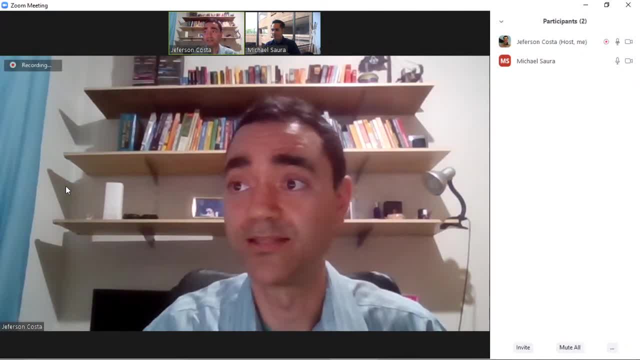 Not yet. they don't have a question not yet. Yeah, later. And guys, if you have a question, If you have any questions, please let. you can let in the chat and I may address that to Michael if it concerns to our subject here. 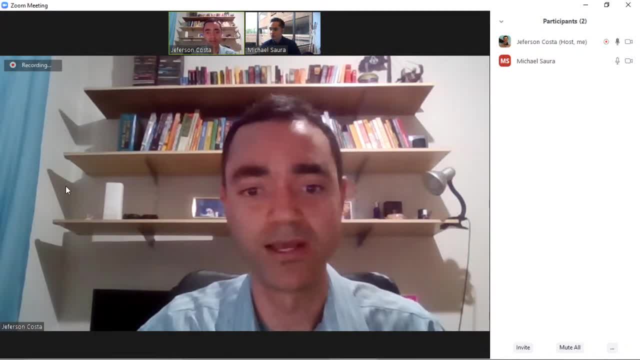 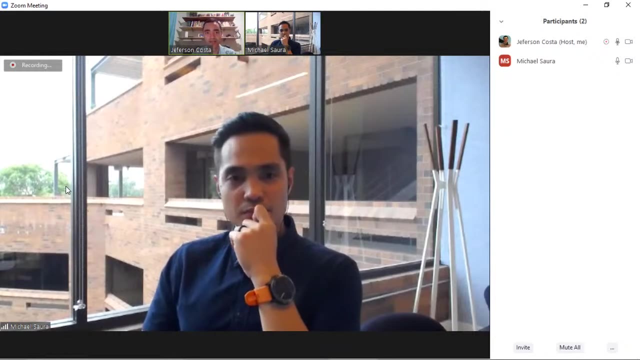 And Michael, I would like to ask you something. I saw that you have a control valve and a shutoff valve, and sometimes companies use the same valve to do the same both functions: safety and control. How is it? It is a question of regulation. 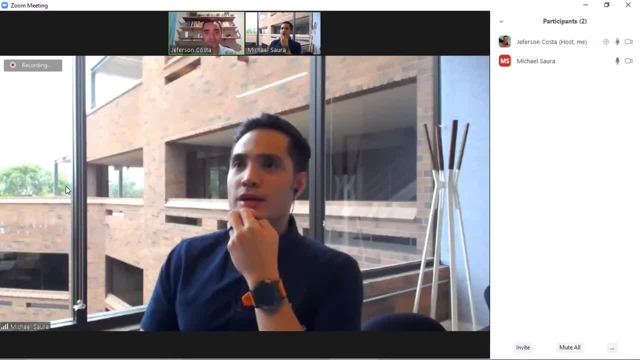 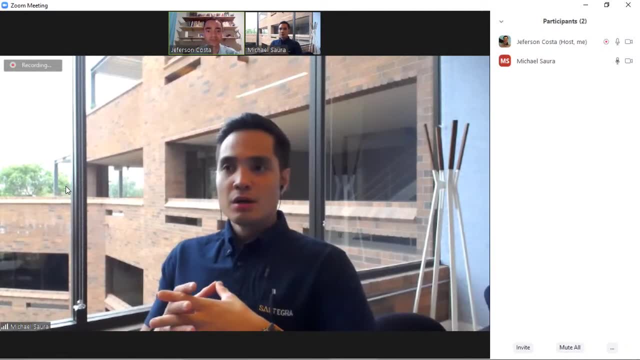 What do you think about that? So I can't speak of regulation outside of the United States because I only know so much. So, in terms of regulatory requirement outside of the US, some companies might be requiring some regulations, might be requiring that they need to be separate. 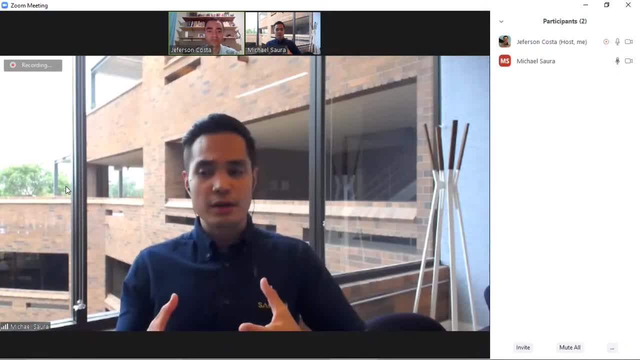 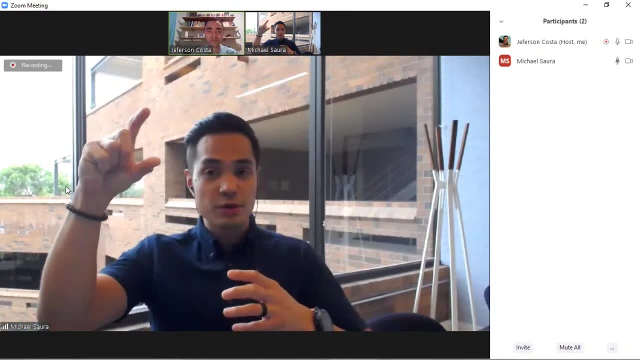 But in terms of There's been a lot of, There's been a lot of, There's been a lot of talk about that, but typically because the final element is being shared, even if the transmitter and maybe the logic solver is separate, right. 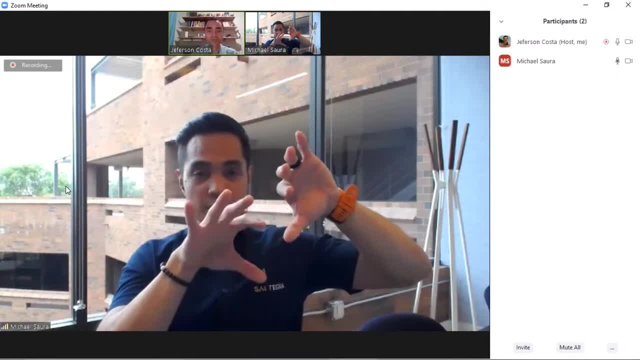 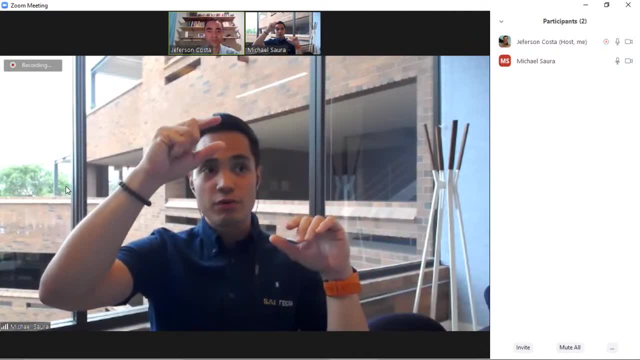 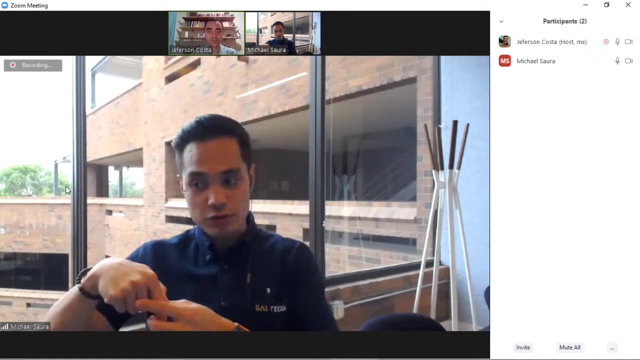 So let's say the BPCS is. you know, BPCS and the control valve is one loop, and then you have a separate transmitter for the shutdown function and a separate logic solver and even a solenoid valve that will force close the control valve. 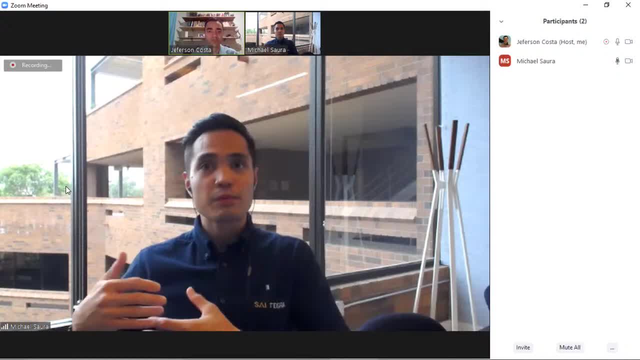 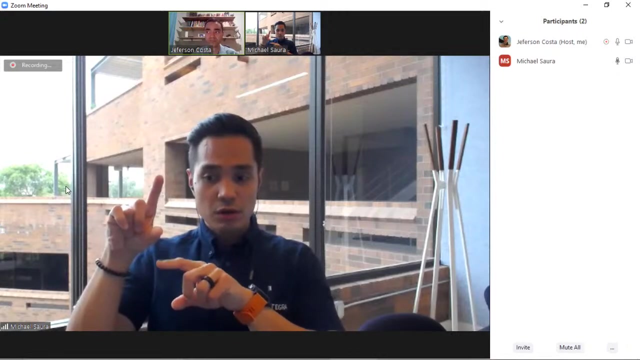 That's another loop. So I have seen it where some companies would allow those two to be considered two independent entities so long as they can get a calculation of the shutdown loop. If you can confirm and verify that that has, even if it's sharing the final element, if there's no common mode of failure, even though it's just one valve- and I know this is hard to picture- 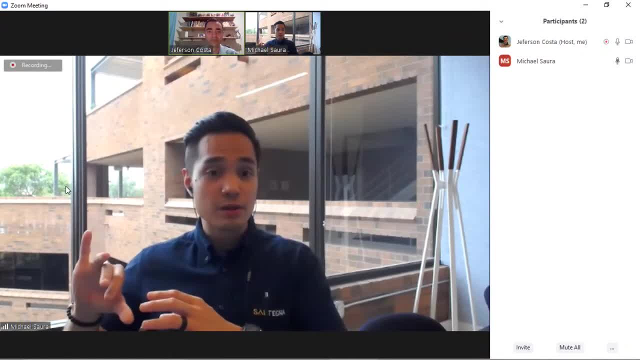 I have seen it where they qualify that as an independent entity or an IPL from the BPCS system. But in best practice you would want, let's say, it's a new plant. I wouldn't try to do that. I would try to install a separate shutdown isolation valve that is separate from the BPCS. 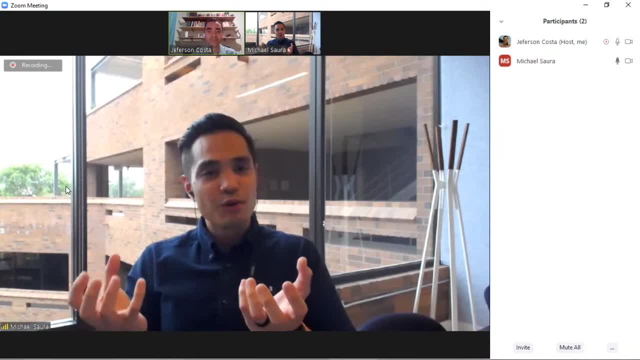 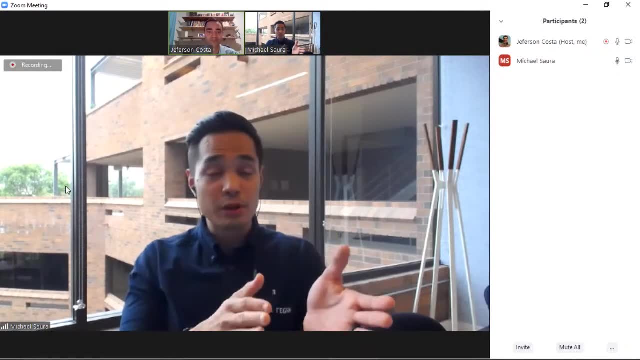 It's just safer. that way, You have no common mode of, There's no common mode of failure and there's no complications with the calculation of the PFD or the RF, which is probability of failure on demand, or the risk reduction factor, which is, again a fact. 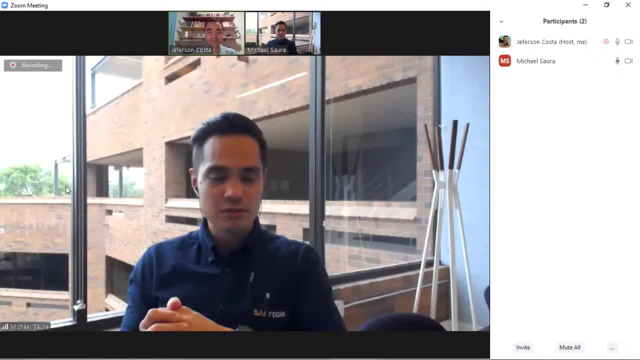 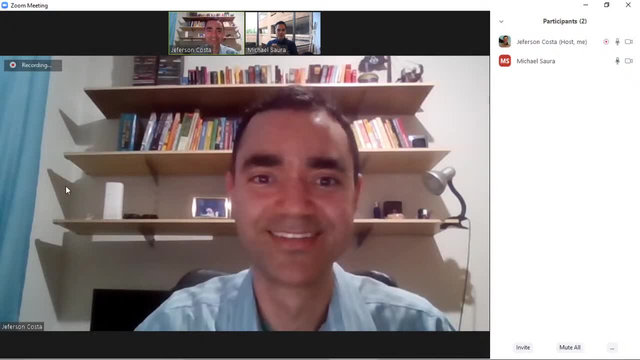 These are terminologies for safety instrument systems. But yeah, that's a good question, Jack. Okay, So you say you've seen that as well in your experience? Yes, I am from a separation right And I have experience with hydrocarbons. 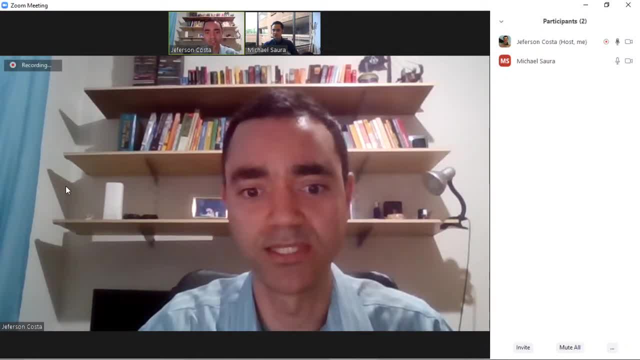 Hydrocarbons, petrochemical industry and I have seen that they were more addressed to use safety separated from control. So in the safety it would go to the PLC and the control to SDCD, But in air separation we do everything at just one PLC. 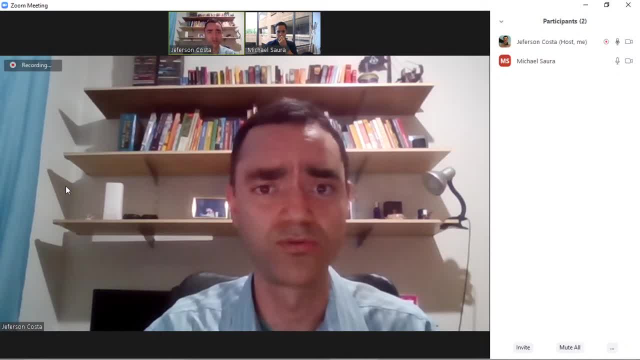 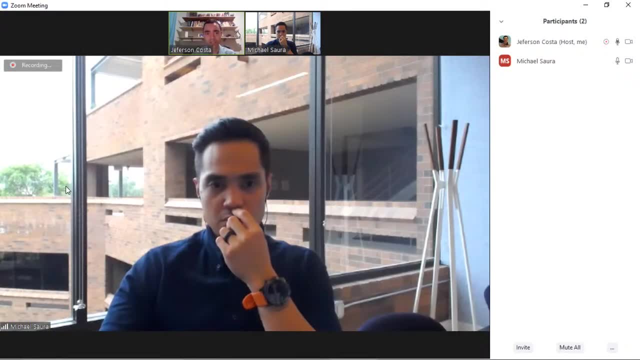 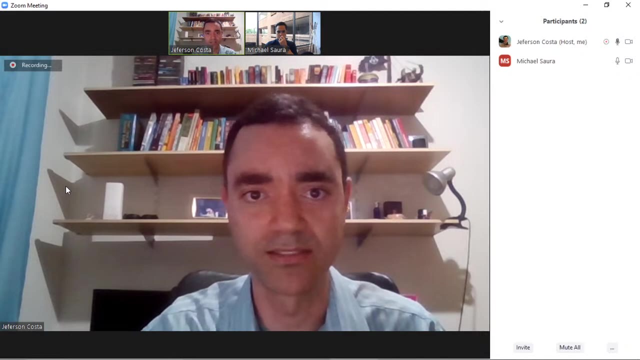 So everything is together. It's not so common to separate safety and control Only when we have some specific issues of something like leaking or something oxygen leaking and something like that and nitrogen leaking. But usually we only have one valve to everything. 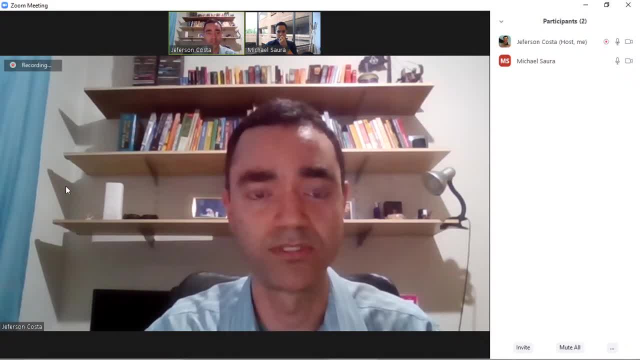 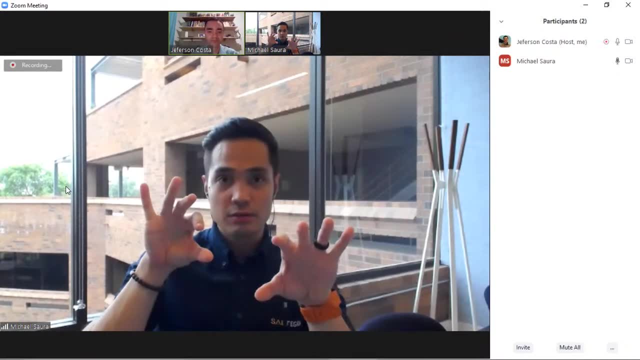 And we consider that the alarm, the shutdown and something like that Mm-hmm. But I would want to say that just to clarify that consideration for sharing the same loop is mostly allowable in the sense of talking about layers of protection analysis. 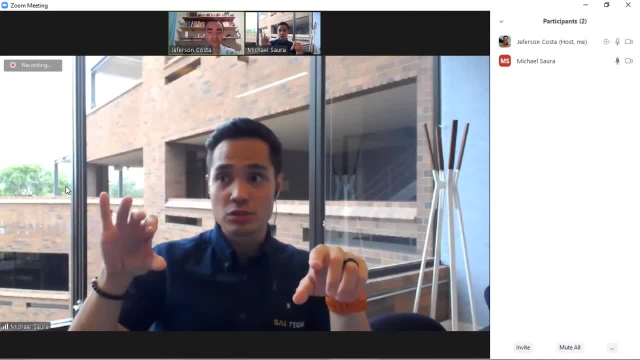 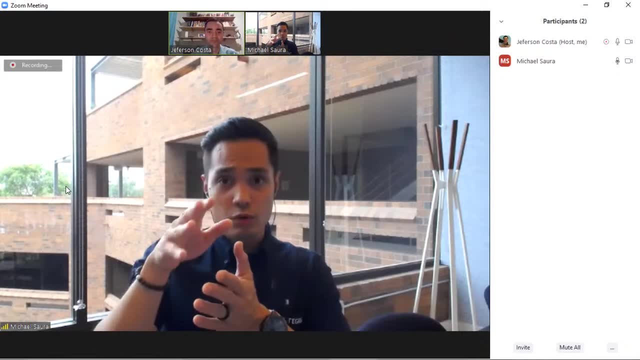 But in IEC 61511, which is the standard for functional safety. if you want to consider that loop as a safety instrument of function, then you should be separating the final element as a requirement of 61511.. If you want to comply with that standard, then it has to be separate. 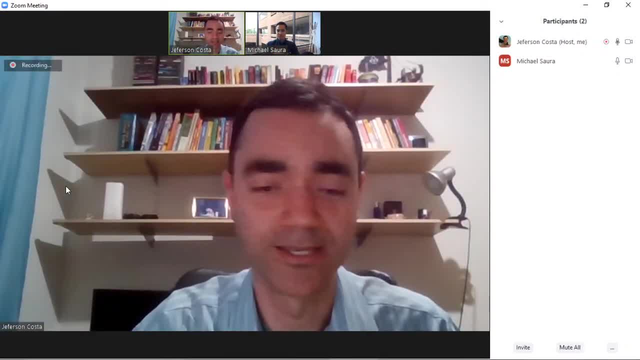 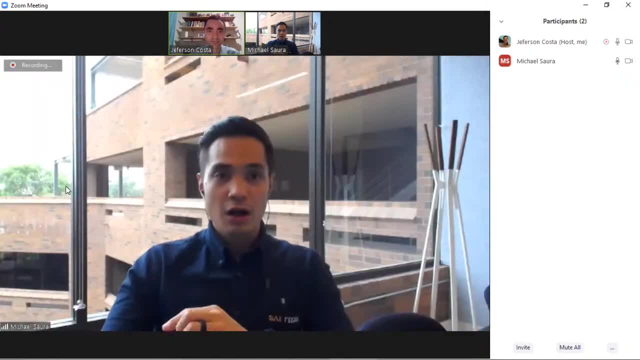 Okay, I have a question here. You will talk and show an example of seal calculation. No, not today. It's a very detailed discussion. It will take more than an hour, So you just have to understand the concepts first before you start diving into seal calculation. 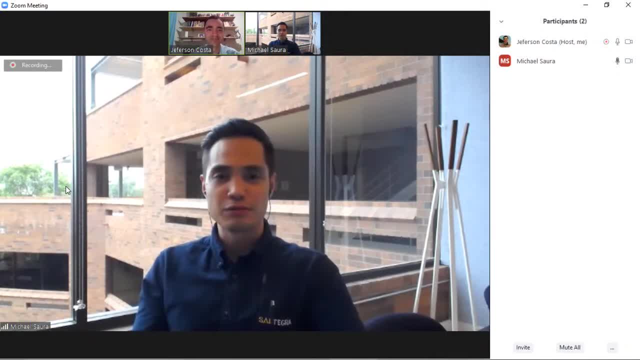 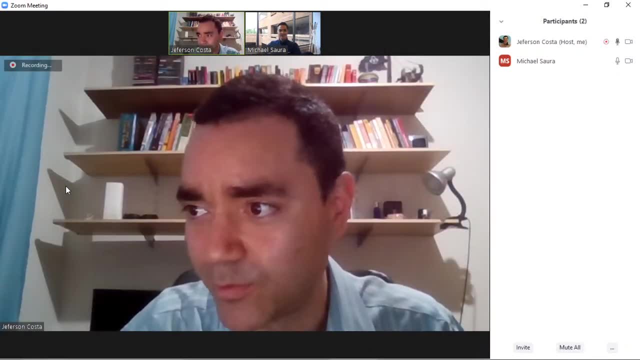 And I'm happy to probably work with Jeff here later on to get that in part of the segment, But not today. Okay, No problem, But I will read the question and let's see what kind of guidance you can give to Tamer. 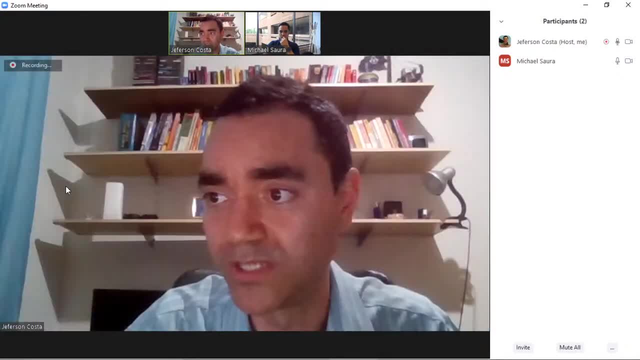 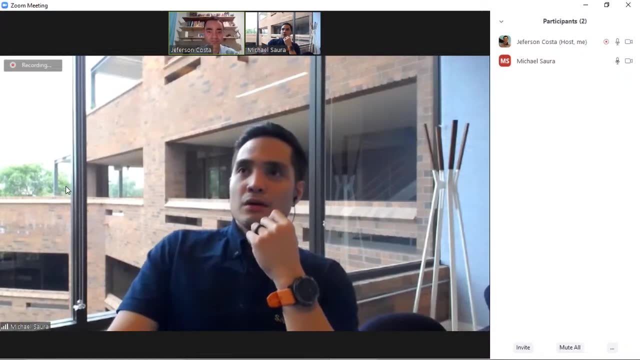 Sure, What are the ways to evaluate the consequences in a quantitative way? What are the methods used to quantitative Sure? So HAZOP is qualitative. You've probably heard of layer protection analysis And I would say that my first go-to quantitative way is layer protection analysis. 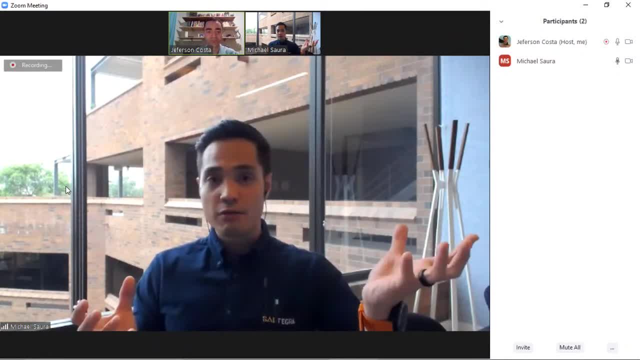 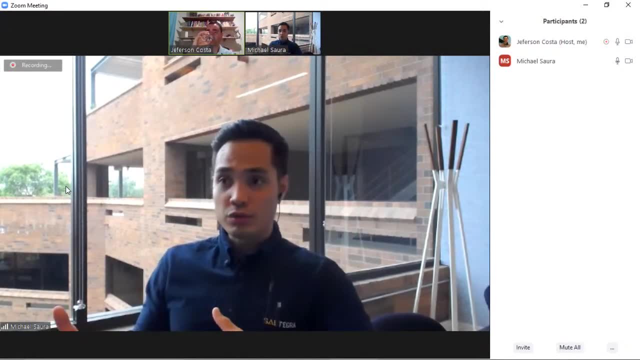 It's very easy to get into, especially if you already have your HAZOP completed. It's easy to transition from HAZOP to LOPA. It uses a set of rules that are already widely used, you know, in terms of the initiating, consequences, cause, frequencies, et cetera. 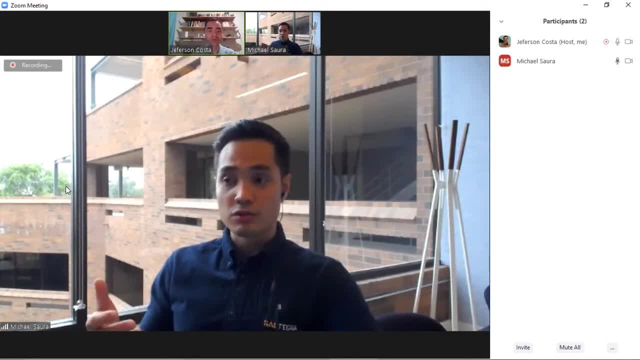 It's a very good quantitative way of identifying and understanding your risk. If you want to even go deeper, you can use other quantitative risk analysis techniques. You can do fault tree analysis as well, or event tree analysis. So those are going past LOPA. 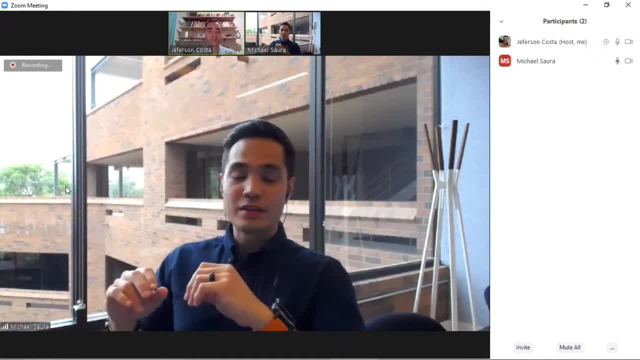 And LOPA, a lot of people will say, is semi-progressive And LOPA is quantitative, but it still uses numbers, It's using a set of rules, So to me it's still considered a quantitative methodology in terms of risk analysis. 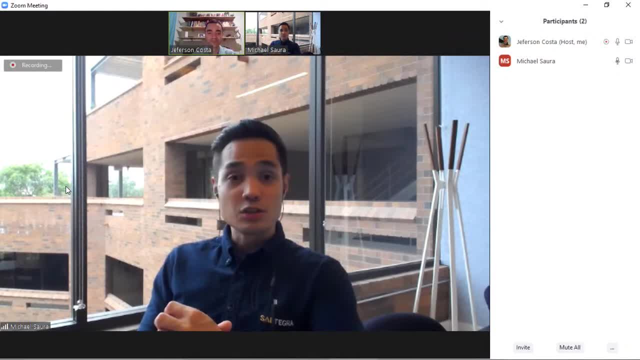 So that's something I would get started with that, And I can send you references. Actually, we will talk about that later, but I can send you, or anyone who's interested, references as to where to look in terms of these subjects. I'll be happy to provide information. 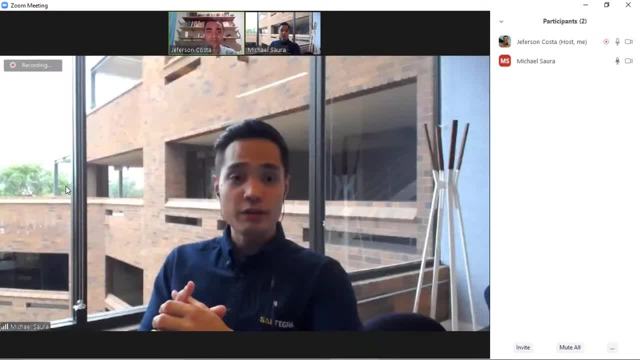 Do you have an example from LOPA? I don't have an example for LOPA- yes, I didn't have time for that- But I can talk about it. like I said a little bit, but not an example today, just because of time. 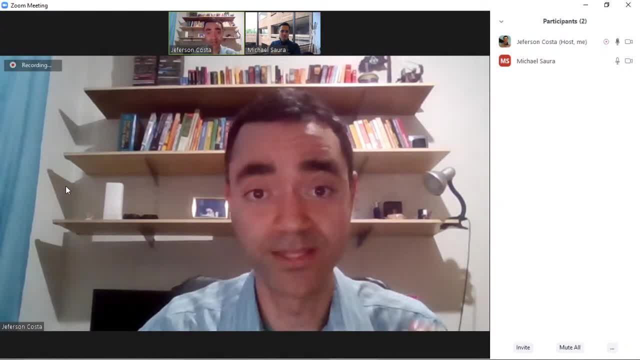 Okay, no problem, my friend, No problem. Our intention here, guys, is to introduce you to this subject because it is very, very important, And I have been working in companies that safety is a question of employability, So it's. 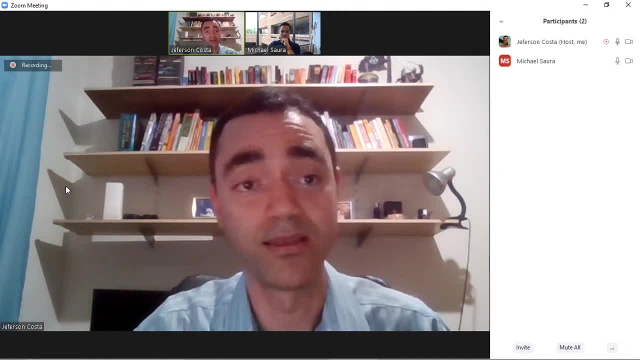 If you do something wrong and nothing happens, eventually people will not worry about that. But if you do something wrong and something wrong happens, if there is an incident, accident, injuries, sometimes it's like burning witches in the Middle Age. Okay, so you must take care a lot about that, not because of your job, but you must go safe to your home every day. 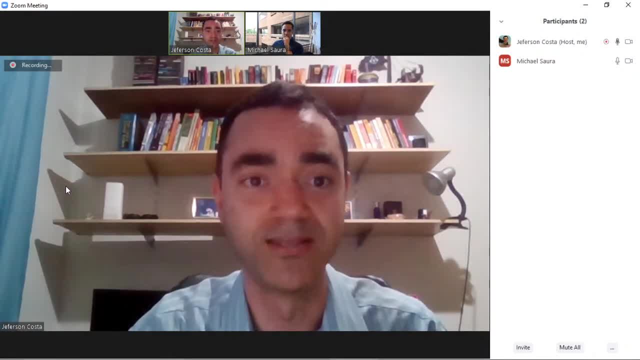 Okay. So you must take care a lot about that, not because of your job, but you must go safe to your home every day, And that is the way that it should be, Do you agree? I 100% agree, Okay. 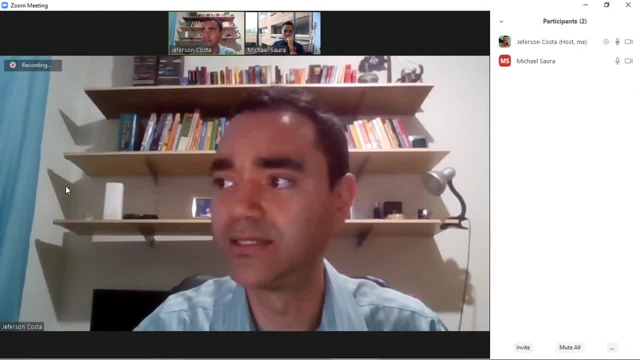 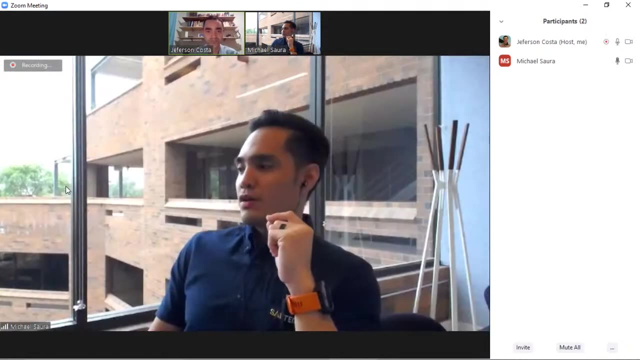 And what are the tools and softwares that are used in this kind of activities like Hazopi, SEAL and Lopa? Or is just the spreadsheet enough? What do you think? No, So I am not sponsored by any of these companies. 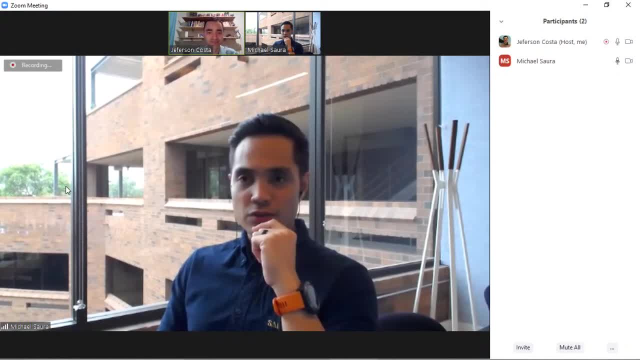 And it's just that Because I use them. But there are softwares such as PHA, Pro, PHA Works are at least the top ones that we use here in the United States. I'm sure there are other software out there. But PHA Pro and PHA Works are the most used, at least in my field, in what I see in oil and gas and in pharma and chemical manufacturing. So those are two great softwares. Very, very robust- You can do a lot of programming in it to make things easier for you- and a lot of reporting capabilities. 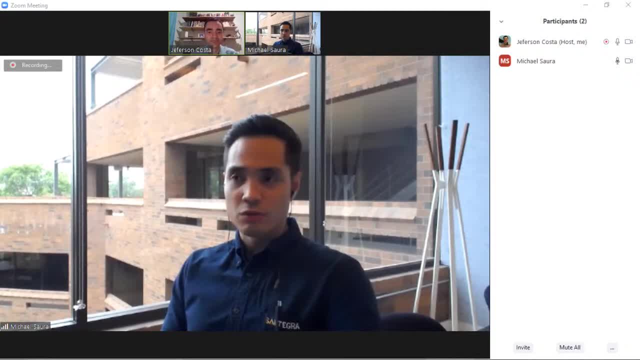 So, like I said, I'm happy to share some information about those. If you want to reach out to me, just reach out. And in terms of one of the newer software that we are actually using is called Bowtie XP And I know I didn't talk about Bowtie in, you know, talking about hazard identification. 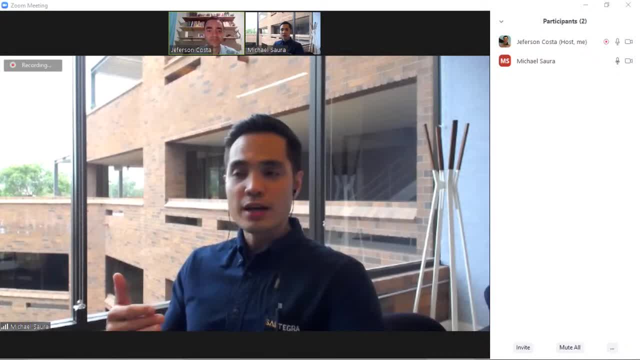 And risk analysis. But Bowtie is actually an up-and-coming methodology. It's been used by a lot of companies for a long time now And it originated from Shell actually. But it's a visual. It's being the visual hazard. 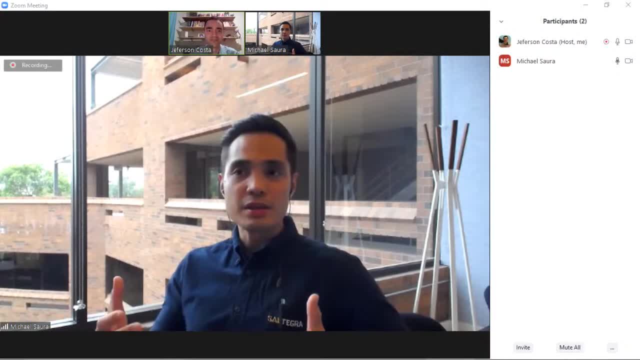 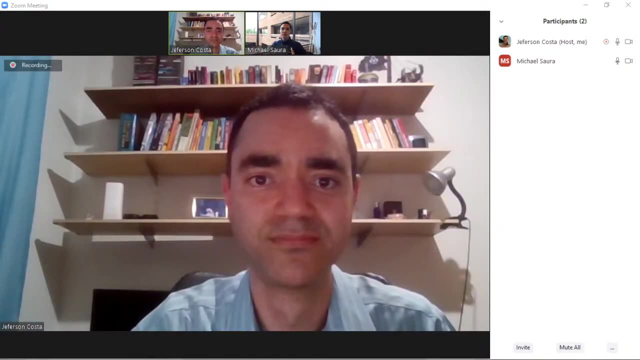 And it's basically a means of showing what your hazards are, What are the consequences Or what are the top events that can lead to certain consequences And what are the threats. So it's essentially a HAZUP, but more visual, And you usually use it once you've already identified your hazards. 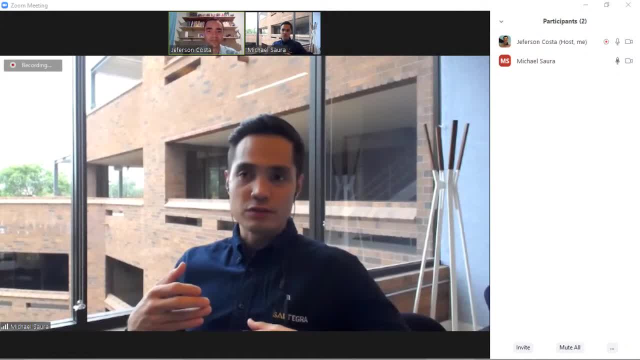 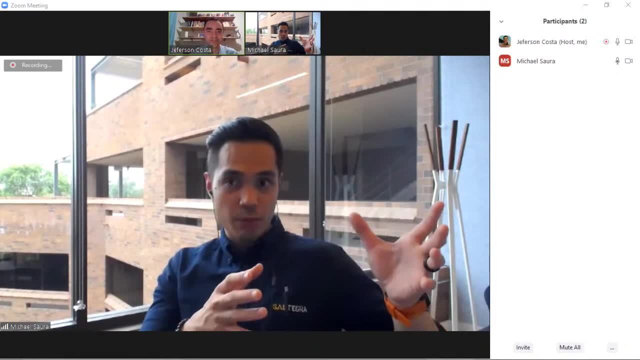 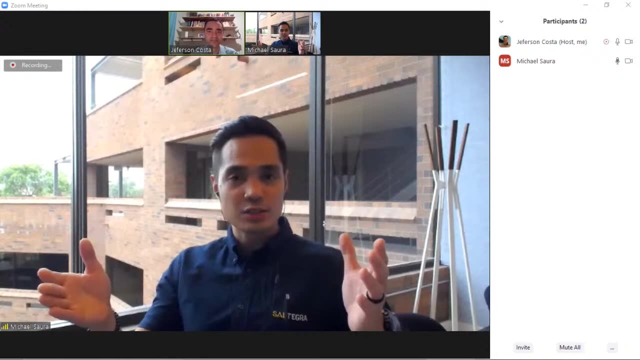 So Bowtie XP: it's another awesome tool If you want to represent your hazards or your scenarios from your HAZUP or LOPA into a more visual representation. Bowtie and Bowtie XP as a software is a great tool. It's a great way of doing it. 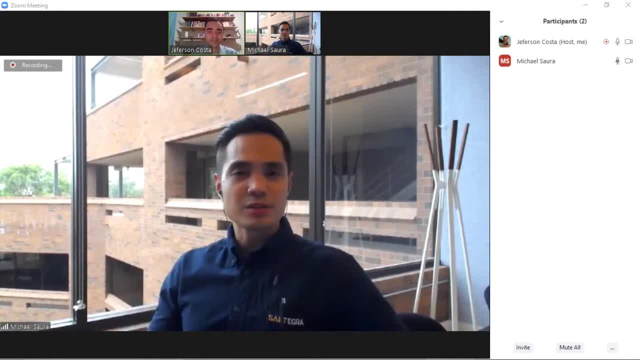 And I think, Jeff, I'd love to talk about that a little bit more when we possibly do a round two of this. I think if people want that, if they vote to do that, I'd definitely love to go back and do a deep dive on certain topics, if the crowd wants it. 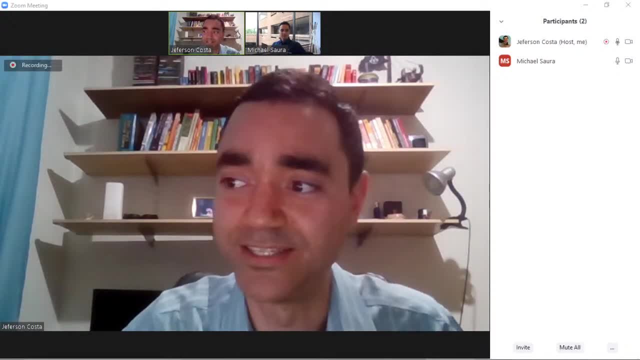 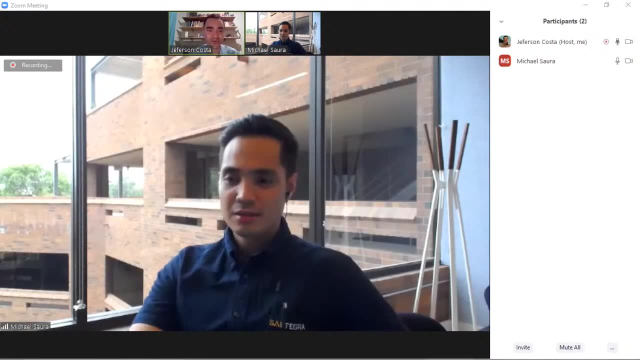 Michael Tamer is very, very interested in this subject. He has another question And guys, thanks a lot for the questions. Sure, sure, I'm pretty sure that Michael will like to answer this one, And probably you already heard about this. 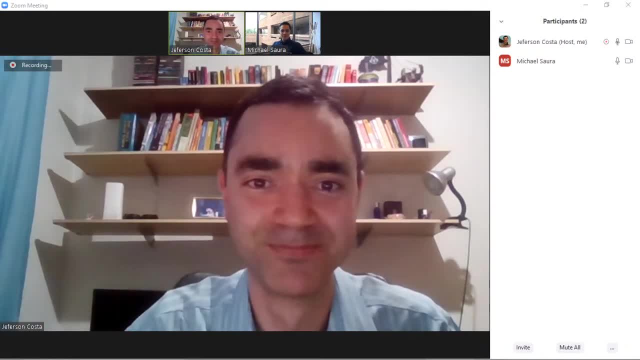 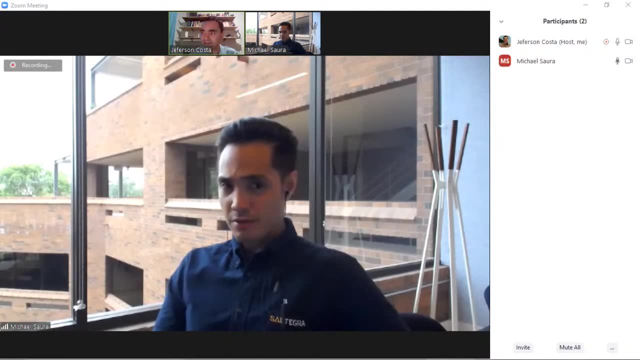 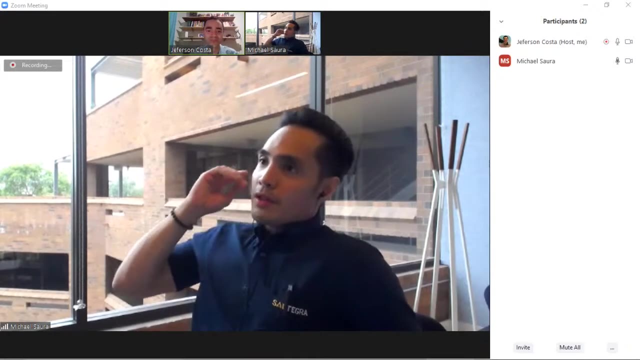 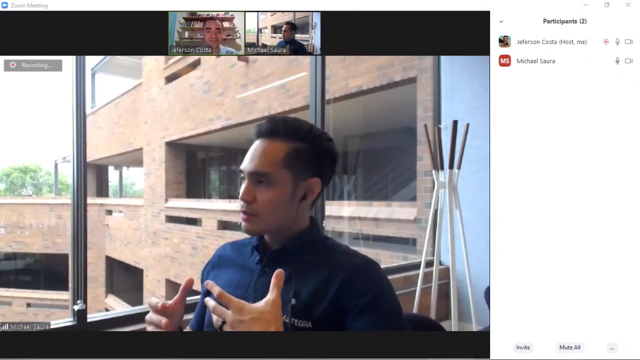 When use if-else and when use HAZUP. I think when he means if-else, he probably means what-if. So what-if analysis? yes, Okay, okay, Good question. So that's a good question Again. usually HAZUP you would want to use in plants that are continuous. 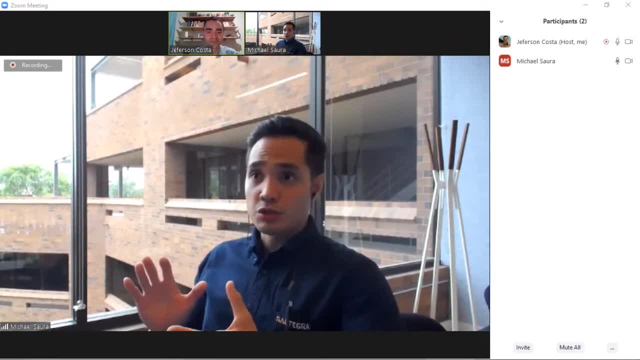 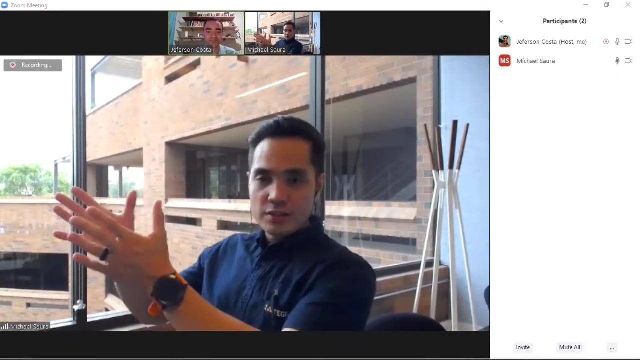 Continuous, Continuous processes. I'm not saying that HAZUP should not be used in batch processes, But sometimes what-if is more suitable to certain types of operation, especially for batch processes. I've seen more robust way of brainstorming, Because HAZUP is structured and it's designed for you know, when your process is operating in its normal condition, what can go wrong. right. 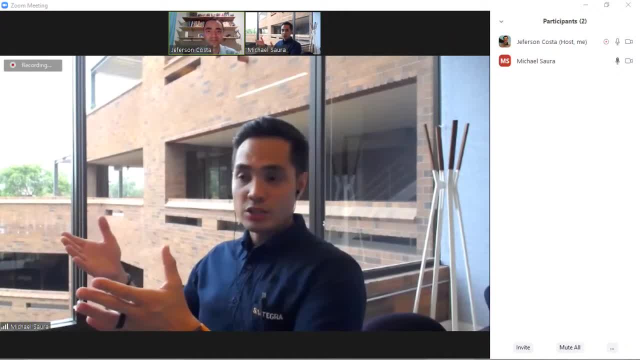 But sometimes you have batch operation, or what we call transient operation, where that's actually where a lot of the incidents had happened, Where things that are not written in a procedure. they have to do it, maybe once every five years, once every ten years. 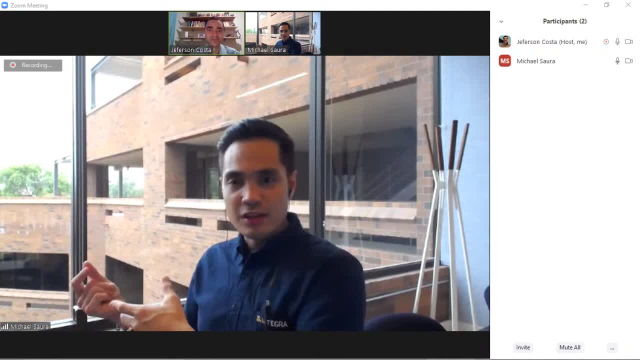 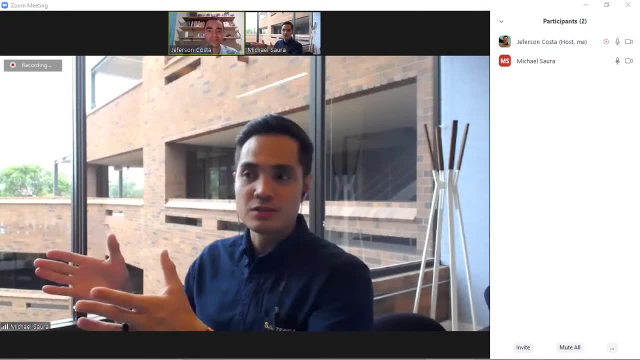 No procedure, no training whatsoever, And then the incident happened. Those are actually good processes or operations that you want to do, But what-if? And what I've seen is, for example, they'll go through the steps of the procedure and try to deviate from those steps. 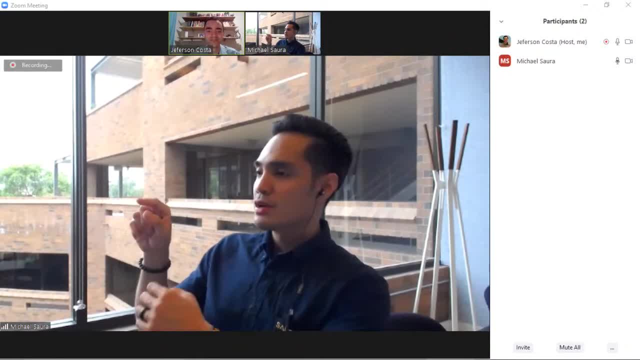 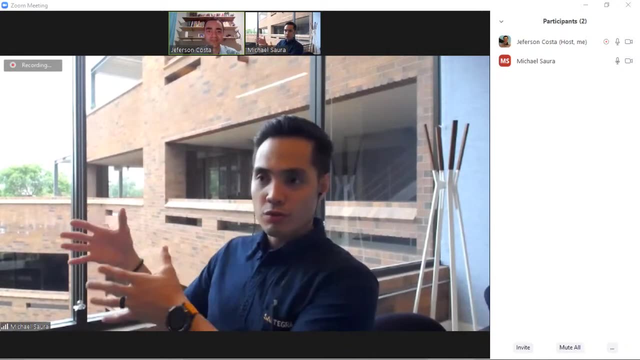 So, for example, if we're talking about, I have to set this control flow control into my- you know my- reactor at with a fill rate of 50 gallons per minute right into the reactor. So it has to be a controlled flow into the reactor to support the reaction. 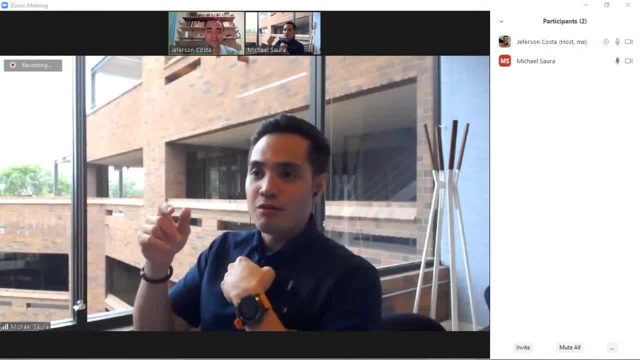 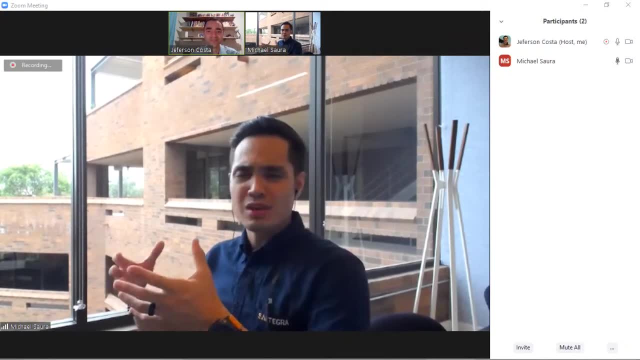 But what if the operator failed and inputted 100 gallons per minute. So that's a what-if. In a HAZUP you can do that, but it's just more fluid to do it in a what-if. So that's usually one way of using what-if. 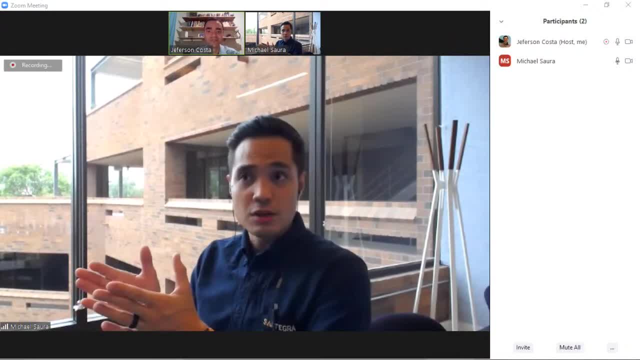 Now what we do here in our practice is we actually combine HAZUP and what-if. Nowadays you'd see that combined, because sometimes you address some small batches. So you would do some batch operation that you do in a certain plant And so you would do some what-ifs as well. that is not correlated to the guide words in HAZUP, if that makes sense. 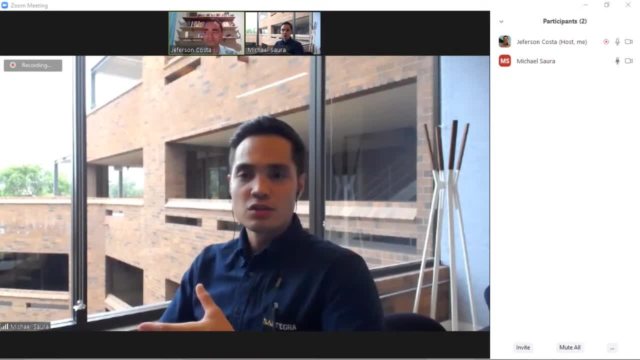 So but definitely a lot of use. I find a lot of use for it in smaller plants in batch operations. you know companies who aren't maybe like a plant that you can do a PHA for five hours or four hours. Usually a what-if will be faster for those types of plants. 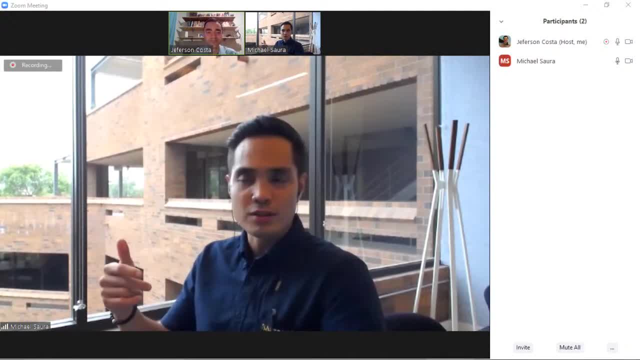 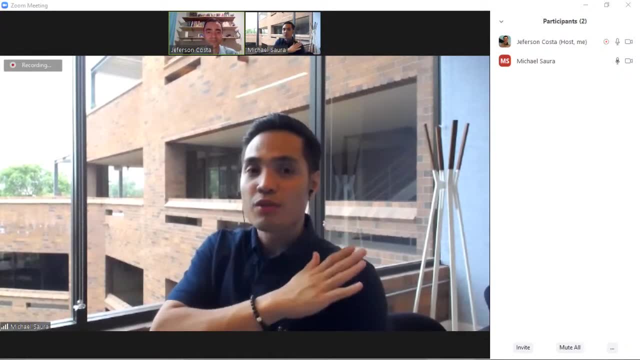 So as long as people are contributing with a brainstorming process, so long as the facilitator has prepared well and tried to understand what the hazards are by talking to people doing their research, checking their previous notes from the similar HAZUP, you should be okay with a what-if there. 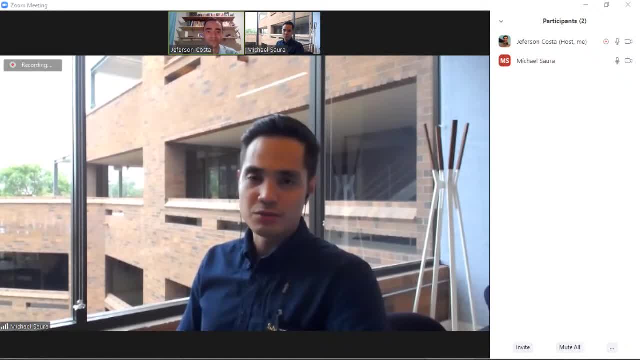 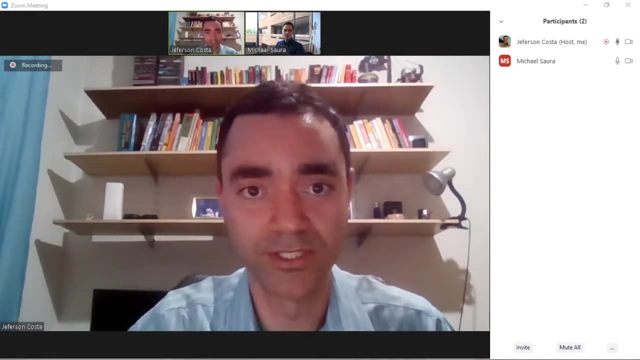 But my go-to is again usually HAZUP studies, just because it's more structured, It's cleaner and you know that you're hitting all the items that you need to address. Okay, okay, And you are a mechanical engineer and you said that you need to work a lot to get chemical engineering concepts. 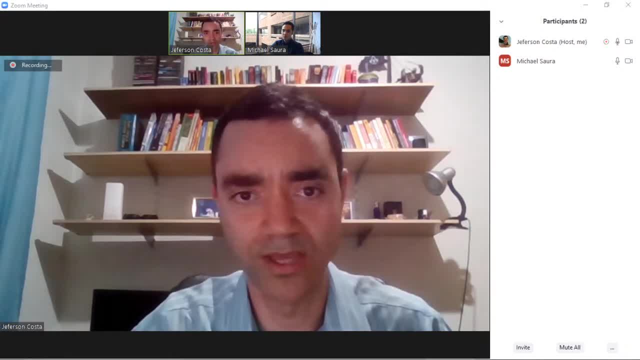 And when you face now you have a lot of experience, so you are familiar with a lot of scenarios. But let's suppose that You are facing a new process and how is your relationship, or the consultancy relationship, HAZUP leader with the chemical process engineer? 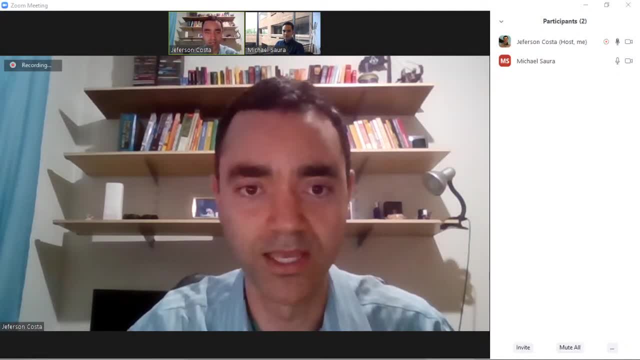 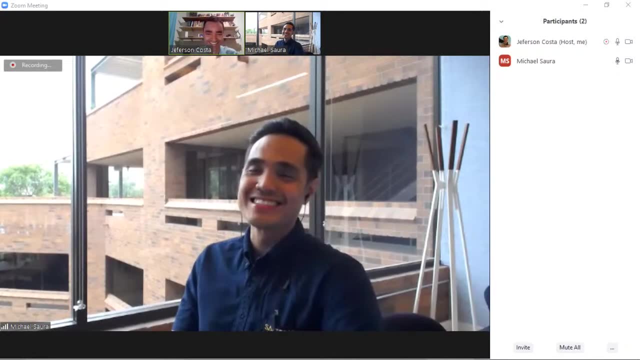 How the process engineer can help you and how they can let your work harder. They can make your work harder or easier. I would say that your process engineer or chemical engineering representative in a HAZUP are your best friends. You should make them your best friends if you're a facilitator. 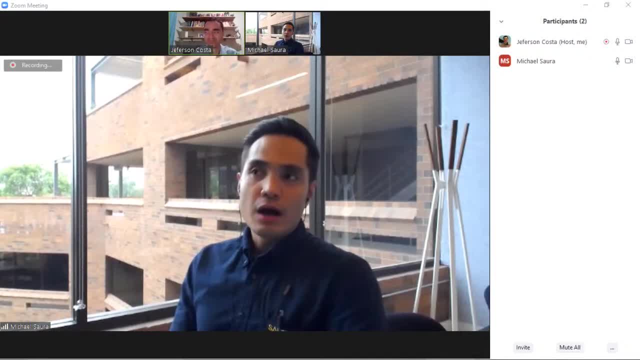 But in all seriousness, I try to do a pre-HAZUP meeting as much as I can before I go into the actual session. Why is this important To me? even if I already know the process, even if I already know the operations and what can go on that type of process, I still don't know everything. 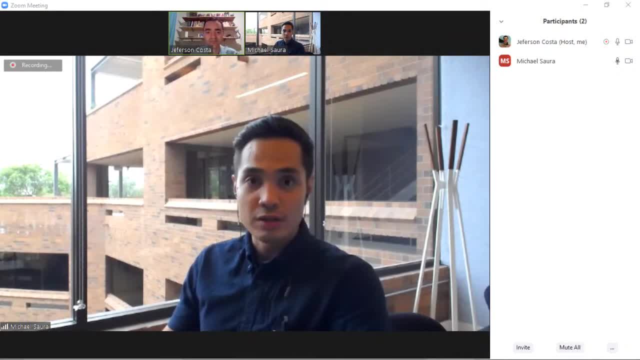 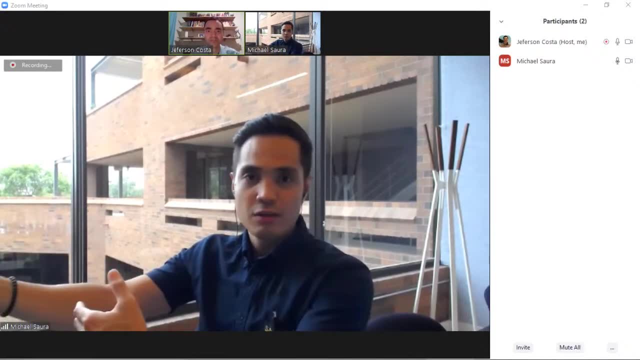 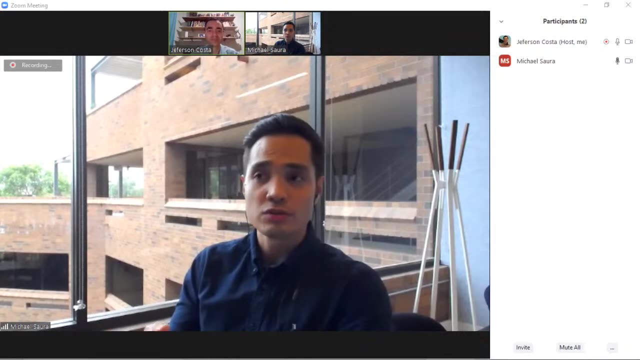 And also the process conditions are different. every plant. even if it's an identical technology, identical type of system, it can be operated differently from plant to plant. So I would go talk to the process engineer and maybe some of their operators to try to understand. hey, so let's talk about your process, let's talk about your plant, to help me understand what the process conditions are. 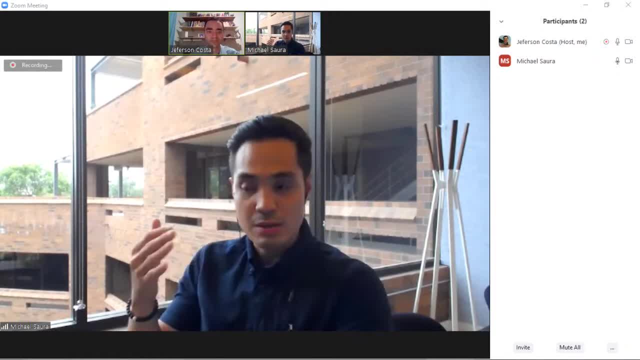 So I can maybe do a pre-evaluation Already as part of my preparation. And then also I would already try to get them to do some of the process safety calculations. And I know I'm throwing a lot of jargon here, but process safety calculations are usually like: how fast will my vessel fill up if I were to block the liquid outlet? 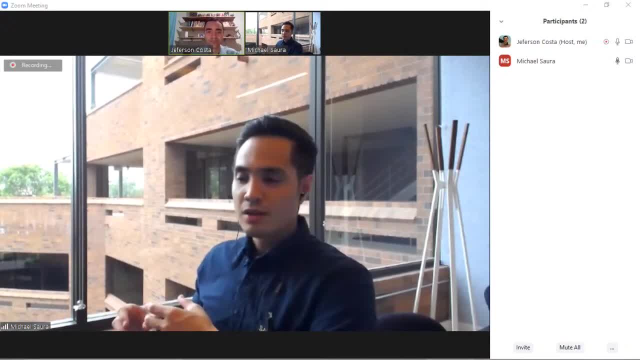 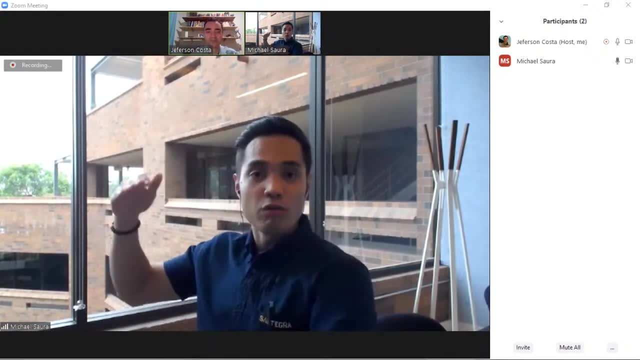 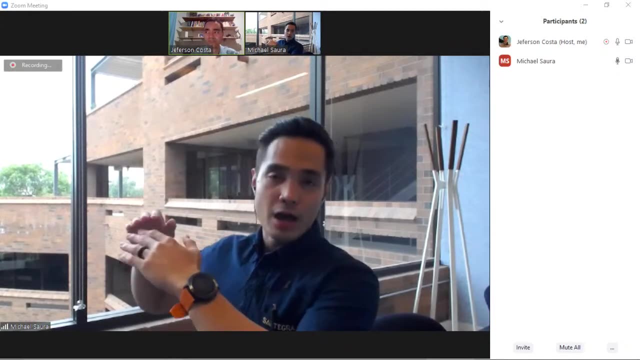 For example, if we're talking about a crew tower right, If I block the bottom valve control valve, if that closes, How fast will level build up until I overfill? That's typically a process safety calculation By the time you get the high level alarm or hi-hi, whichever the company wants to do- until you overfill it. 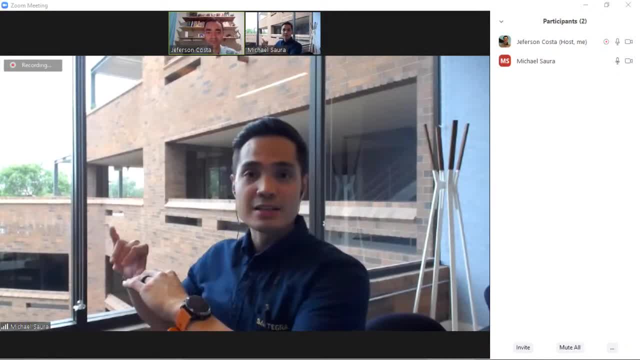 And it leads to a consequence of interest: how fast is that time So that I know where is my alarm sufficient? So there are cat ears that I need for my alarms to be considered sufficient in barriers or protection analysis. So I have them. do some of those scouts already. 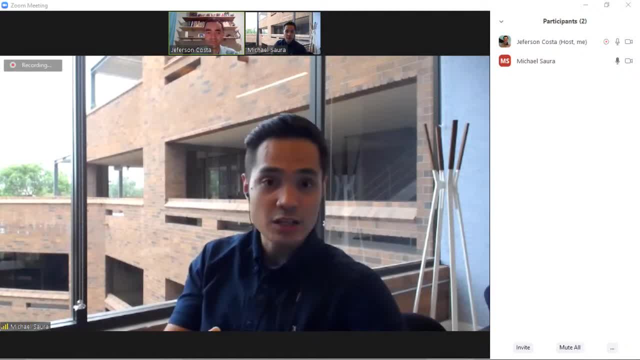 Some companies require the HADZUP team to do release scouts. So what are release scouts? Release scouts are basically how much material can I release if my pump seals were to break? and now I have leaking sour water with H2S of maybe 10,000 parts per million. 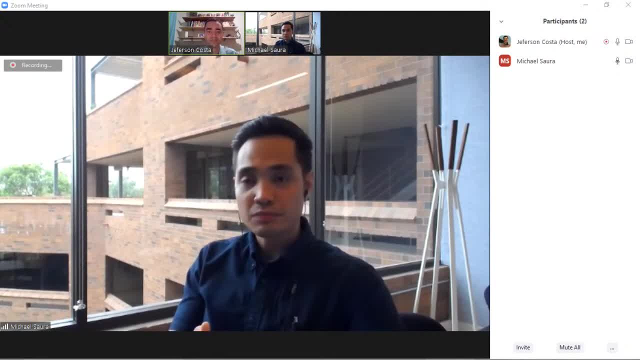 So the instruction there would be how much of those can impact people, and they would have to calculate that. So I would already ask the engineers ahead of time if we can do some pre-calcs, if they have time as well. So that's how my relationship is with them. 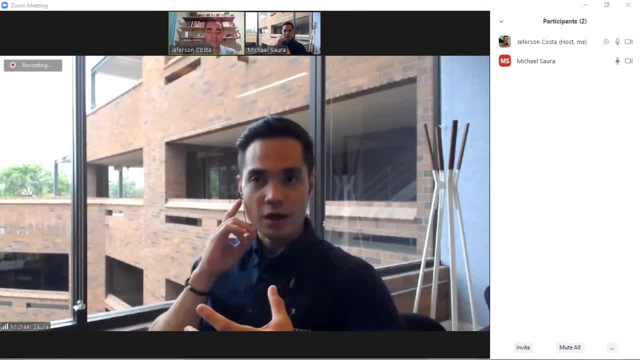 and we get to understand the process together, because I also tell them: hey, these are what we're looking for, These are the possible hazards, And then they'll tell me, and then I'll ask them: what else are we missing? So in this way, when we go to the HADZUP, we come prepared. 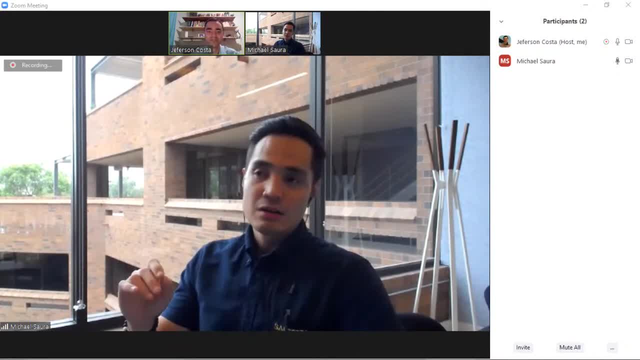 and it goes smoother. There's less interruptions because we have to park or put something aside. We have this system called a parking lot list, where you put the questions into that list so that the other people can address it right. So, for example, one of the parking lot would be: 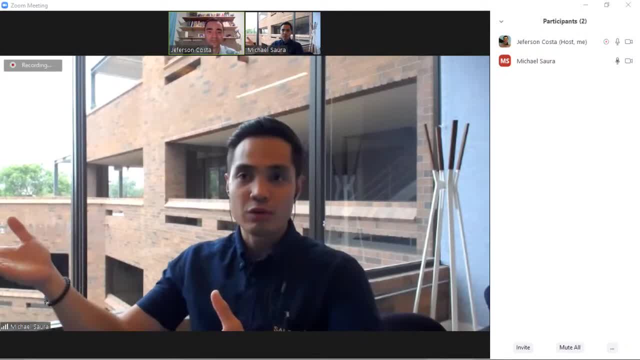 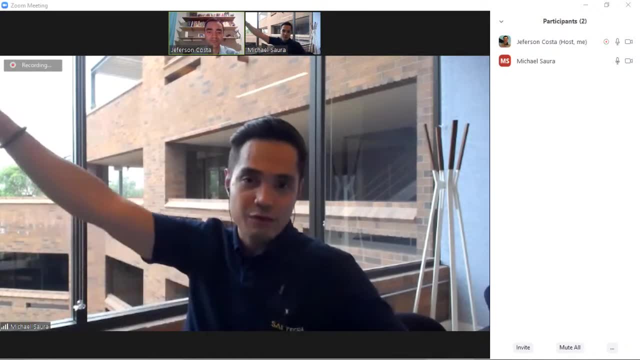 you know what is the set point of that relief valve? It's not listed on the P90.. It's not listed on my relief valve document for some reason. So someone would have to go on top of the tower and check what it is. 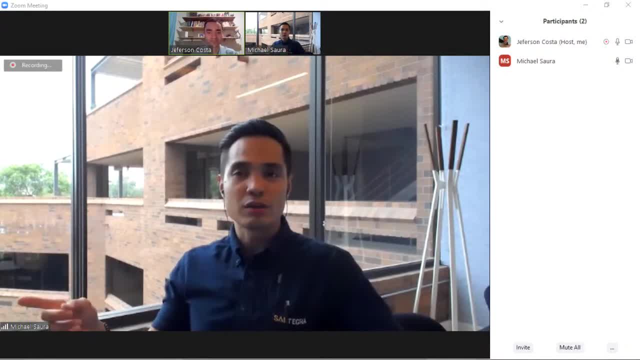 So it's better that way. We don't have to do that a lot. Instead of doing that later, we do some pre-work ahead of time as part of the prep. So that's my relationship with chemical engineers as a facilitator. But another thing is we also do audits. 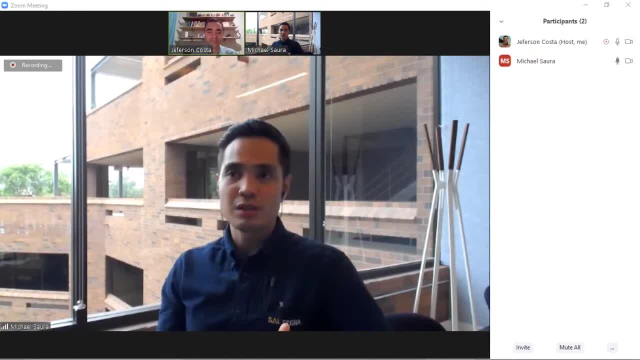 So when I do audits, process engineers would. usually it depends on how much involvement they have with the PSM program, but I would also interview them sometimes depending on who I need to talk to. But, if you know, they're involved in a lot of the PSM program. 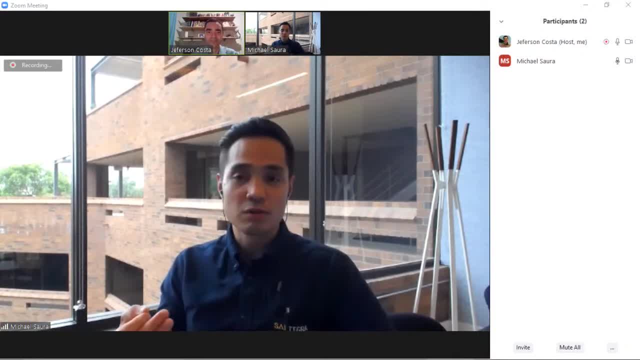 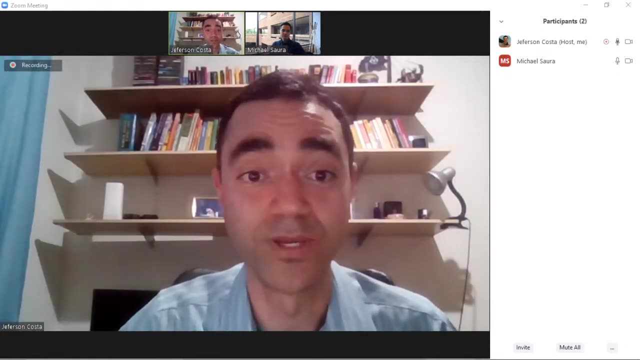 I would interview them and ask questions about certain or specific parts of the elements of their PSM program, But for the most part that's my interaction with chemical process engineers As a facilitator, as an auditor and as a consultant. Michael, we're going to the end of this live session. 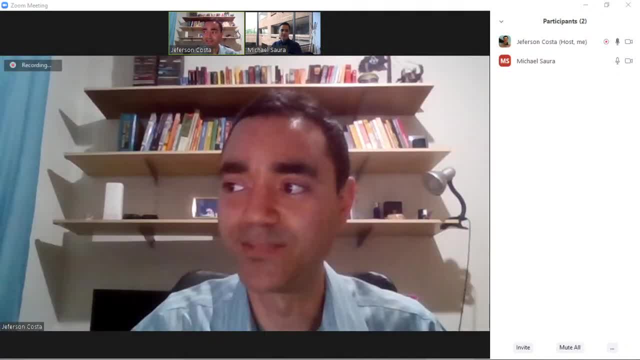 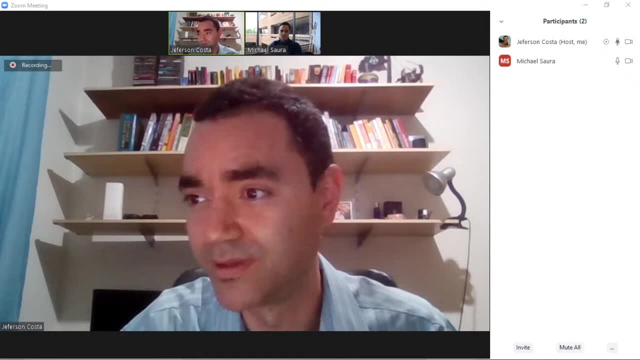 It is very, very nice to talk to you about this subject And let me ask you a question that it is in my preliminary questionnaire, but actually, oh my God, let me find it. Actually I have. what material should fresh graduate refers? 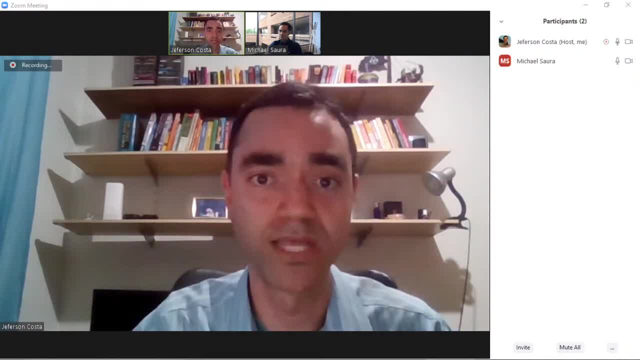 And I would like to add, if you want to get deeper in this subject and get eventually, want to start working with this, what they should do: References, websites, books and stuff like that. courses- I don't know if your company have course to offer. 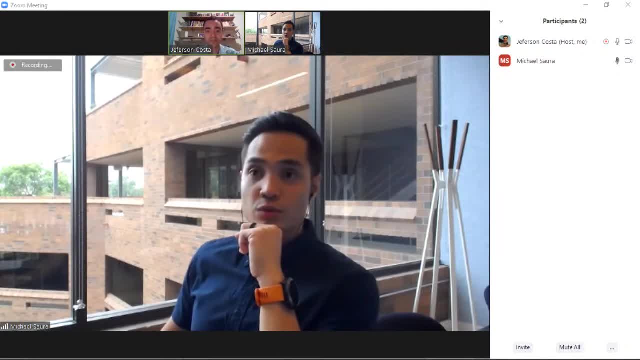 Yeah. so my first suggestion would be: there's a lot of free resources out there, but my go-to would be the CCPS Chemical Center for Processing, and they have a lot of free resources that they have. They have a lot of information. 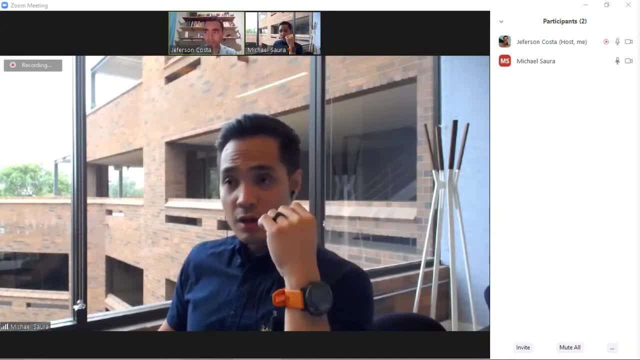 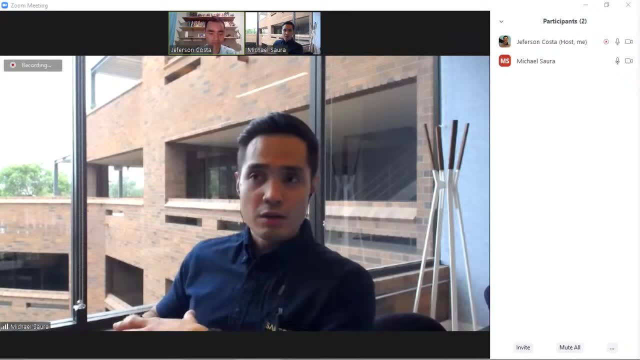 You can register there and you can also join as a member if you want, for a fee, but there's a lot of free resources that they have. They also have books that you can buy through the Kindle or Apple store. There's eBooks that you can buy or physical books that the CCPS had published. 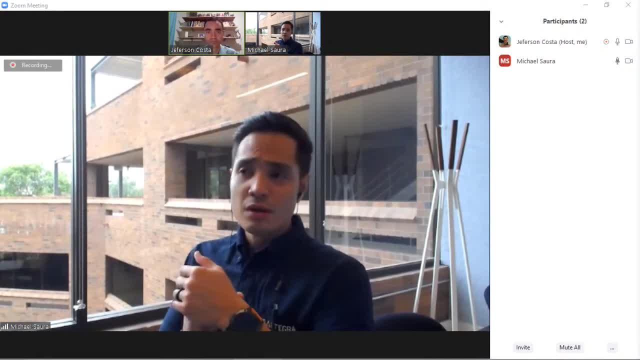 and a lot of good information about process safety, Risk management. also, a lot of they have developed books that are widely used all over the world now is the books for LOPA, or independent protection layers, and also conditional modifiers, et cetera. 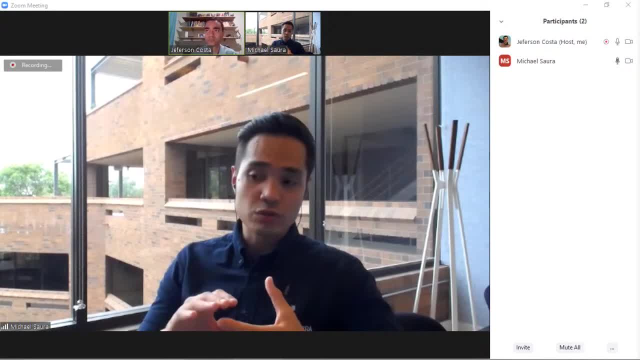 So a lot of CCPS books, I would say, are my go-to or my suggestion. ICAM-E is also a good resource in the UK, And then there are schools that are actually offering online courses for process safety, And so these are all neutral, non. 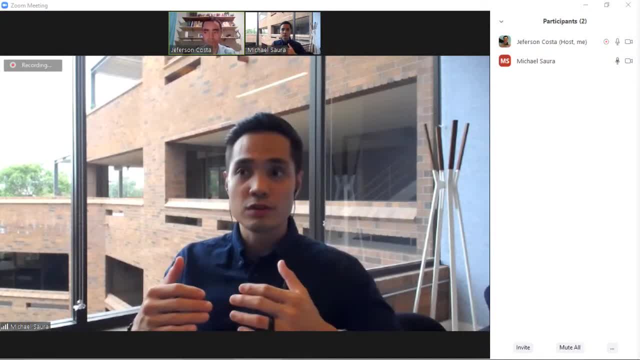 they aren't from a consulting firm, they are all neutral. So these are information that you can easily get to, some free, some. you have to pay for some of the courses. But, like I said, feel free to reach out to me. 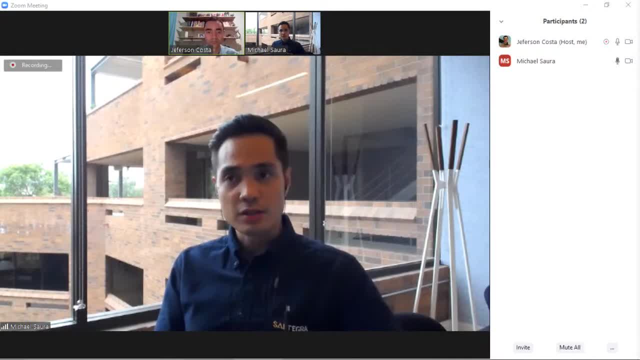 I've been mentoring some undergrads before. I've mentored some chemical engineers who wanted to get to get into process safety, So I've given them some of my insights And also I would suggest that you also reach out to other practitioners in the industry from LinkedIn. 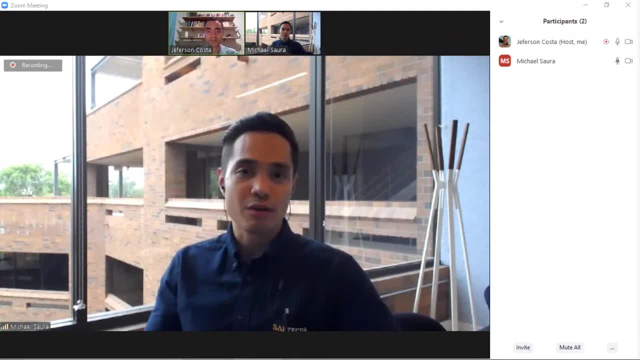 You'll be surprised as to how many people out there are willing to impart their experience and their knowledge to, just because we need more people here in this field. It's a field where not necessarily taught in school all the time It's a new subject or a new matter. 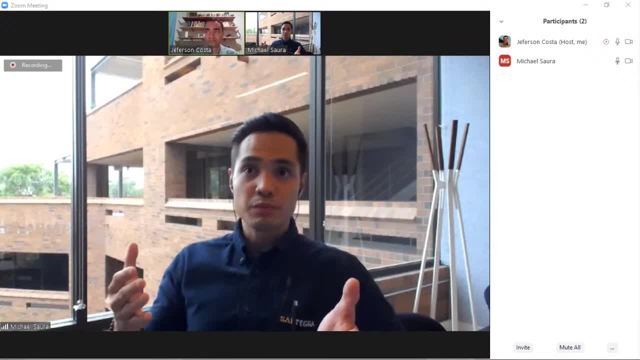 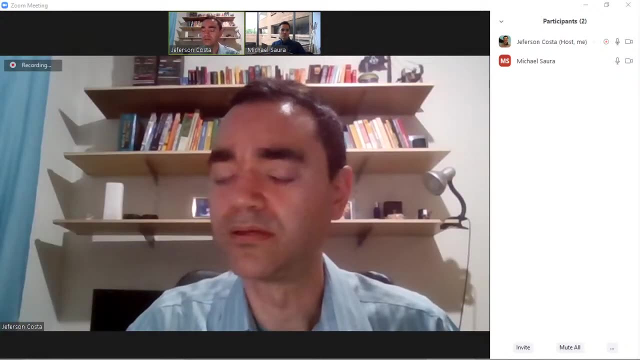 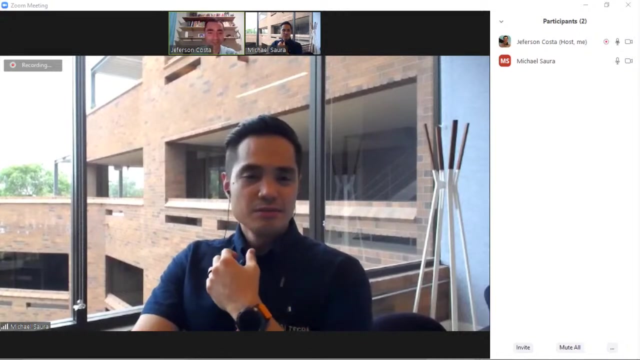 a new field where it's growing and people are more and more getting into, but still a lot of people can find the resources to know and understand about it, And I forgot what I will say to you. No worries, My friend, what are your plans to the future? 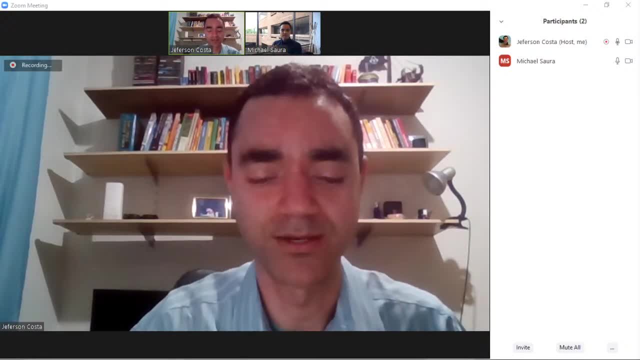 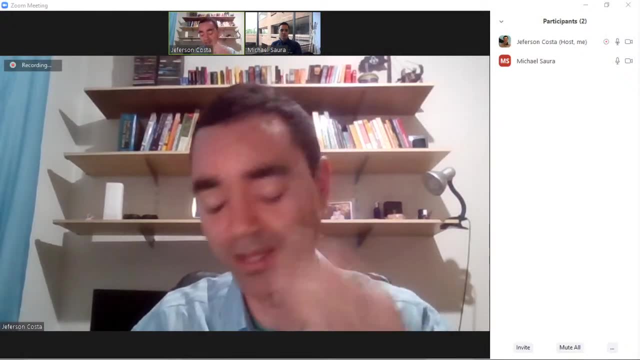 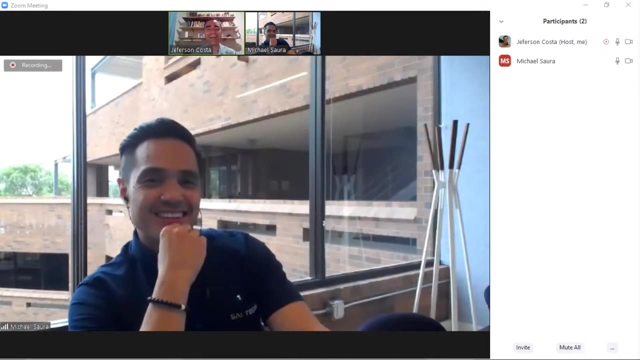 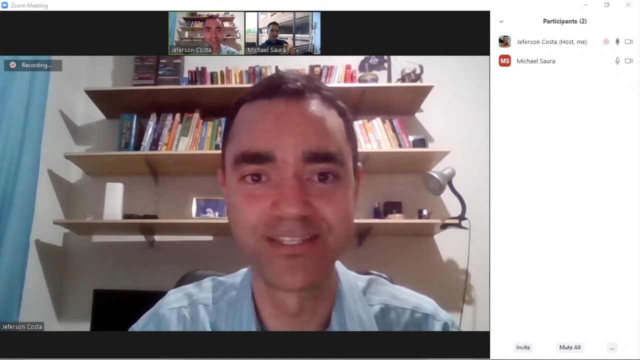 Your UI is a constant and more than 10 years of experience in safety processing- Ah, I remember what I would say. Sorry guys, live session. okay, There is no cuts. I can add your LinkedIn link in the description of this video, right? 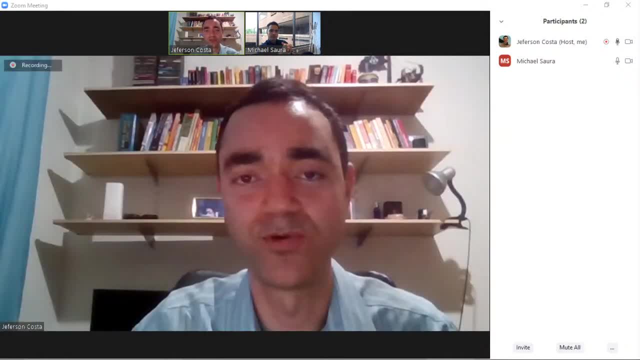 Yes, yes, no problem, So it will be easier. guys, if you want to know more, more information about course and references, you can see the Michael LinkedIn profile and talk to him, And he is very, very nice guy And, if you don't know, I met him in the internet. 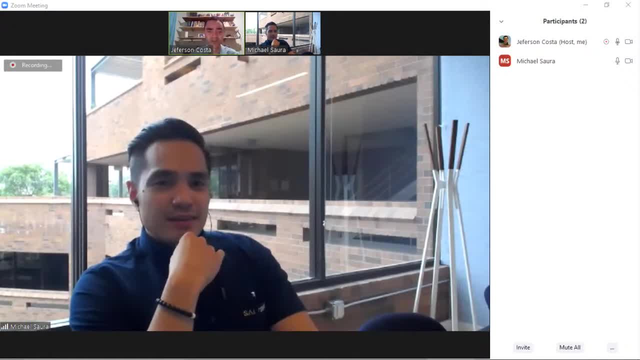 I think it was one year before or something like that. I did some posts related to HAZOP and you comment on that, So we started our relationship and now he's my guest And he will just talk about how it was. like, where were we when I started my business? 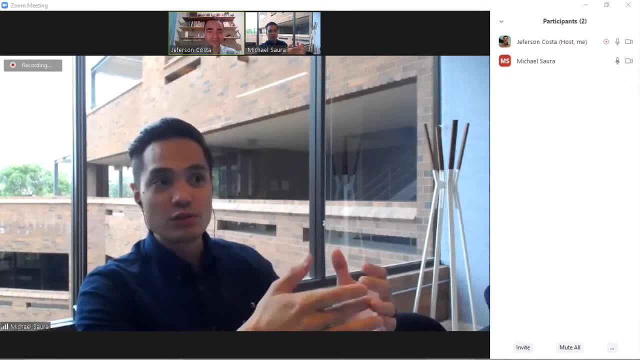 And he said: yeah, you know, we're hosting a very open, very open community of teachers to internet. all of us, and you know, in our office we do this campaign as well, So it's a lot to do. 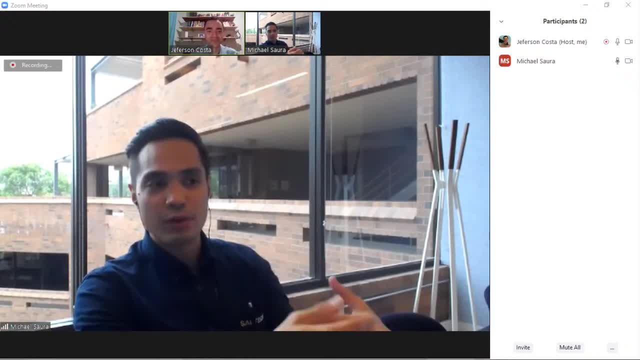 Yeah, Thank you, No problem. But yeah, we're coming- actually something that I understand. we're actually coming with a lot of resources as well from from our company. So just go to salt triggercom Right now there's. it's not there yet. 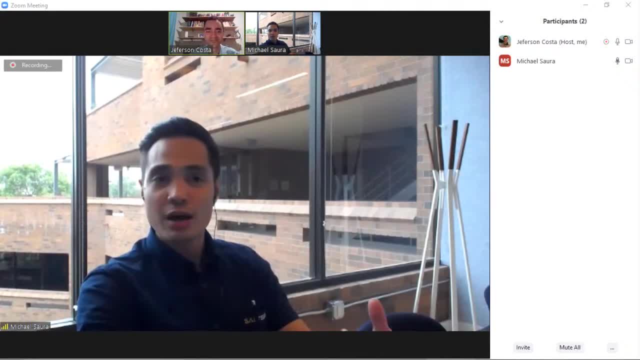 but we're developing that platform where people can get free up to date. but for now, feel free to reach out. happy to answer any questions. just you have my linkedin um. just reach out to my um for my linkedin, okay, michael, thanks a lot for accepting my. 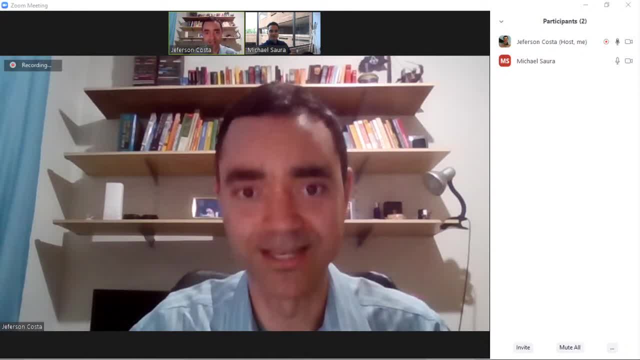 invitation you accept properly, properly accept my invitation to talk about process safety. it is a very, very nice subject and it is very, very, very big and we just get a introduction here to to fresh engineers and people get familiar with this subject. of course there are- there are much more to. 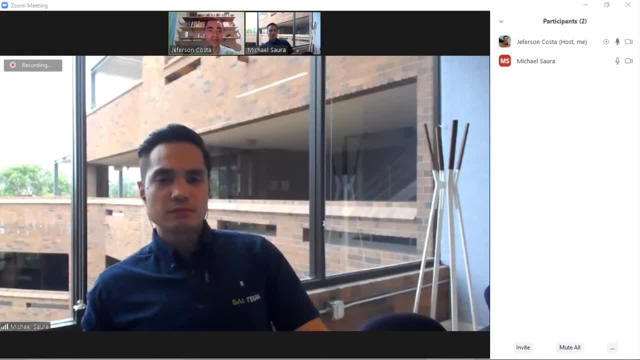 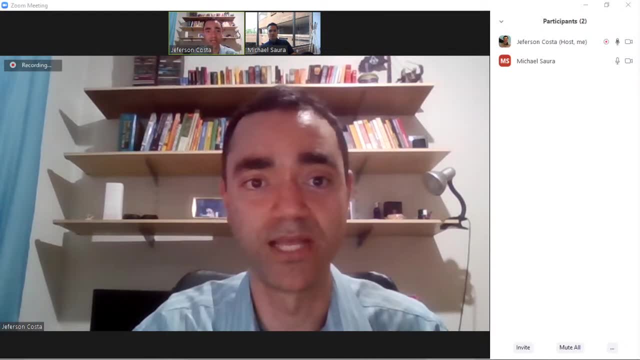 be said and please, if, if you can give a final message to people that are here with us. there are some other questions, but i will let for another time, because we passed from one hour here and i i want to let you free to to give any message that you want to. 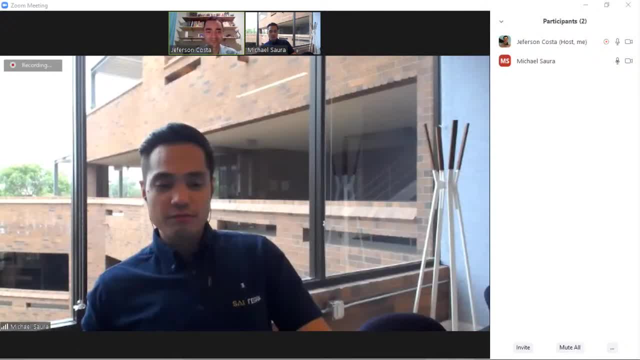 uh, so for- thank you, jeff, by the way. um, but for, you know, people who are wanting to get in the field, or people who are looking for jobs in process safety, i would suggest that you know you just it's, it's a, it's hard, it's hard right now. it's hard times, but, um, just keep on, you know, keep on. 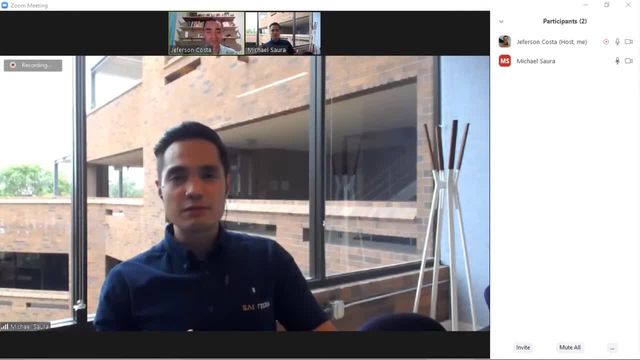 studying, keep on building yourself, especially with process safety. this is a more experiential and knowledge-based subject. i mean a lot of people are going to be able to do that, so it's a lot of you know, a lot of uh disciplines are, but in this field, because there it's so wide. 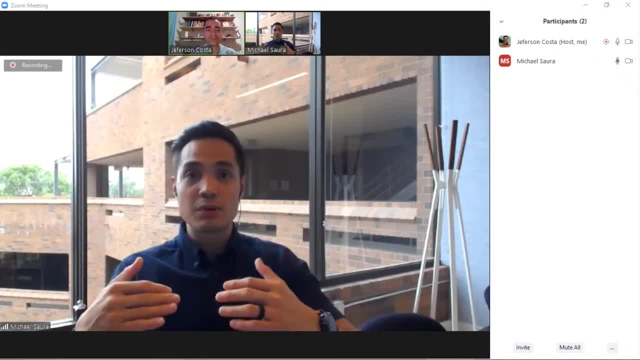 you would have to understand at least the basics of it, which is process safety, and then from there you can pick what specific element or topic you want to get into. but just you know, go read the resources um, try to get as much e-learning or courses out there and then reach out. like i said, 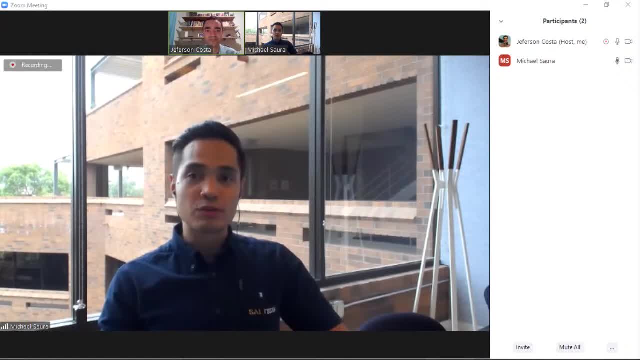 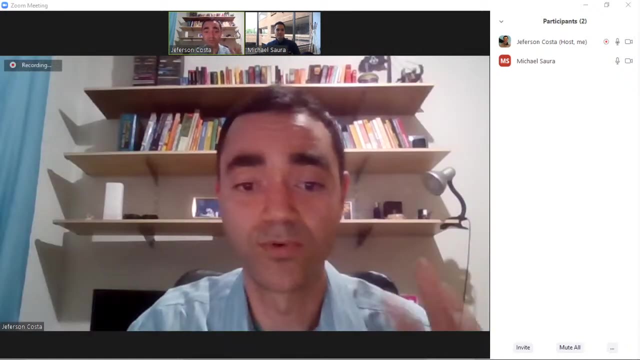 reach out to mentors, reach out to um other consultants, other uh people like jeff is an awesome resource. so, yes, just uh, keep, keep in tune, and i'm sure jeff and i will be happy to help you in regards to process safety. hey, michael, i almost forgot something that. 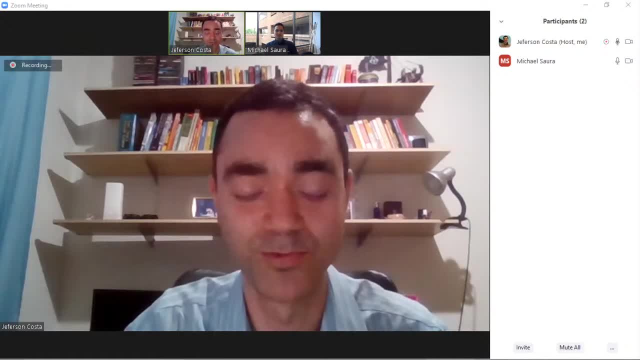 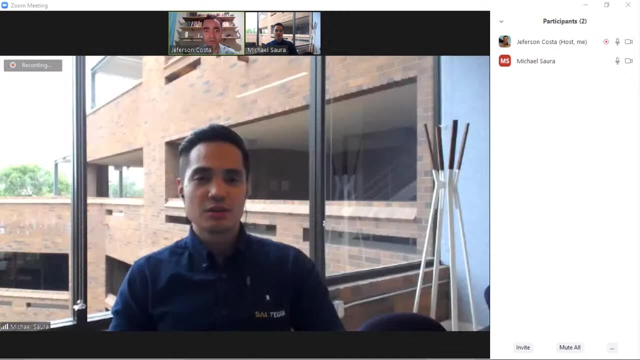 i promised in the beginning of this live session that it was: how did you get from philippines to the us and work abroad and please could you give us a little bit? i know that many years, a lot of of time. so us government that may may change it a lot of rules, but how did you? 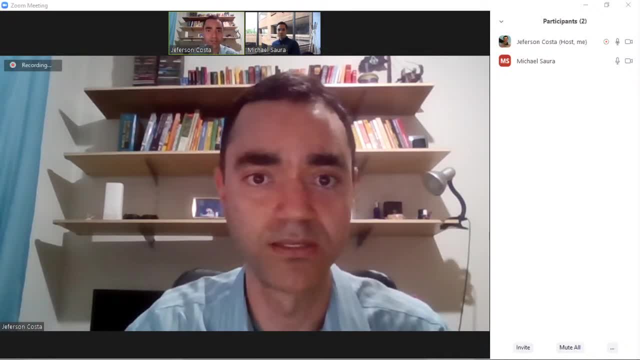 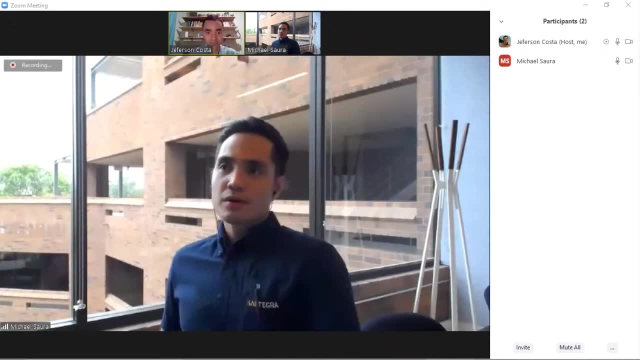 decided to, to to left philippines and work on us, and how you prepared yourself for that. so, um, there are. there are many ways to, you know, get to the us and start working here, but for for me, i was petitioned through family, so my family has migrated ahead of me, um, about five years before me, and then my 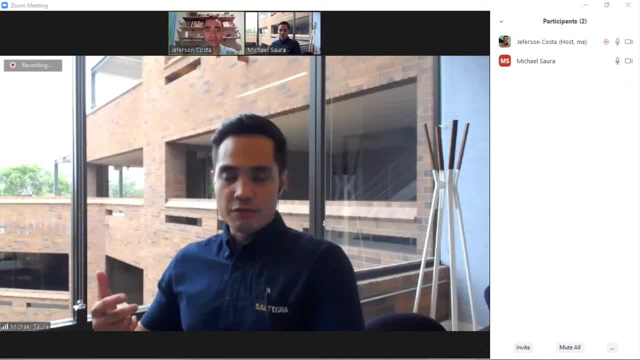 parents started working here, they got their visa as an h-1b visa. so right now you probably for people who are interested- you've probably heard of that visa. now it's basically a working visa that you can get from an employer, so an employer has to sponsor you. 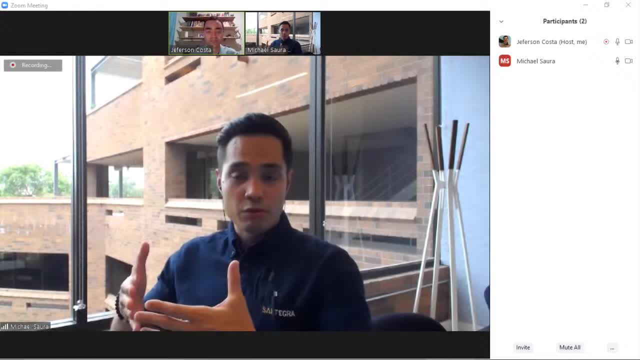 um, through uh, through, through them, through the company, as a specialized uh type of type of visa. so this h-1b is where you come over here, you apply and then- or actually you can- you can apply from abroad and see if they're sponsoring h-1b visas. so that's one way of doing it. 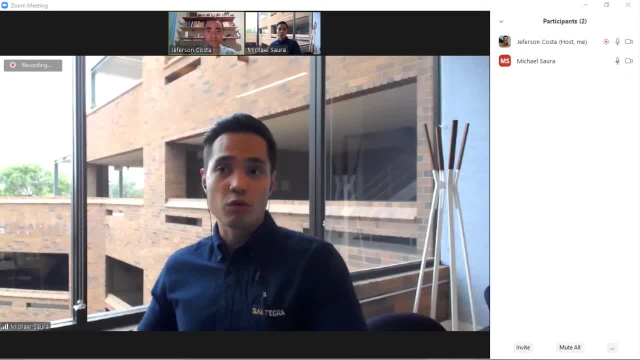 there's also l-1b visas, which are more specialized, um and again, and it has to be from the company and it's based on unique special uh skills. so it's because it's a special skills visa where, if you're only one of the few who can do that type of work or the subject matter that only a few of 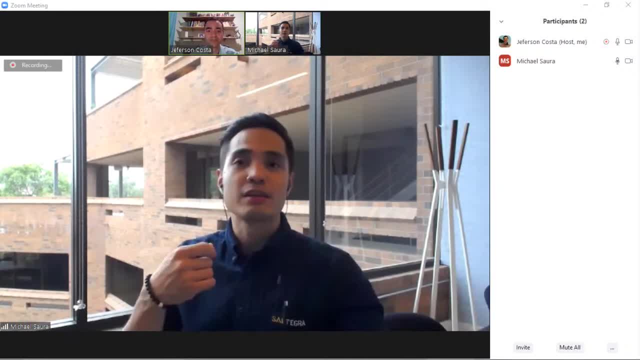 you know in your, in your industry and the company really needs that, then they can, you know, go in. so if you're a positive safety person or chemical engineer with very niche knowledge that only you know how to do or what to do, and then you can do that, and then you can do that, and then you can. 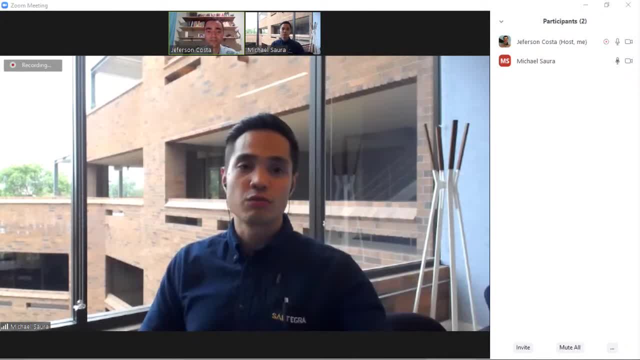 do and the company needs you, they can sponsor you for that. so again, it's back to the knowledge and experience um based uh way of getting here. so those are the two main things that i know. i won't. i'm not an expert on immigration so i couldn't speak of uh any other ways, but for me also you. 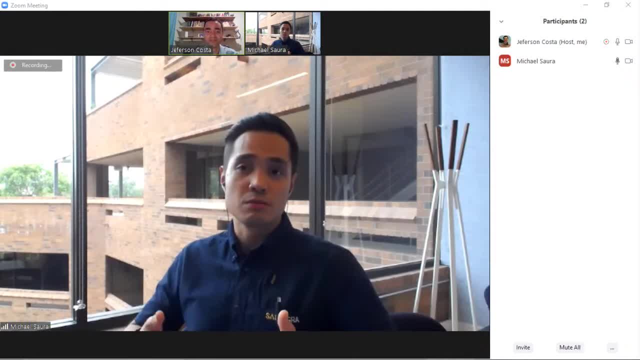 know i was like i said, my parents were here. they petitioned me through their visa, which was from an h-1b visa as well, but that has to happen before you are 21 years old. so if you're under 21 and you and then 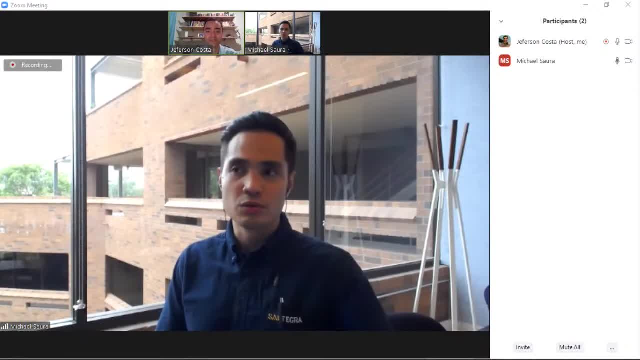 someone here. maybe your parents are working here, then they can petition you. a grandfather or some other relatives can, but they're they take longer. parents petitioning uh it um, their, their, their children are faster, but if it's a grandparent, an aunt, they can, but it takes longer. so there's a. 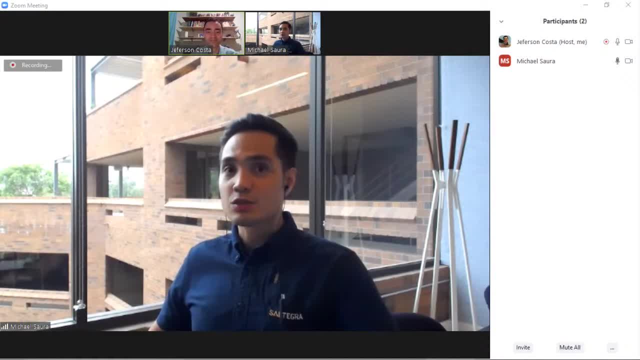 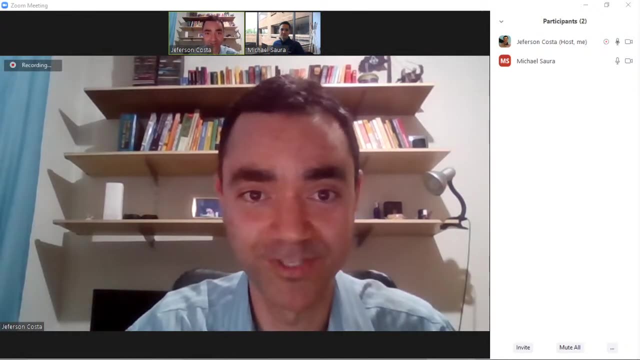 longer wait period there. so usually the fastest way, i would say if you don't have a relative, is the h-1b visa or the l-1b, but you have to reach out to employers and ask them if they're sponsoring those visas okay. so, guys, this is was the bonus of the live session. it is nothing related to. 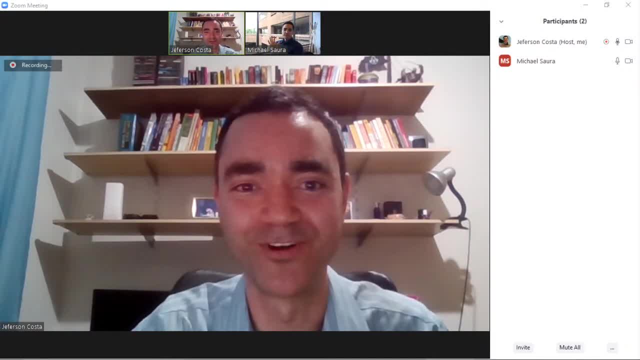 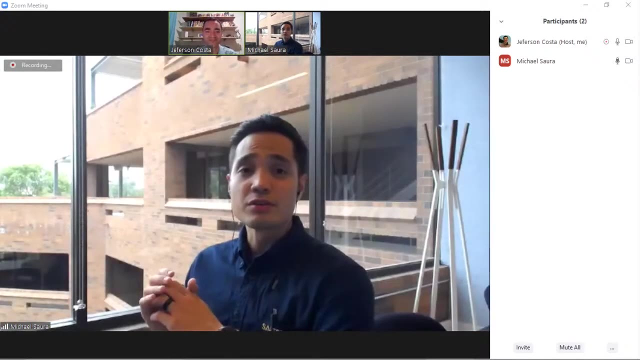 process safety. but thanks, thanks a lot, mike, for sharing that with us and my friend. have a great, great saturday and we meet you soon. another live session, or now, now in in zoom and something like that. okay, my pleasure, jeff. thank you as well for having me for the audience. thanks for your participation. 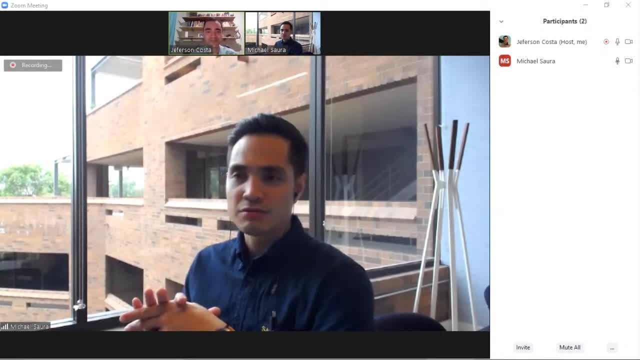 i'm happy that you know you guys are following jeff. just please support him. he's doing an awesome job here. you're making chemical engineering a popular thing again. so, jeff, i'd like to thank you again for what you do. this is, this is amazing. keep it up, and i'm happy to.